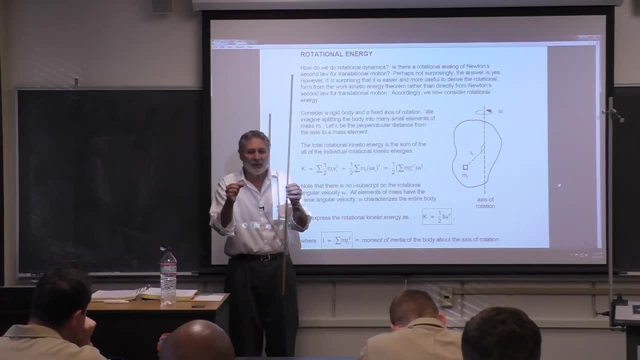 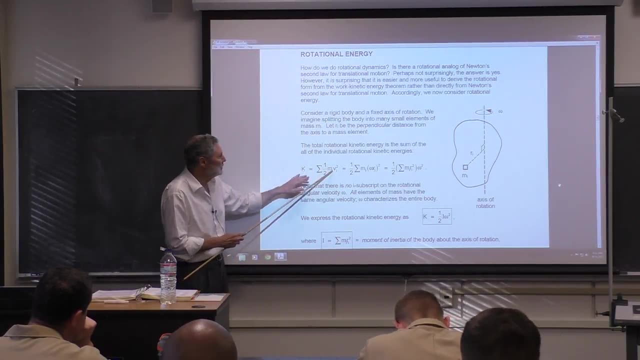 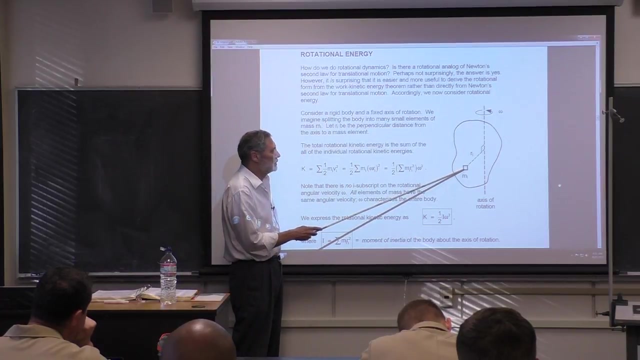 It's supposed to be out towards you like this. So that distance is important because the kinetic energy, the total kinetic energy, is going to be the sum of all these little kinetic energies due to all these particles. So the ith one here has, it's going to be one half the mass times, the square of the speed of this little particle here. right, The speed, remember what it is, It's omega times r. 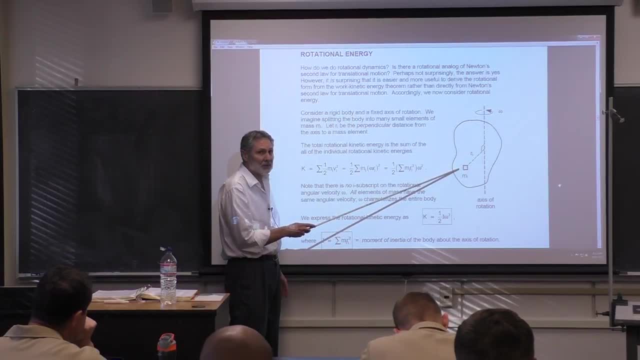 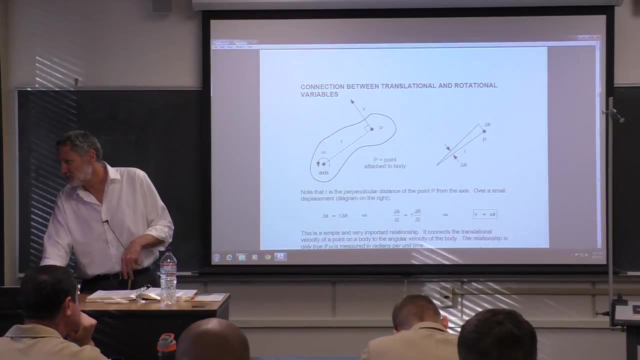 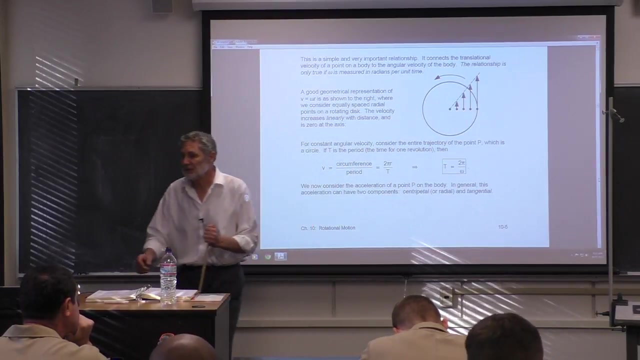 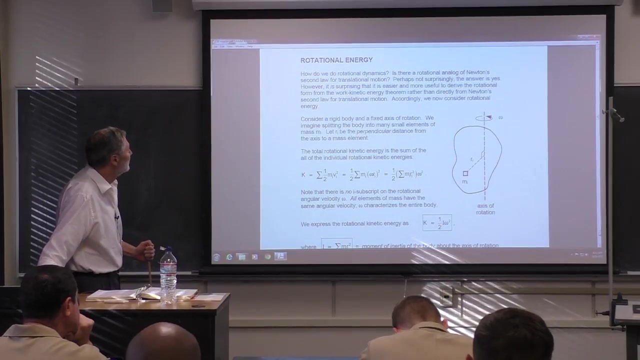 It's proportional to the distance. We talked about that yesterday, So remember this. Oops, right there, Right. So for a rotating, rigid rotating body, here the speed of a particle is proportional to the distance. So we substitute that expression- v is equal to omega r- into the- into here We square it. 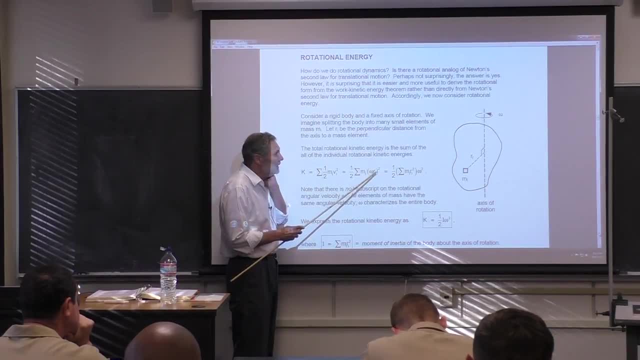 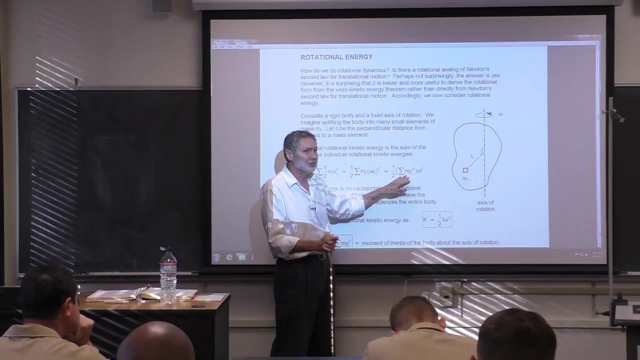 And now omega is a constant It. every point here has the same omega. It has the same rotational rate, right? This is a rigid body, So we don't have an ion there. It's characteristic of the entire body, So we can factor it out of the sum. 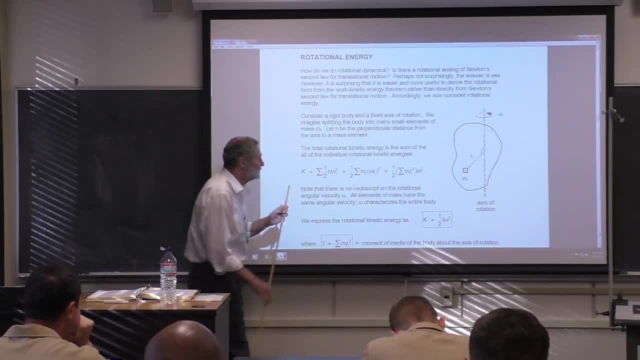 Now you normally think you want to factor it this way. Well, I'm factoring it this way for a reason. Look at the form of this One half, something involving the inertia times: omega squared. So that's how we write it. 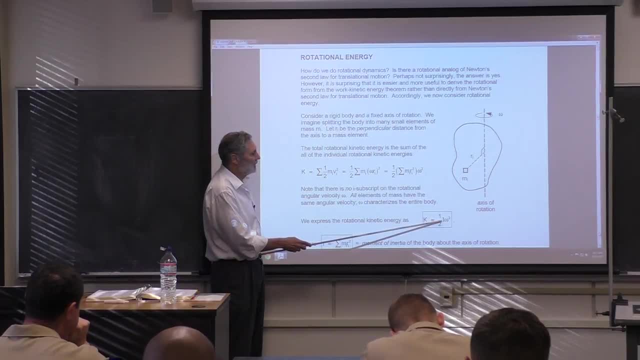 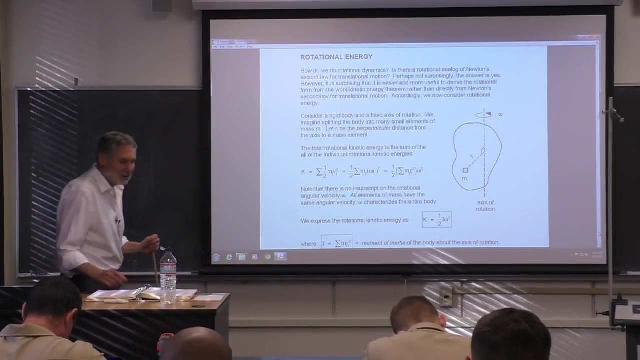 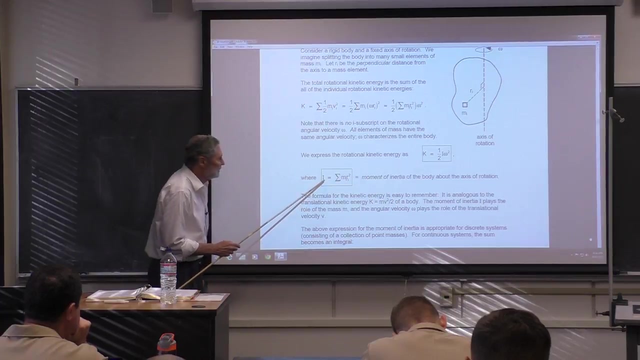 One half. We called all of this capital I, and it's called the moment of inertia of the body, About this axis, About that particular axis, and what the moment of inertia is is. you can see it from here. you have to sum up. 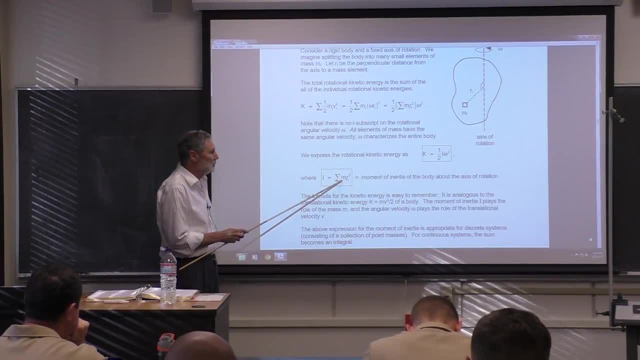 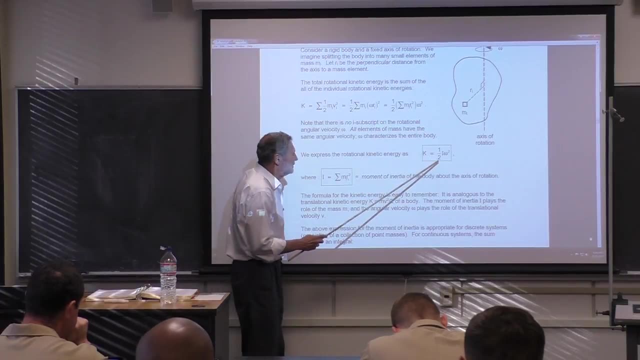 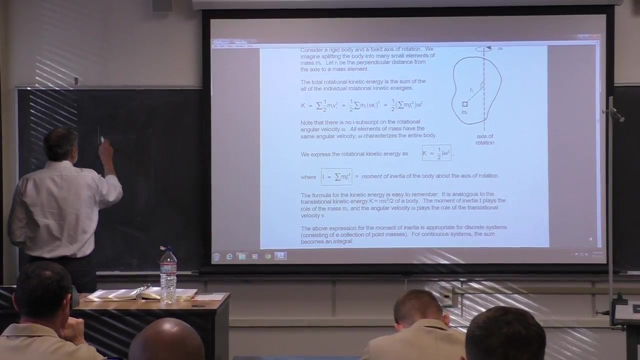 all the mass elements and multiply by the. each mass element, you multiply by the square of its distance to the axis of rotation. So does this look familiar? This should look familiar. It looks a lot like the linear result, right? So it's easy to remember. 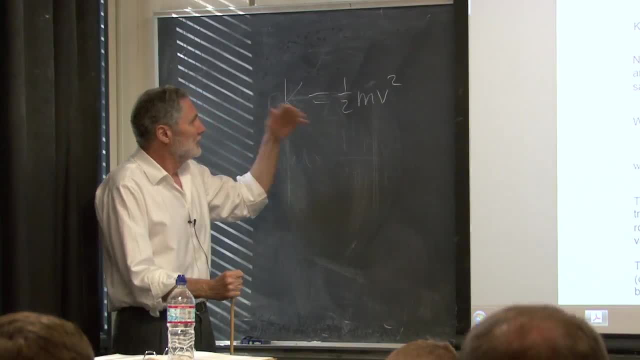 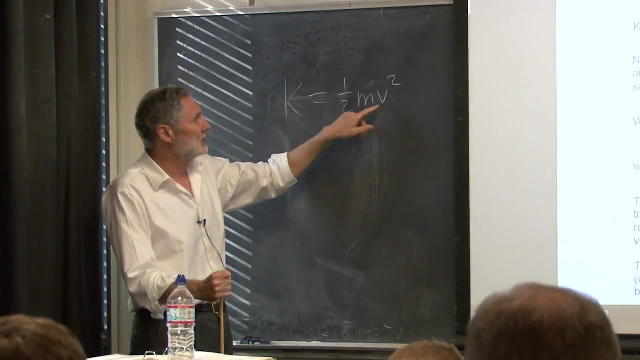 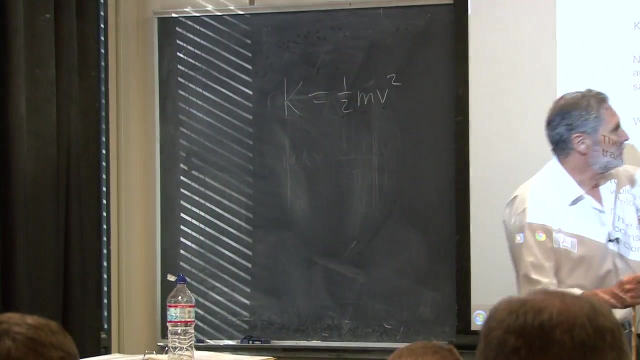 So for straight line, for translational motion, the instantaneous kinetic energy of a particle is one-half the mass times the square of the velocity. It's the same thing for rotation of a rigid body, except we have to use the analog of the mass. 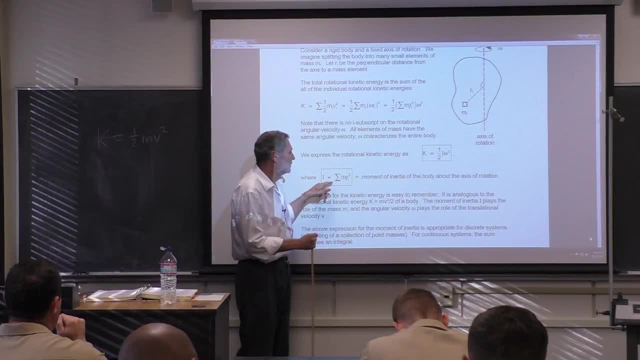 which is the moment of inertia here, And we have to use the analog of the velocity, which is obviously going to be the angular omega, the angular velocity. So it's easy to remember this Now. you'll notice here that this doesn't just involve the mass. 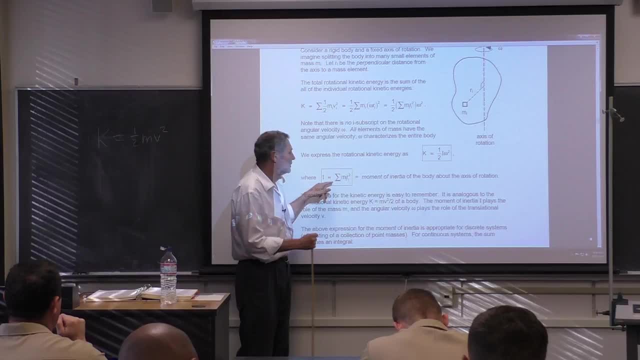 It involves the distance the mass is to the axis, And that's got to be true because this is contributing us some kinetic energy To the total value. If I doubled R for the same omega, what's going to happen to its contribution to the energy? 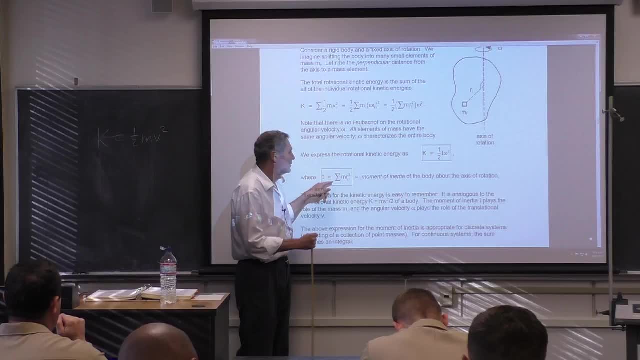 It's moving twice as fast. It's going to contribute four times as much energy as it does here if you double it. So distances are important here. Now any questions so far? So that's the basic formula. Now, often 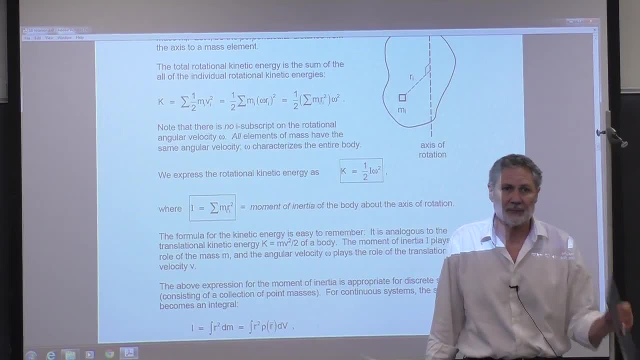 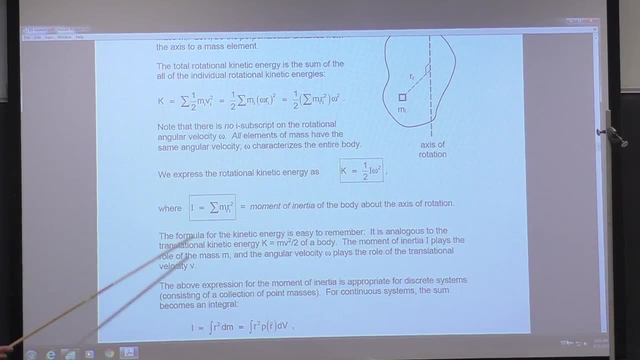 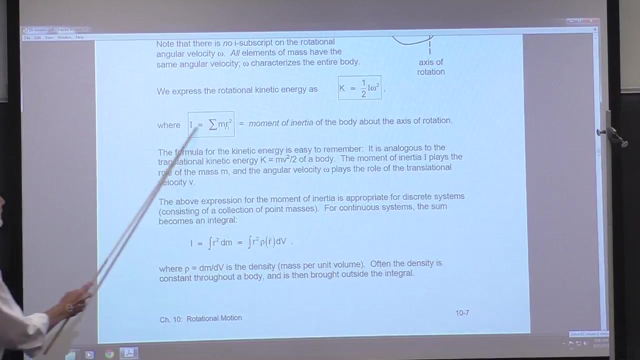 we're dealing with continuous bodies, OK, like this. And in that case to calculate- and we're going to do several calculations today- to calculate the moment of inertia, the sum here becomes an integral. So an integral over all these little mass elements. 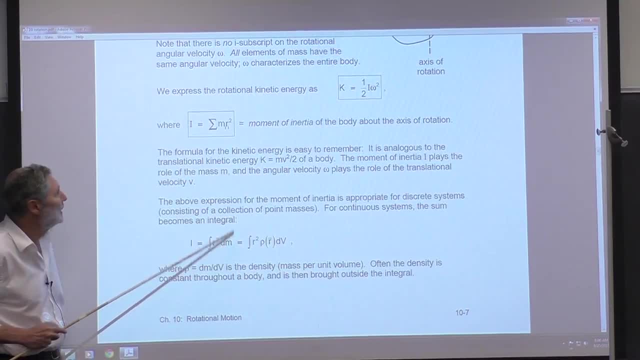 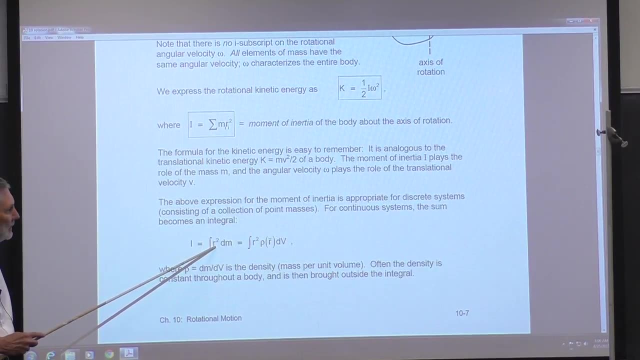 So the mi becomes dm, a little bit of mass, and you need to multiply by the square of the distance of that little mass from the axis of rotation And then integrate over all of them. OK, So this may look strange to you. 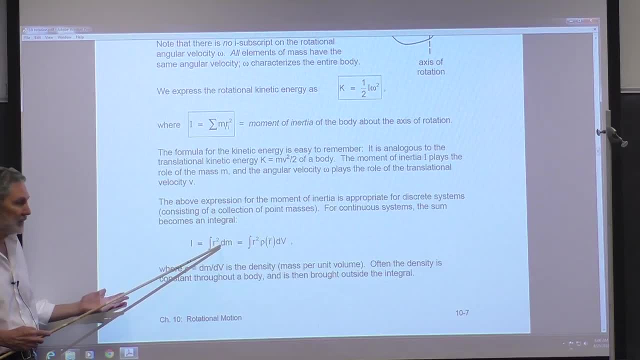 but it's perfectly legitimate and it's very physical. You know, it's just a little bit of mass times the square of its distance. To convert it to an integral that we can do. we want to get rid of this mass. We want to put it in terms of coordinates, right? 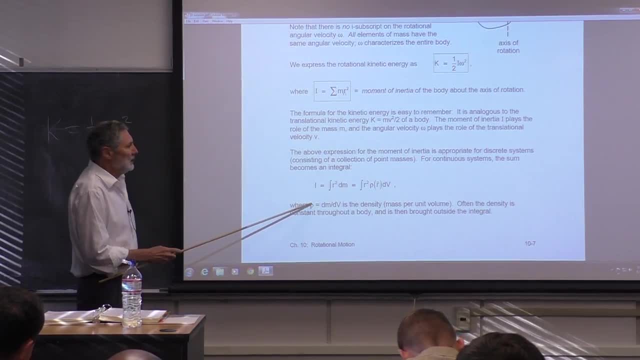 A little bit of volume. So we do that with the density. The density is the mass per unit volume. So we'll go through some examples. We'll go through several examples. We'll go through several examples. We'll go through several examples of this. 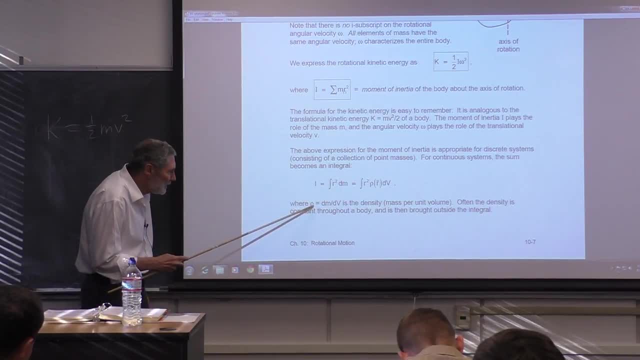 But just formally here, in the general case the density at the location of this little mass. here there's going to be some density And by definition it's the mass divided by a little bit of volume. So I can substitute for dm here. 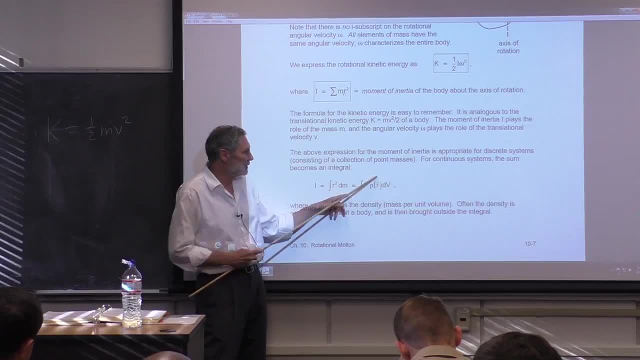 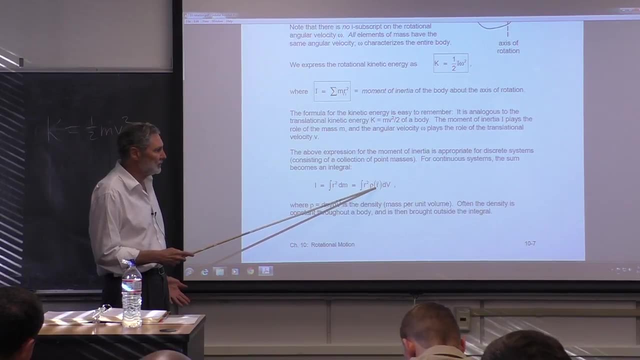 I can substitute rho dv. So that's what I've done here. So now we've got something. Once you know how rho, what rho is as a function of r, now you've got an integral. This is a little bit of volume. 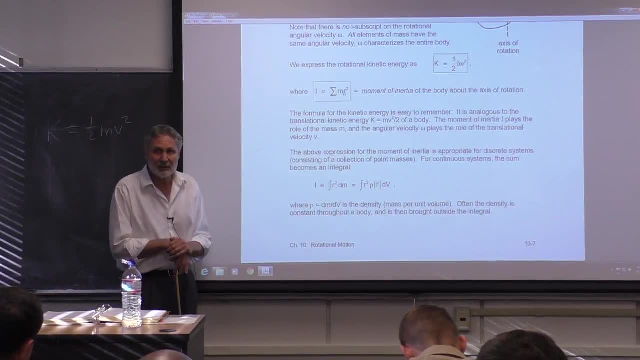 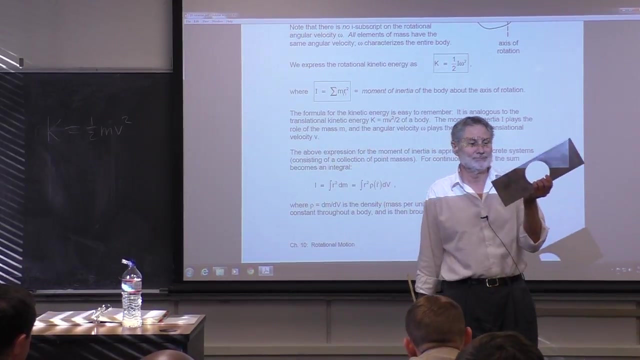 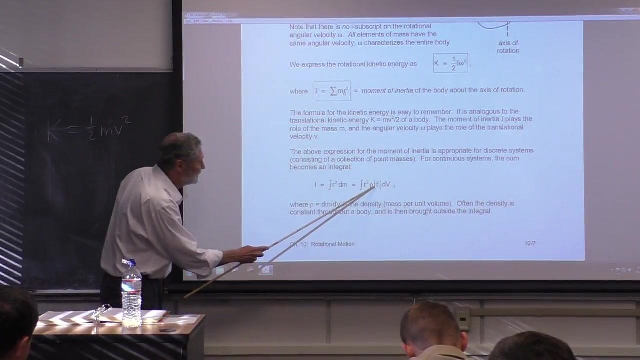 In Cartesian coordinates it's dx, dy, dz. Now it's reduced to integral calculus. Now in this class, I think all of our densities are going to be constant, Like here, for example, right Density of aluminum. So once we realize that it's a constant, 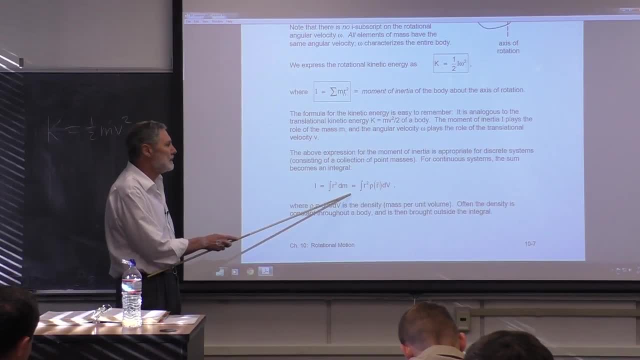 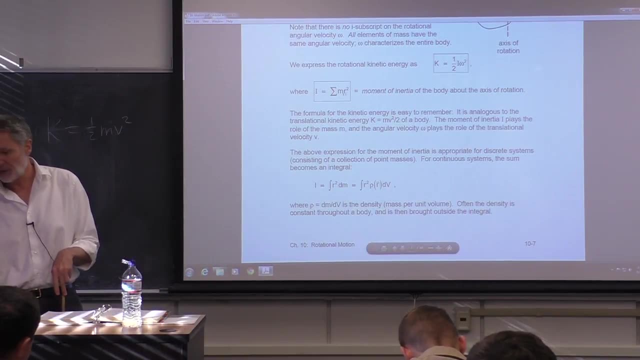 it can come outside the integral, And then we have to integrate r squared over a little bit of volume elements. So that's what we'll be doing. We're going to do that very soon. Before I go to the next page, any questions so far? 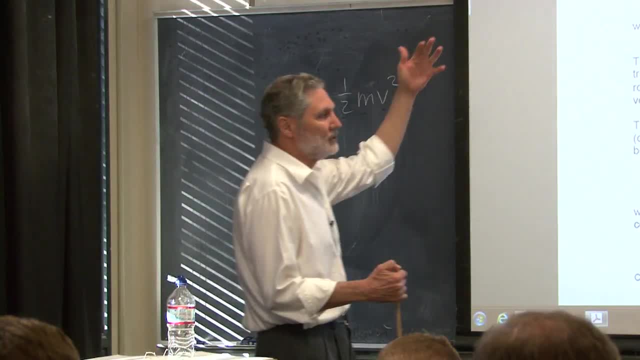 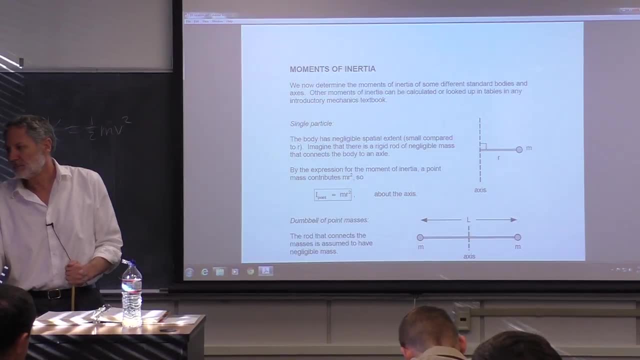 This is pretty straightforward. It's a big advantage. using energy, We're going to be able to get at the dynamics using energy. Okay, So what about this? We're going to spend some time now on this quantity called the moment of inertia. 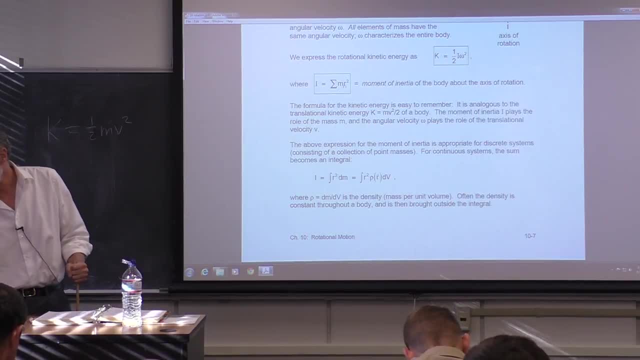 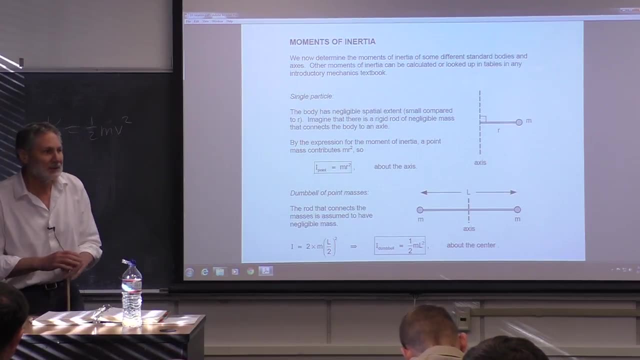 Okay, We're going to calculate it. in special cases And all introductory mechanics books you can look up moments of inertia of different objects and different axes of rotation. So let's go through. Let's start with the simplest possible case and that's a single point mass. 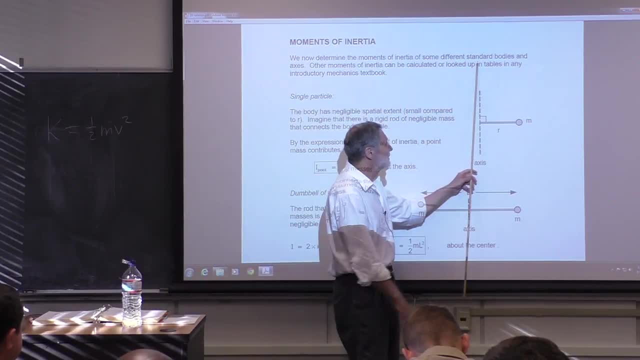 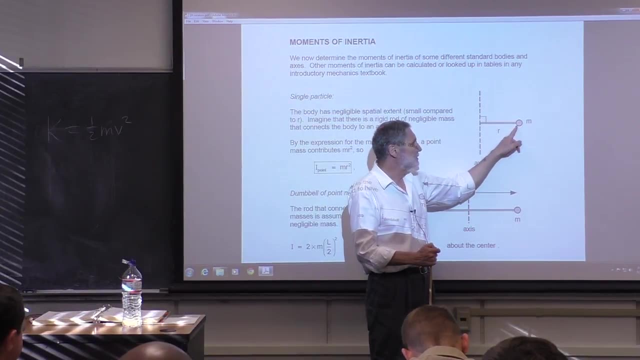 So this is a mass here. It's some distance off, It's not as far from an axis of rotation And it's small compared to this distance. It's really a point. Okay, From a practical perspective when we say it's a point. 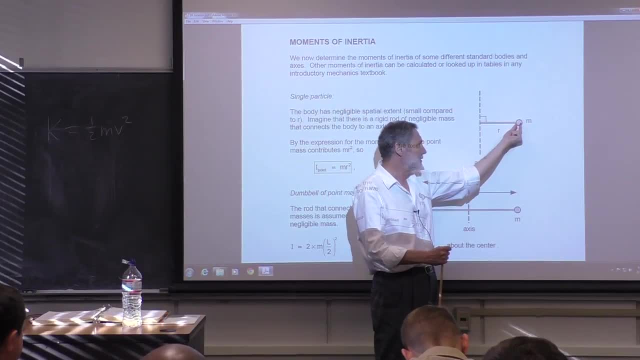 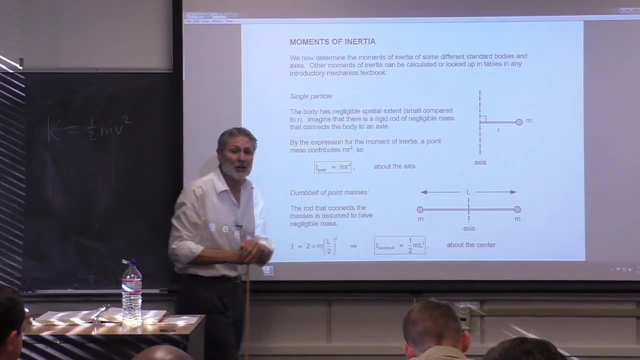 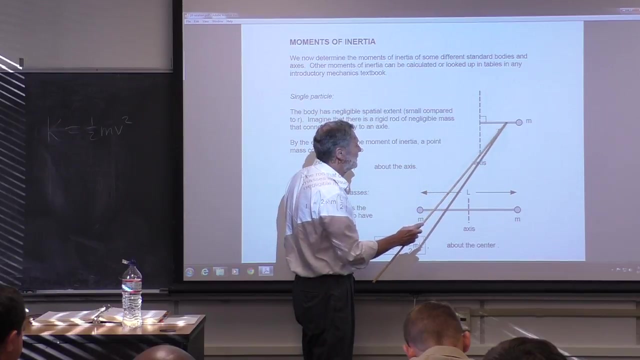 what we mean is it's diameter. here it's the characteristic length of this body. the radius or the diameter is small compared to that distance, So we can approximate it as a point. So to help see this, you may want to imagine a massless rod, a rigid rod of negligible mass. 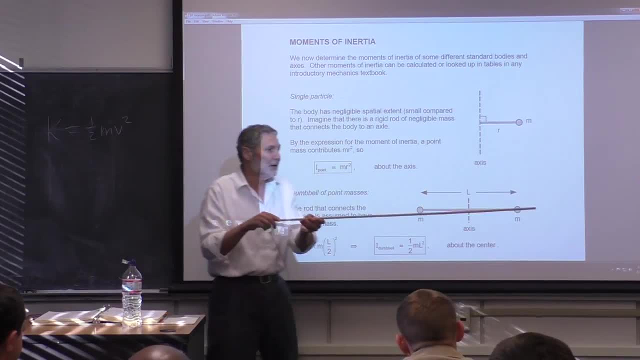 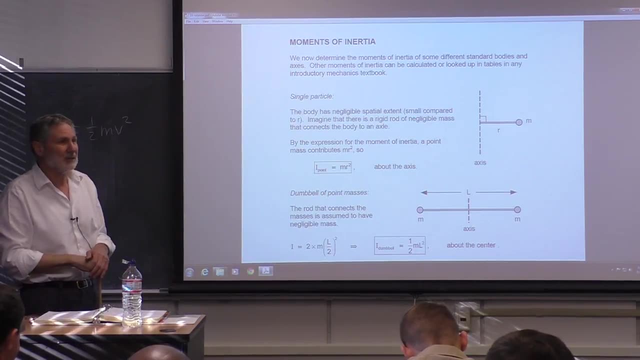 connecting the axis to the mass here and that this is going around like that. Okay, It's got a moment of inertia. What is it? It follows immediately from the definition: Each particle contributes its mass times the square of the distance. So we're done. 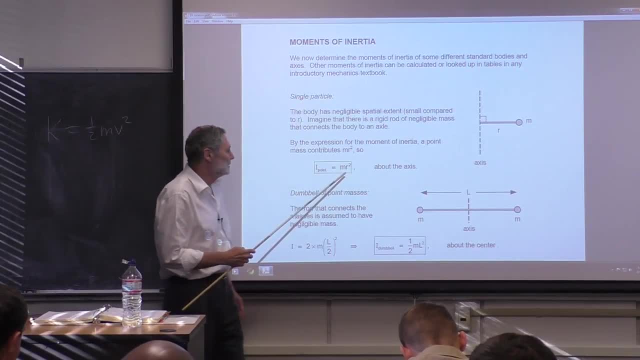 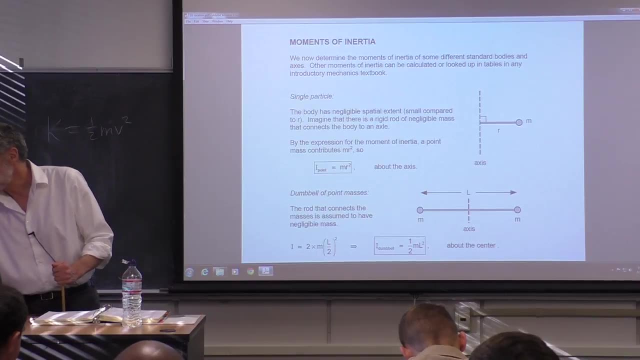 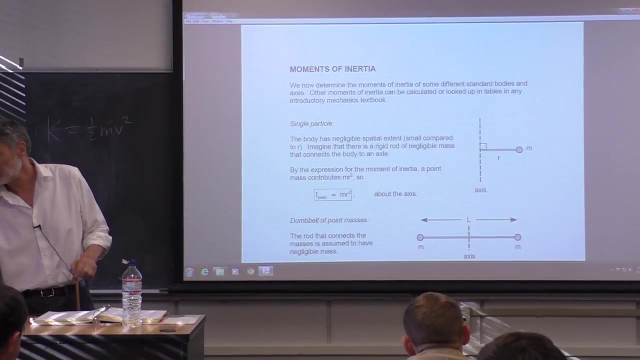 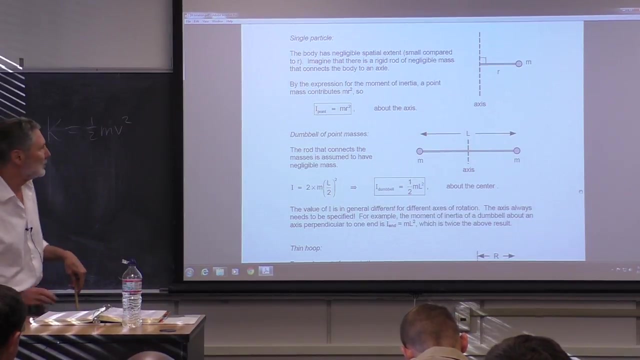 The moment of inertia of a point about some axis. a point mass is the value of that mass times the square of the distance. It comes right from our, immediately from here, Okay, Oops. So next up is two identical point masses. 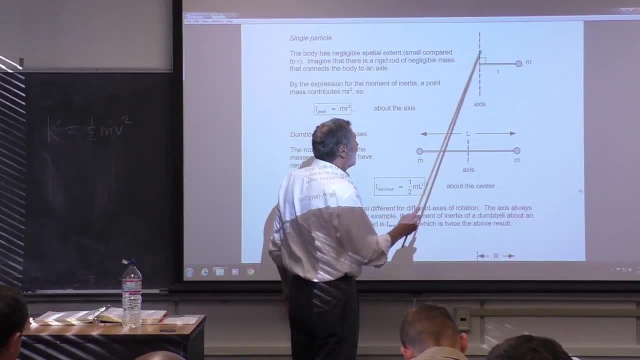 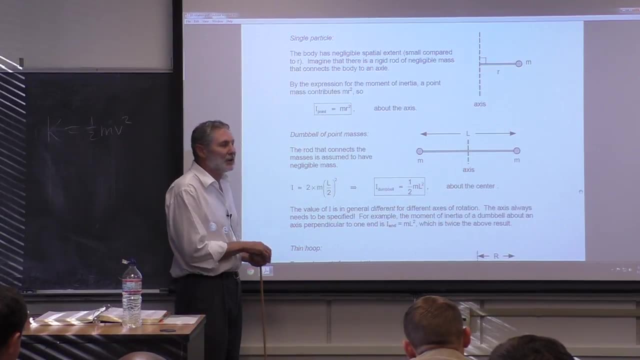 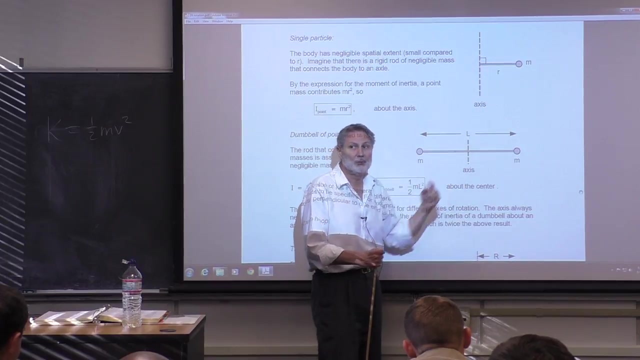 Okay, You can see, I just copied and pasted this and then edited it. All right, So now we're going to imagine two identical point masses separated by some distance that we'll call L, and we're going to choose the axis to be at the midpoint here. 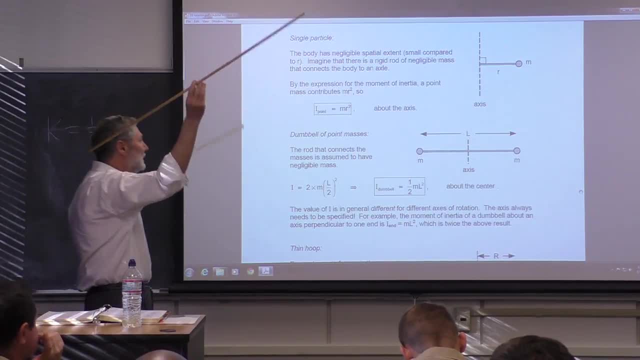 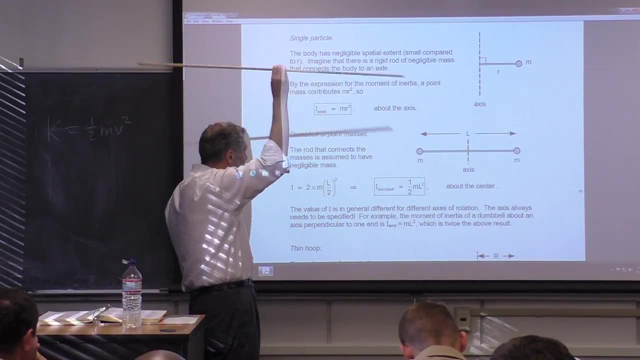 So this is a dumbbell. So you can imagine, And again we can imagine, that we have this massless, rigid rod connecting the two. So this thing could be spinning like that, right with these point masses on the end. So now, what's the moment of inertia? 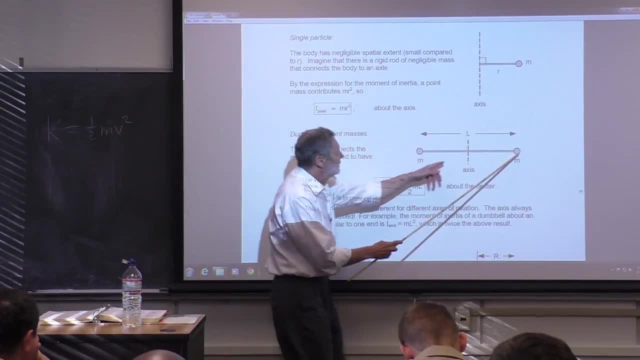 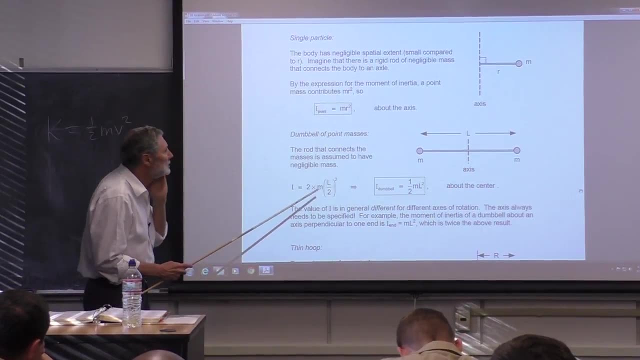 Well, we've got to add- this is going to contribute this: The mass times the square of the distance. This is going to contribute the same. So we just get twice. However you want to be, you always want to be careful here. 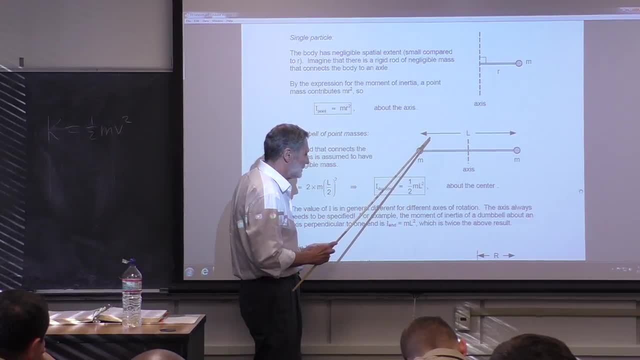 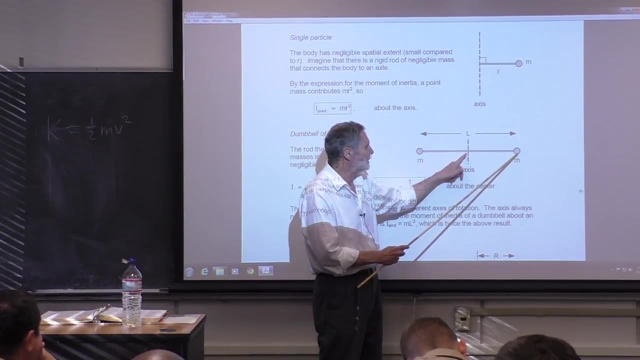 In terms of the param dimension that's usually used here, the distance between here This distance is not L, It's L over 2.. So when I do the sum here, I'm going to, when I look at one mass. 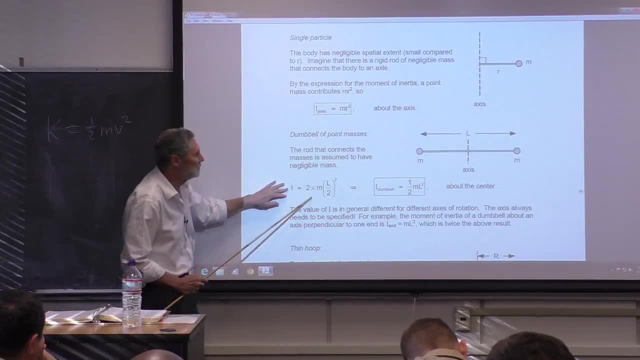 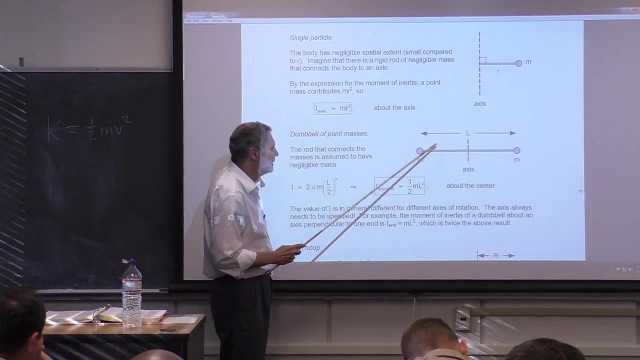 I'm going to get the mass times L over 2 squared, And then I'm going to double that, Okay, And then I'm going to double it because I have the identical one over there. So in the end, for in terms of this length, L here and the individual masses, this is what we get. 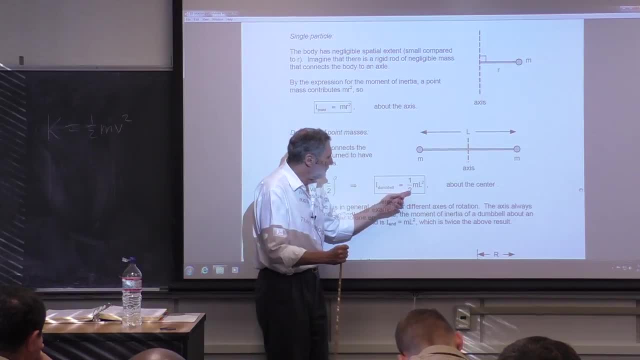 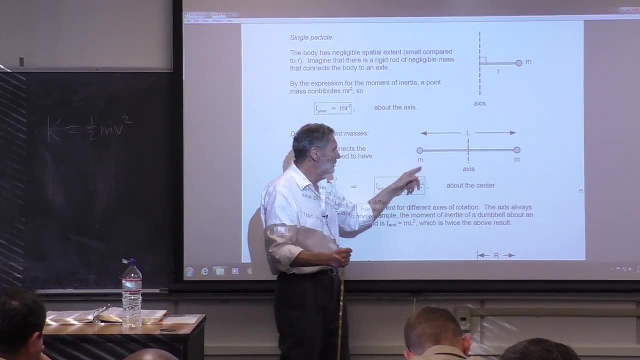 You always have to be careful with these expressions, you know, If you just looked at this, you might think this is L, That's not wrong. You might think that's the total mass. Nope, The total mass is 2M. 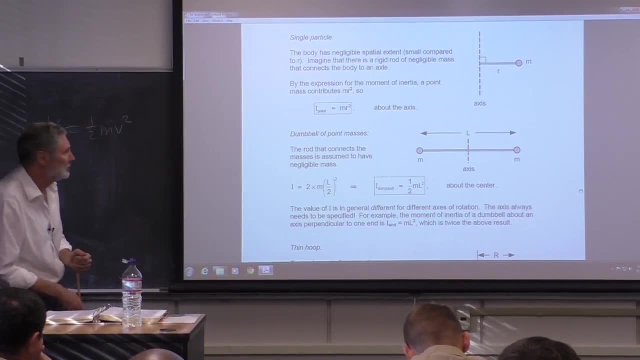 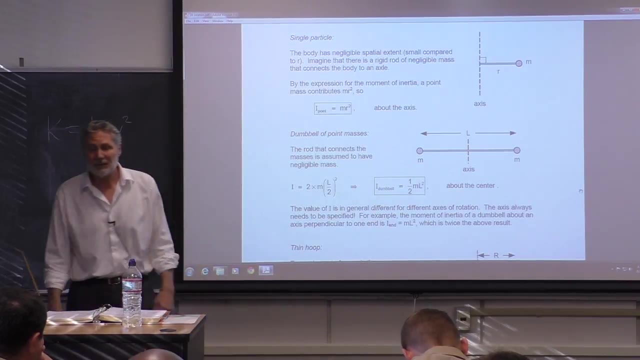 You could express it in terms of the total mass. you know You could make this a capital M You'd have to have. then it would be one-fourth. So you always have to be careful here of what the lengths and the masses are. 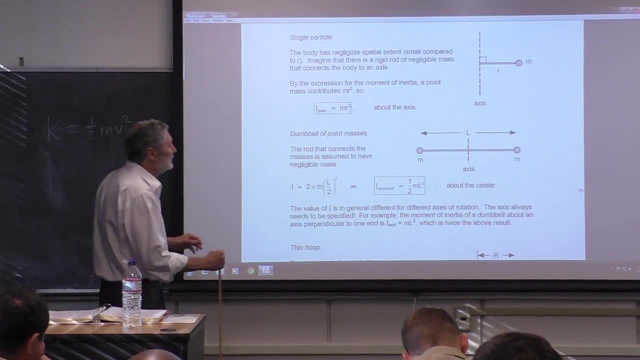 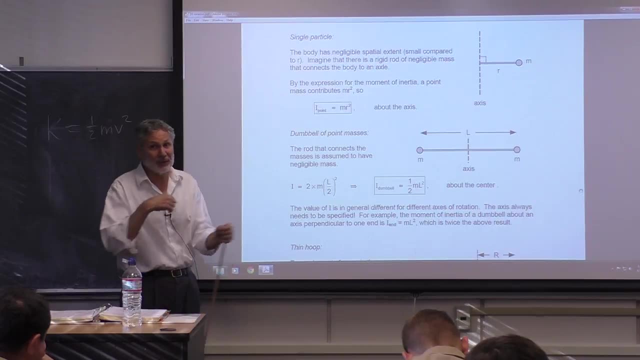 Now, whenever we specify a moment of inertia of a body, it doesn't just depend upon the body, It depends upon the axis, because all the distances have to be measured from the axis of rotation. obviously, Right. So you need to specify the axis. 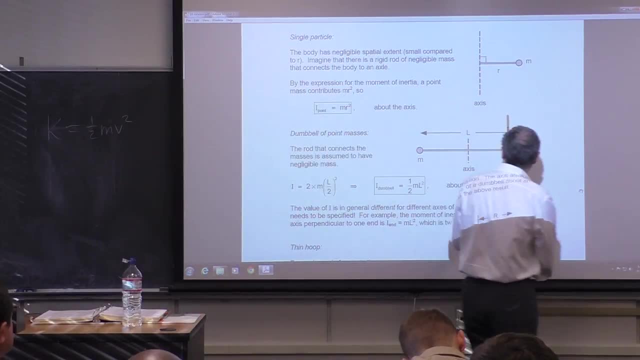 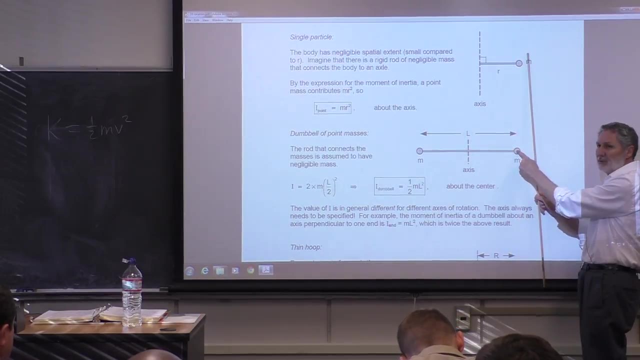 And here's a good example. What's the moment of inertia of the dumbbell about this, about an axis here? Okay, what does this contribute? Nothing, exactly. It's got no rotational inertia, which means you look at it and it spins. 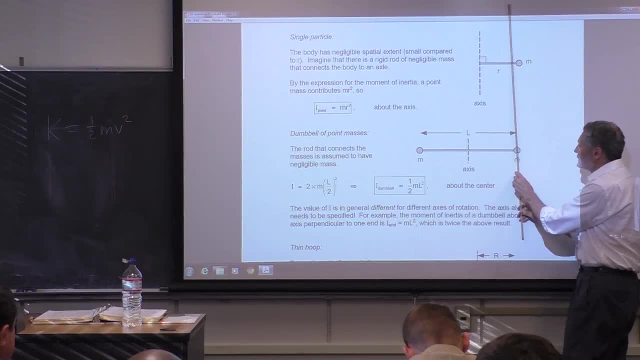 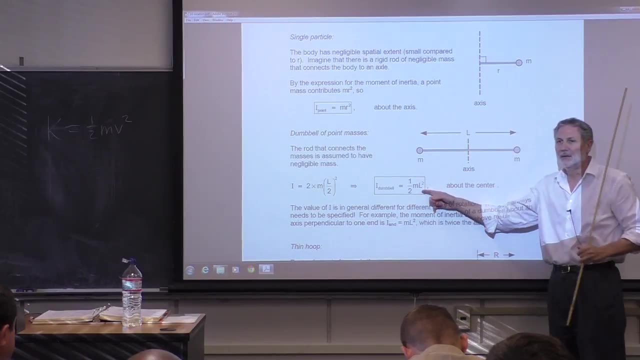 You don't have to do anything, Right? It has no moment of inertia, It doesn't contribute, So it's going to be well ML squared. Is that what we got here? No, we have one-half ML squared, So they're different. 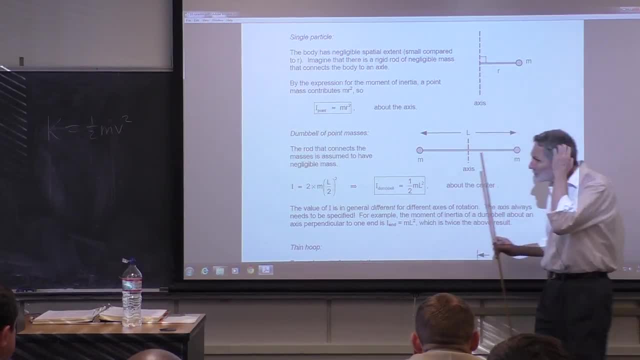 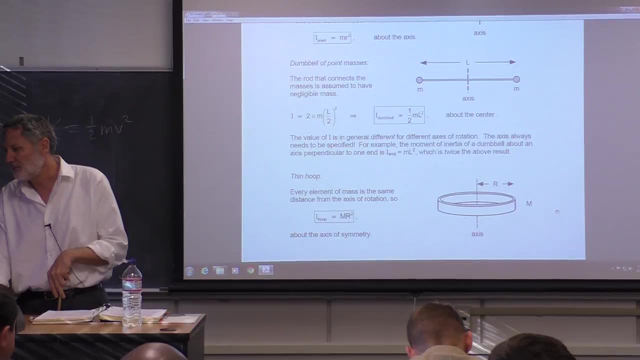 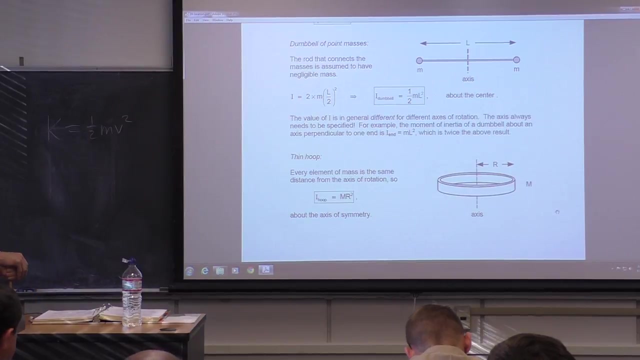 So in general, it's going to be different Move along here, So you always want to be aware of that. Okay, next up- and we're getting successively more complicated- here is the hoop, And we're going to take the axis of rotation to be about the center of the hoop. 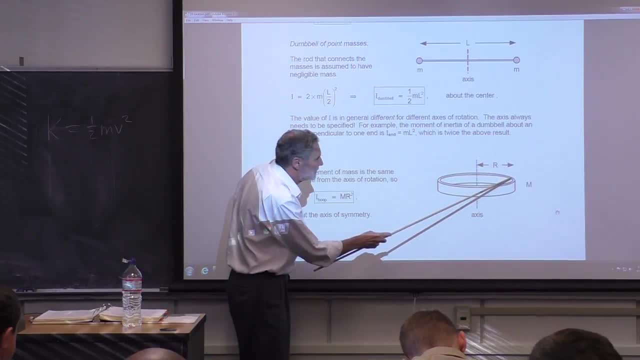 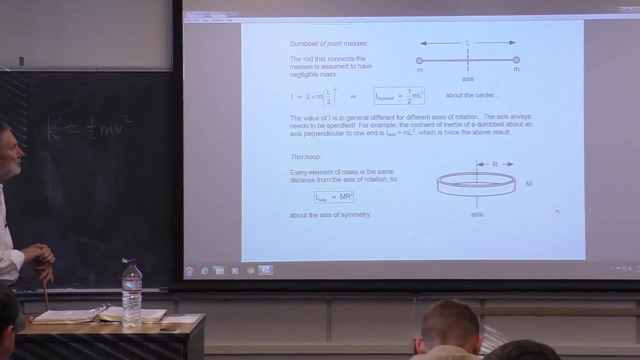 And this is a thin hoop, which means it's thickness here It's small compared to its radius. So for this continuous body we're going to switch to capital M here. This is commonly done. That's the total mass of the hoop. 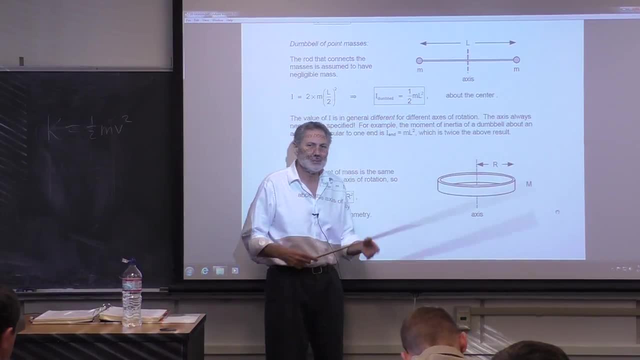 So what's the moment of inertia of a hoop? It's actually easy. You can just write it down immediately. Why can you write it down immediately? Each mass element is the same distance from the axis, So it's just a moment of inertia. 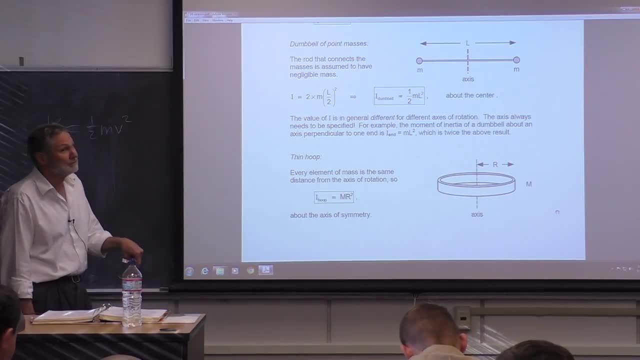 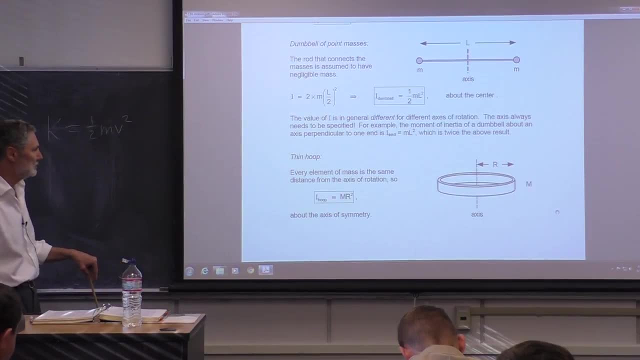 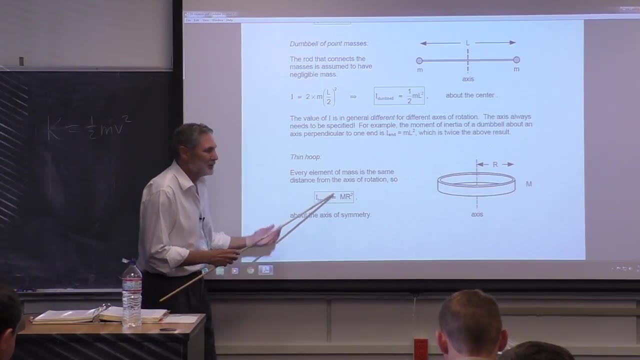 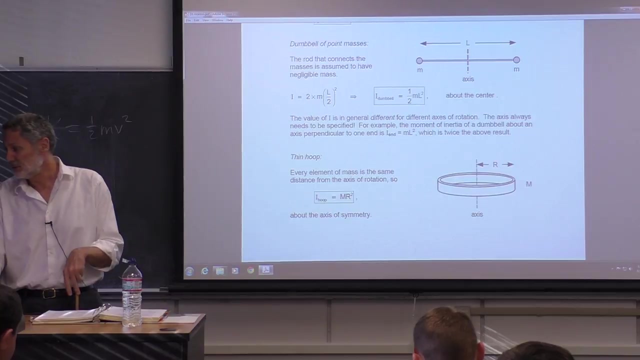 And I get the capital M, the mass of the hoop. So these you know, you don't have to look this up, You can just re-derive this, These simple things like this. they follow immediately from the definition of the moment of inertia. 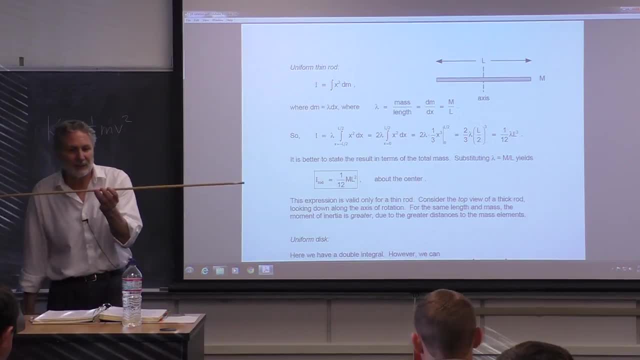 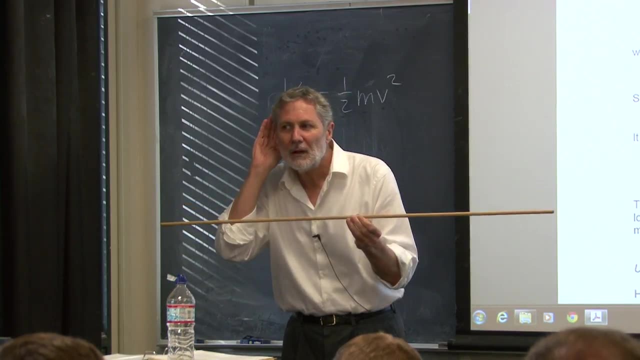 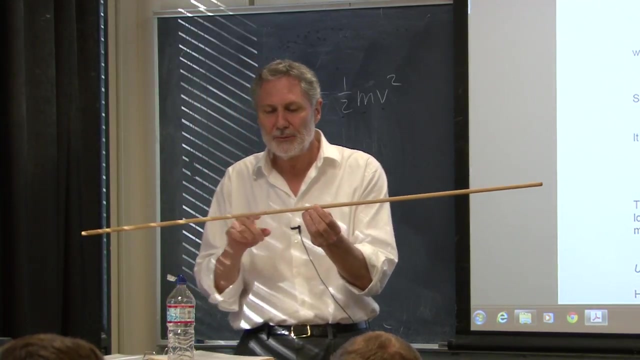 okay, now the rod. so now we have a rod here. this has mass. it's a uniform rod. what does uniform mean? I'm sorry, yes right, uniform means that the density, the mass per unit volume, is the same here. okay, and like I said, I'm pretty sure. 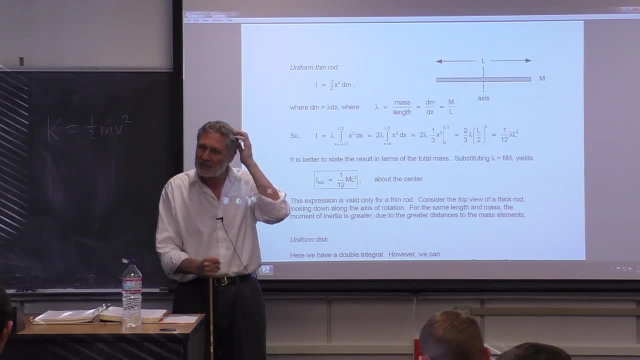 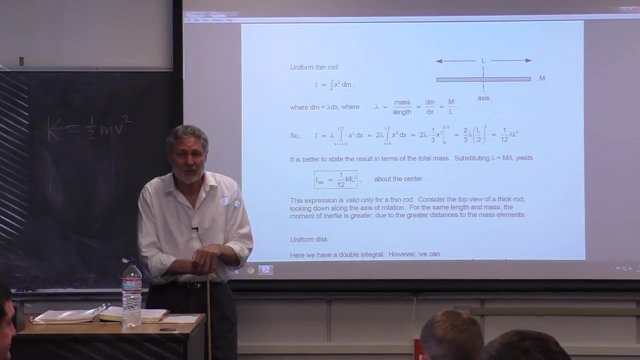 that's all we're going to be considering in this class. okay, now some of you may have done non-uniform density problems in calculus. you may you know because, like I've told you before, these center of mass calculations and these moment of an, they're commonly done in integral calculus courses. so I was talking to a. 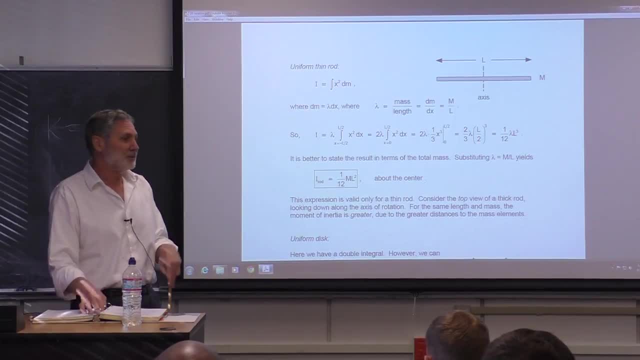 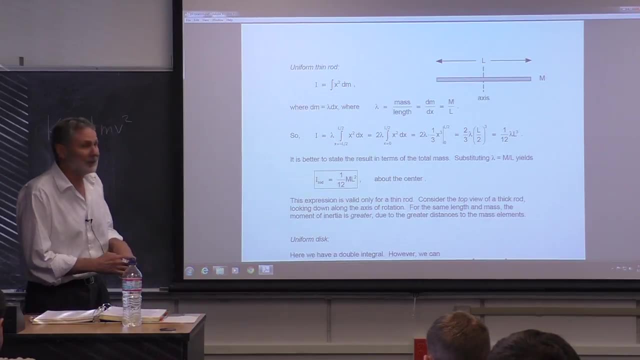 mathematics professor yesterday and he was looking at all the demos we do and I said some of these demos relate to calculus. you know when you need to integrate to find the moment of inertia. so I told him he needs to talk to me about you. come by the demo room, demo lab. 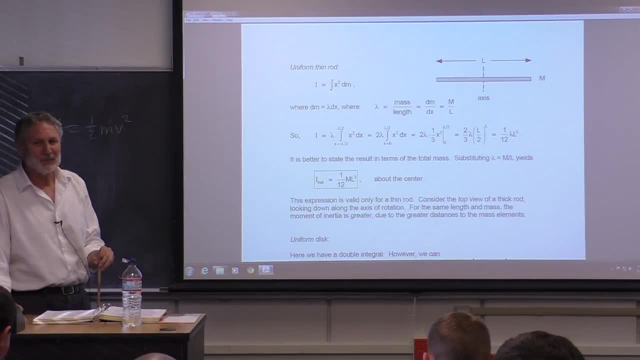 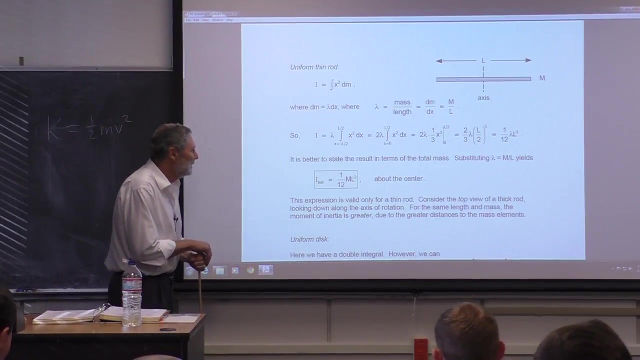 yeah, I think demos are a good thing. you know they help, but you know they do take time and effort and that's a lot of professors just aren't interested in that. okay, so what do we have here? we've got this rod. we're going to choose the. 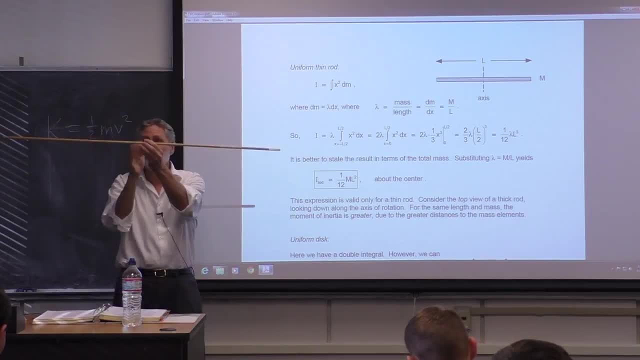 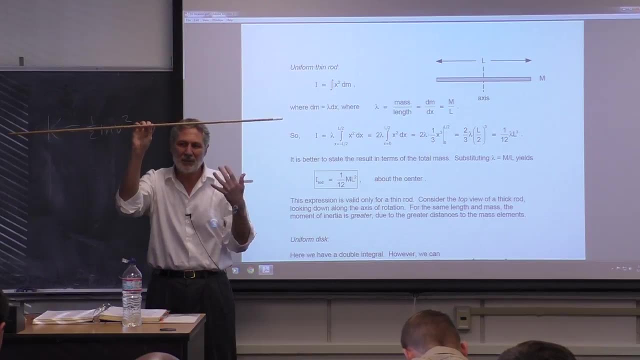 axis, the natural, you know, common choice is this the center here. so it's got some moment of inertia. and oh, by the way, what that means is, if you know, you know where we're headed with this. if I try to rotate this thing, it presents an inner I. 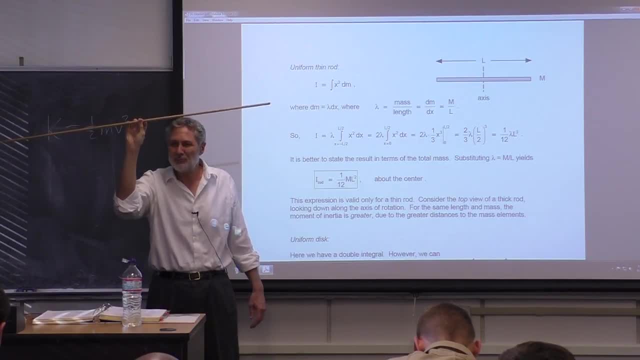 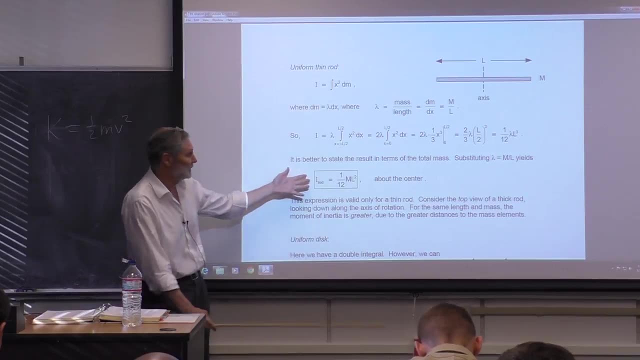 can feel it's got inertia. okay, because when I push on this thing, when I push on it here, it's resisting what I'm trying to do to it. it's got inertia, and that's what this, that's what this is the quantification of that, okay. so here we. 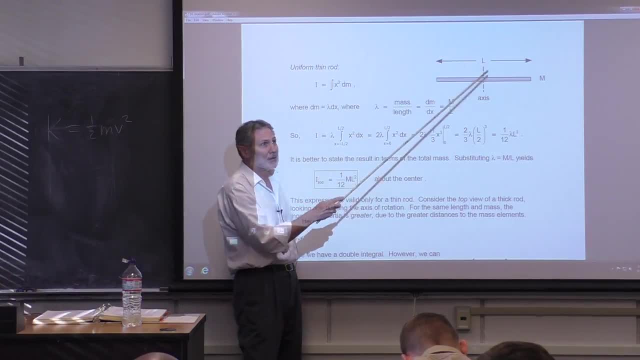 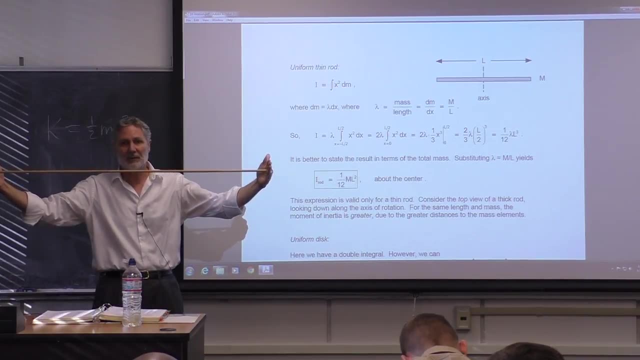 go. this is a one. oh, it's a thin rod too. we'll talk about a thick rod in a moment. this is thin. this distance is small compared to this distance. that's what we mean by sin. so here it is. it's a one-dimensional here. it isn't from a 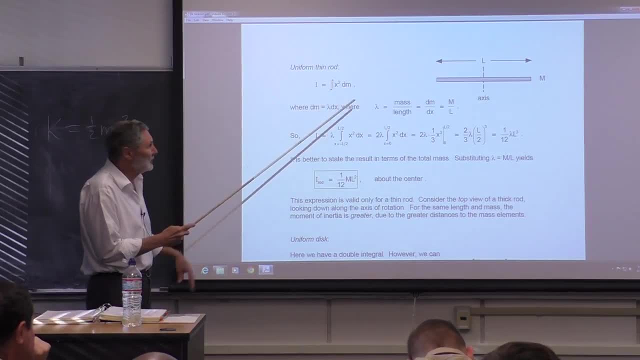 physicist point of view with the DM. we got to get rid of the DM because we got to do an integral right. we use the linear mass, the mass per unit length, here. that's the appropriate density to use here, because it's a one-dimensional problem. that's often. 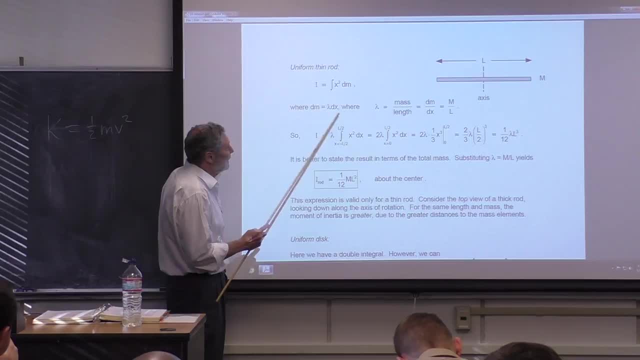 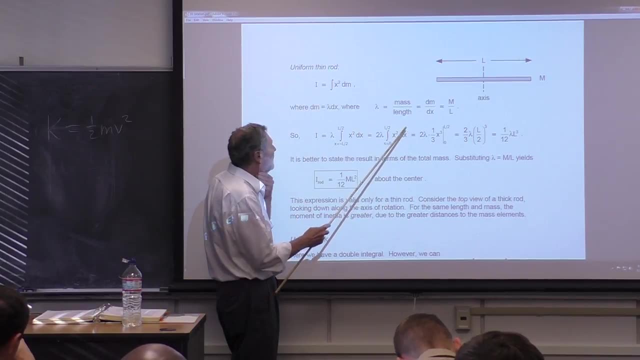 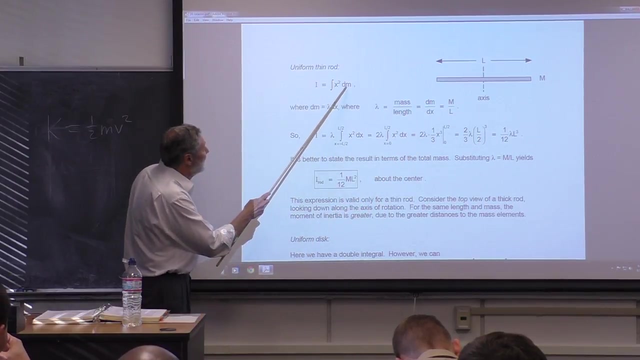 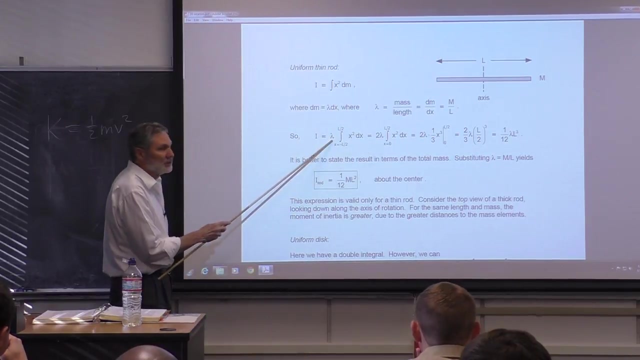 called lambda, so it's DM- DX. lambda is the total mass divided by the total length, because it's uniform and it'll also be given by this and it's a total mass divided by the total length. so I replace DM here with lambda DX and lambdas constant, so it comes outside. we'll just. 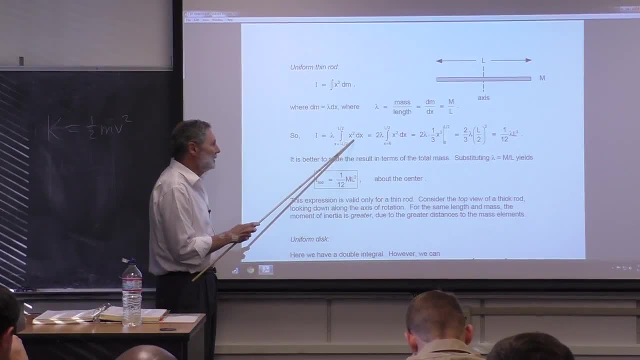 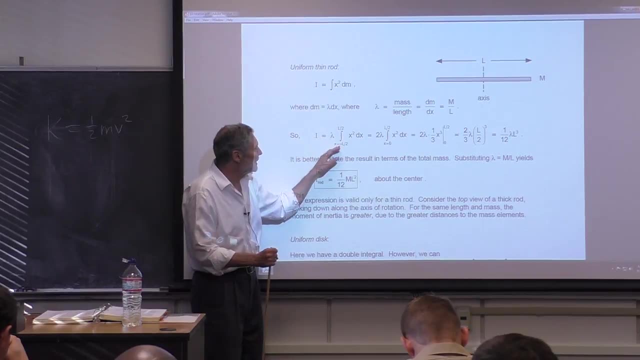 leave it there for now. and now everybody can do the integral of X squared right. it's 1, 3rd X cubed and then you need to evaluate between the limits. now it's common here to make life a little easier and less likely to make. 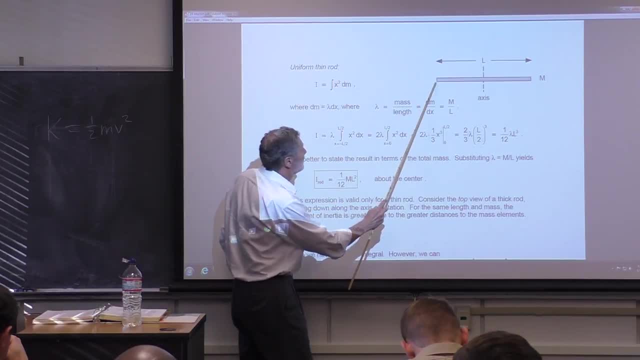 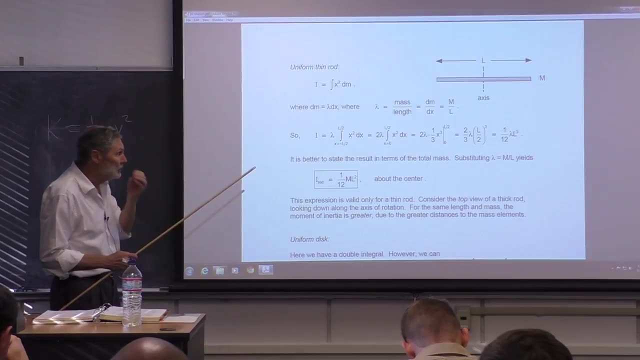 a mistake. we know that when we do this integral from here to here, whatever I get here, I've got to get here by symmetry. so the it's good here. you're less likely to make a mistake and it makes a lot of sense because it's a. 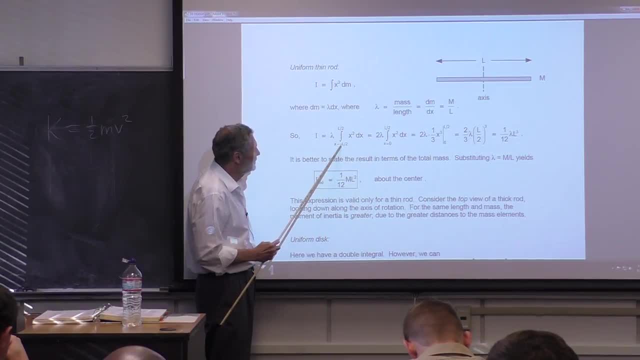 little bit more enjoyable, I think to. instead of doing this integral, I'm going to double the integral from 0 to L over 2. so whatever contribution this is to the moment of inertia, this has to contribute the same. so that's what's. that's the. 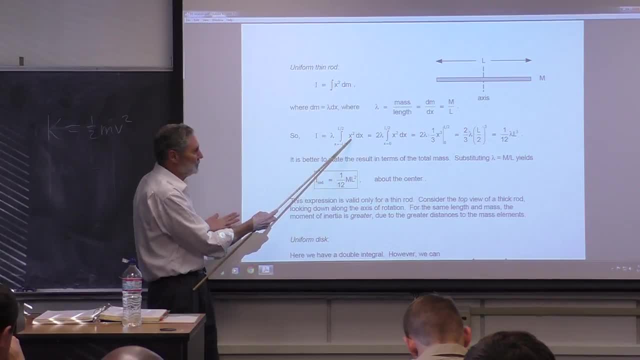 physical statement here you can also see it mathematically. this is a symmetric. the integrand here is symmetric. in X it's the same for a minus X values as a plus value. you know we're finding the area under a parabola and it's going to be symmetric. so we'll double the integral from X equals 0 to. 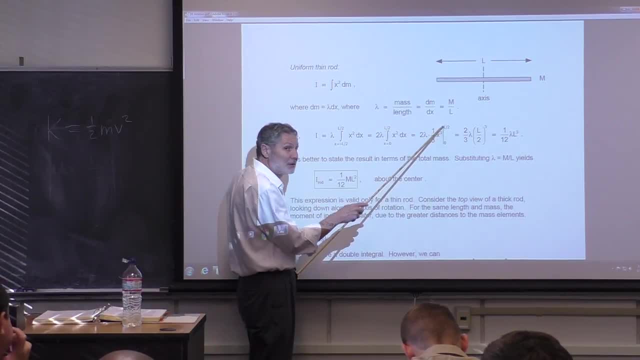 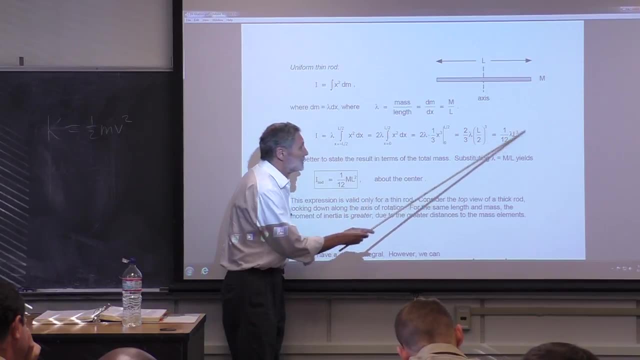 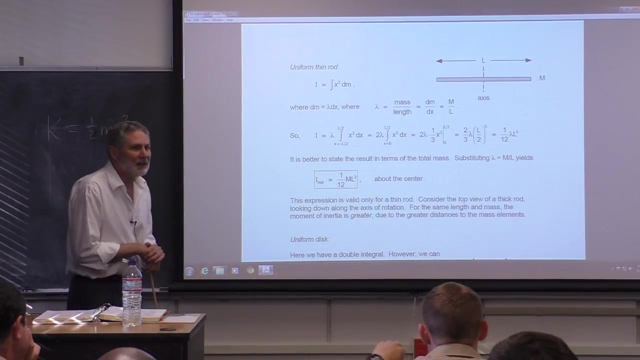 lambda over 2, so I got the 1, 3rd X cubed. I evaluated: upper limit, lower limit, no contribution to the lower limit because it's 0 and we get this result and no one remembers this. okay, I had you know. I look at I go. what is that? the reason is. 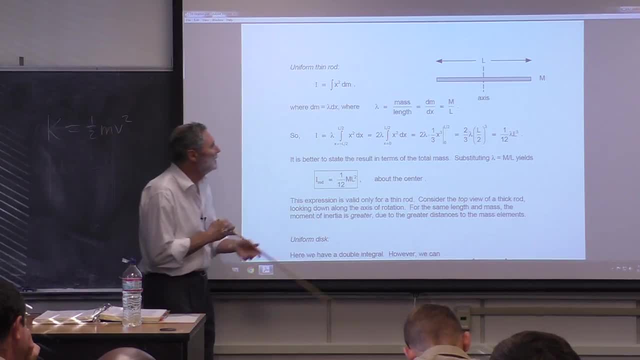 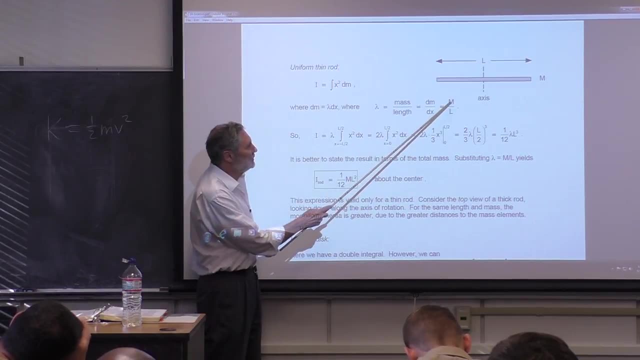 it's it's best. it's much better to get rid of the lambda- the lambda we use temporarily in order to do the calculation of the lambda. it's much better to get rid of the lambda. the lambda we use temporarily in order to do the calculation, but now we're going to go back and substitute the total mass. 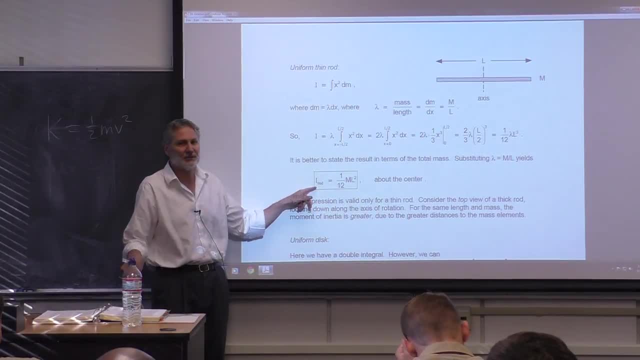 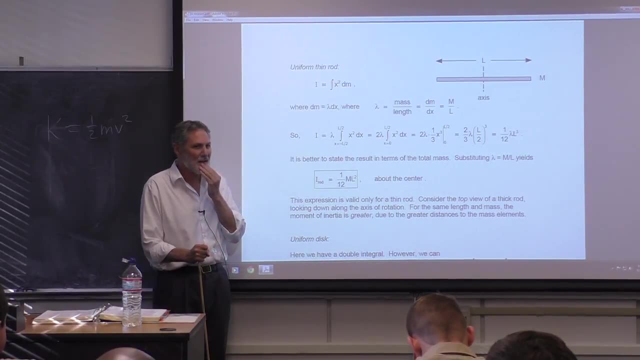 divided by the total length, and now we get the standard result: 1, 12 ML squared. and even this is not that standard. all right, and the reason I'll we will meant. later on in the lecture you'll see why and I'll remind you about this. but 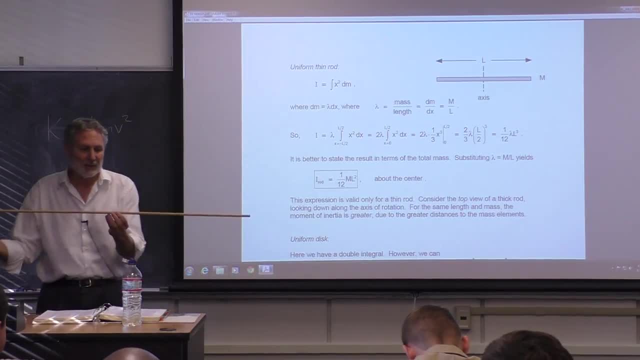 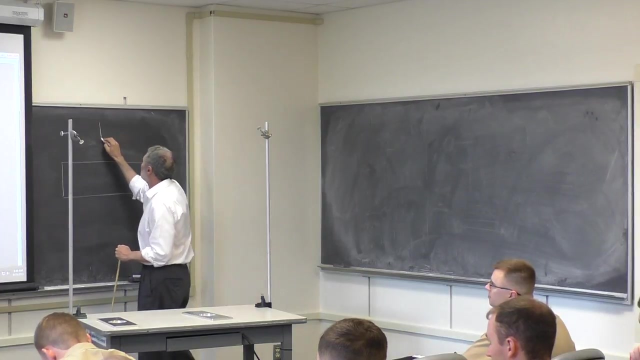 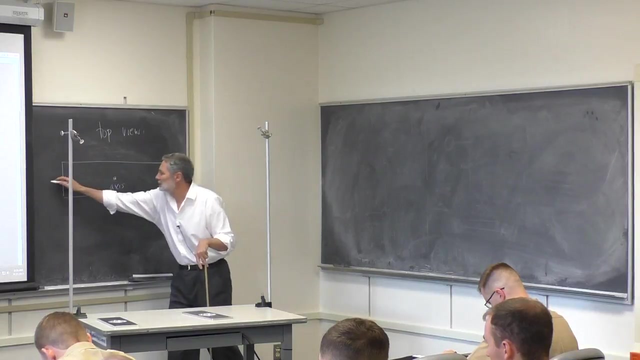 anyway, this is the result for a uniform thin rod rotating about its center. that's the inertia, the moment of inertia. now what if we had a thick rod? so here's the top view. here's the axis coming out at you like this right, and this is going to have some moment of inertia. let me put a dash line here, just. 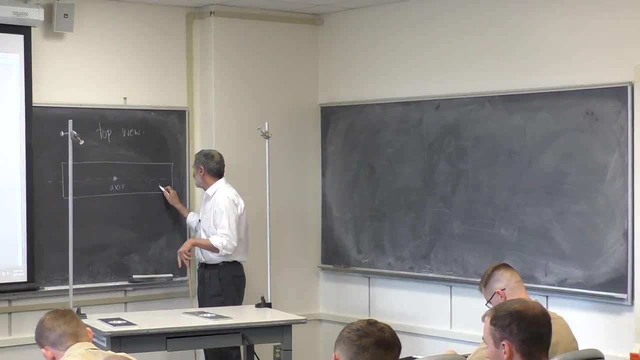 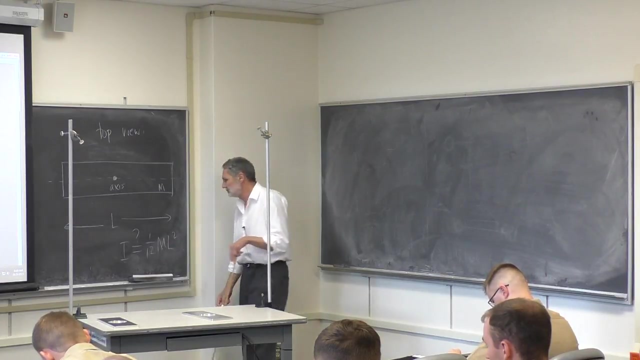 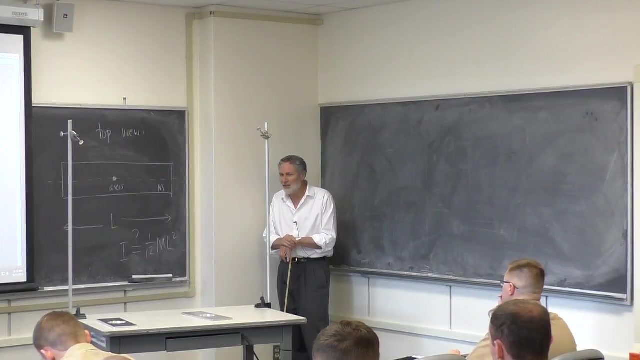 to help. so it's going to have some total mass in. it's going to be some links. here is its moment of inertia going to be 112 in L squared. hmm, what do you think you have to think here? this is it ok? somebody said yes, which is obviously wrong. 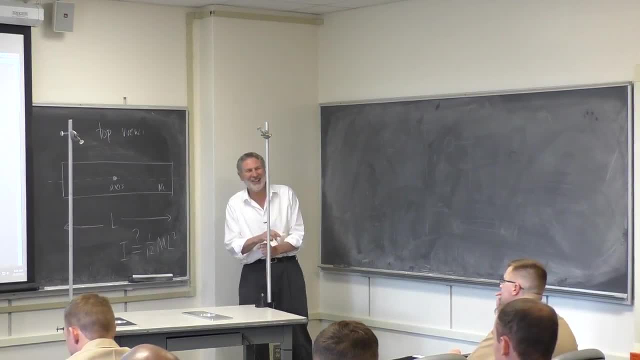 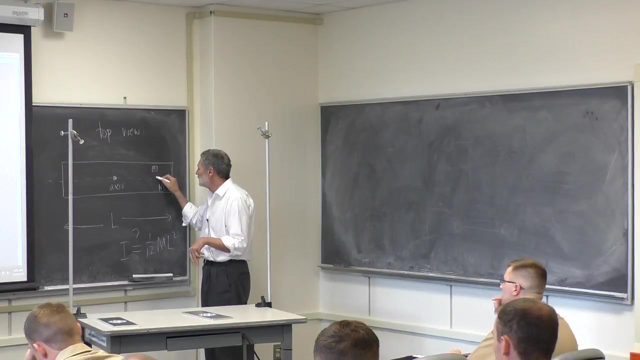 yeah, I'm used to that. you expected that. here's the idea. it's actually very simple. but if you don't see it and you're totally confused, right, let's consider a little mass element here now. before we took this to be down here, right, and we took this length, its actual length here is bigger, you see it. 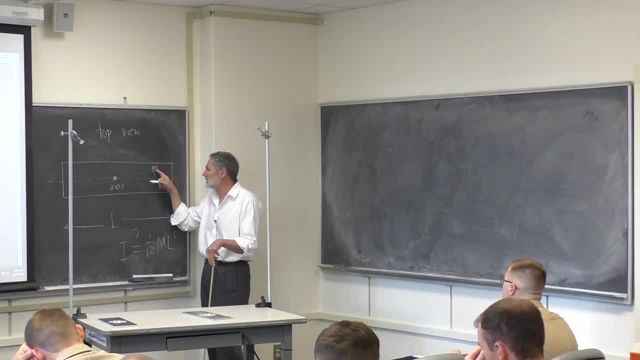 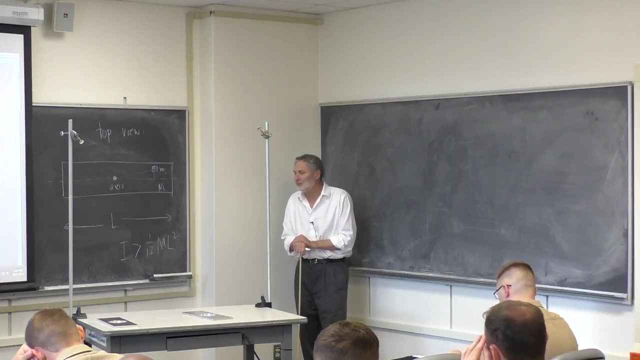 to find the moment of inertia. we don't take this little mass, this mi, here and multiply it by this distance. we got to multiply by this distance. so the answer is the moment of inertia is going to be greater and if you want to know the precise thing, you think- even look it up- business standard thing- it's going to be. 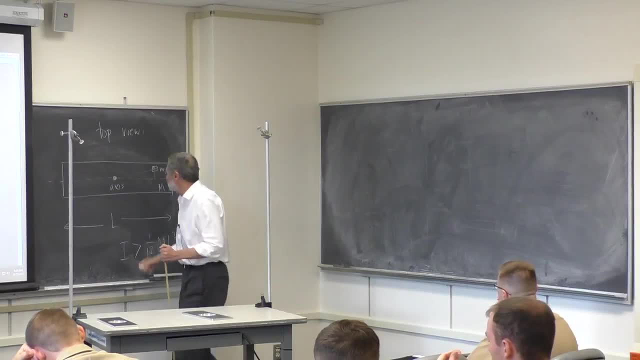 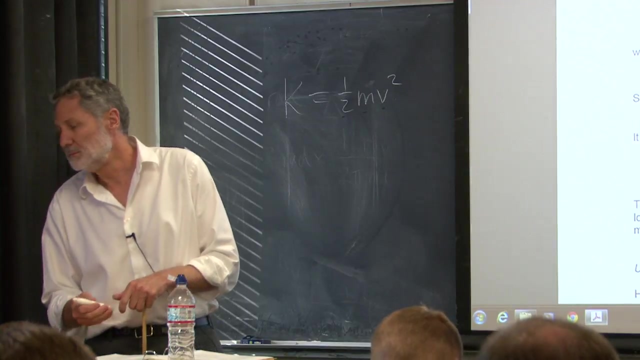 an all introductory mechanics books and will involve this dimension here. you'll need to know this dimension, you need to know that links with it, or the total thickness, whatever. So what makes that different, I guess, then, from the thin rod? Couldn't you do that with the thin rod then as well? 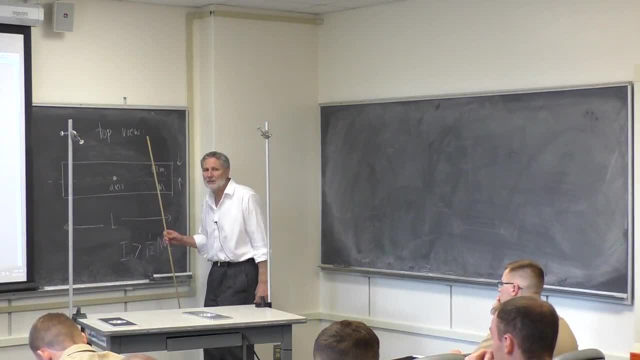 Oh, You can. I'm not sure if this is what you're asking. By knowing the thin rod, you can calculate this. This is really. you can think of this as a superposition of a bunch of thin rods, But you've got to notice here that this thin rod, the axis, is not there. 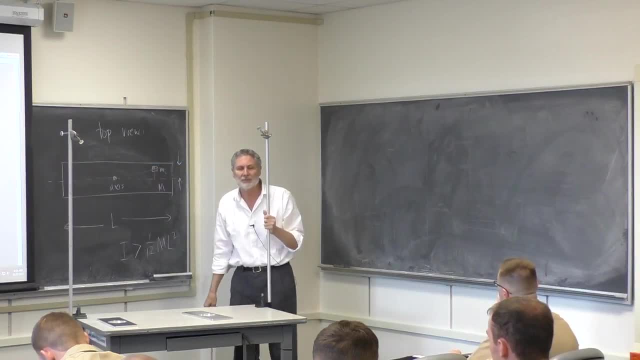 You've got to take that into account. I don't know if that's what you were asking, but that's what you triggered me on. Yeah, You've got to do. look, the bottom line is to get this without looking it up. 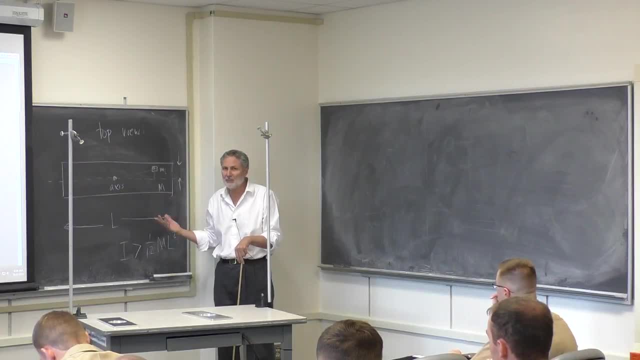 Oh, and, incidentally, I'm sure you can find this on the Internet. Just type in moments of inertia, You'll get more than you want, Okay, So if we were going to do this, we would have to integrate. And one way to do it. there are different ways. 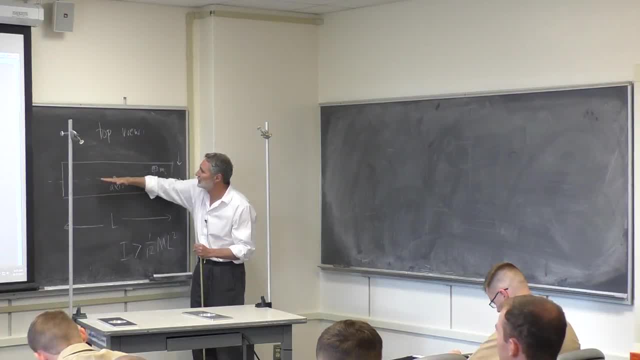 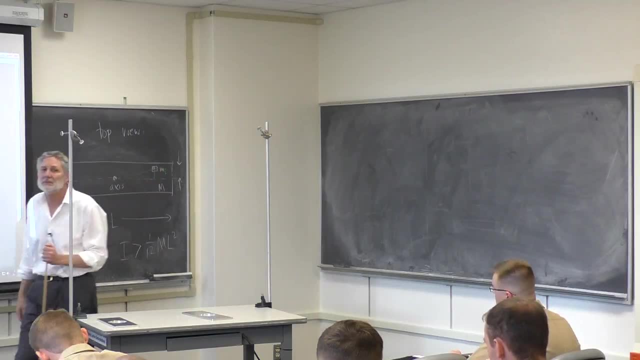 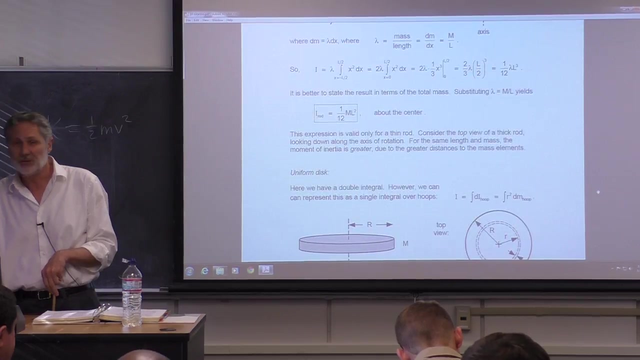 One way to do this is to view this as a collection of thin rods of infinitesimal masses and integrate over all those. That's one way to do it. Okay, next, So the rod is useful. We're going to get use out of this, and we're also going to get use out of a disc. 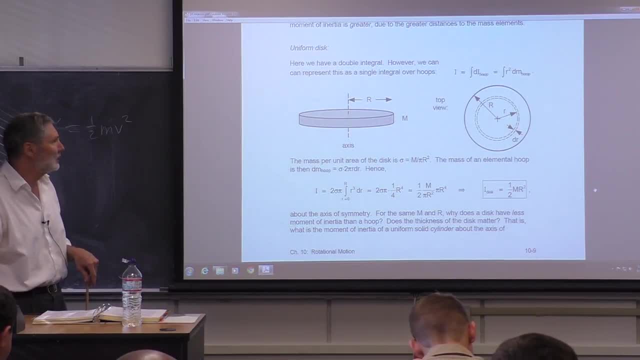 And you can imagine why: Because in the next chapter we're going to be rolling things. We're going to have- look at- axes that aren't fixed, And the main case we're going to consider is going to be an axis moving parallel to itself, like something rolling down an incline. 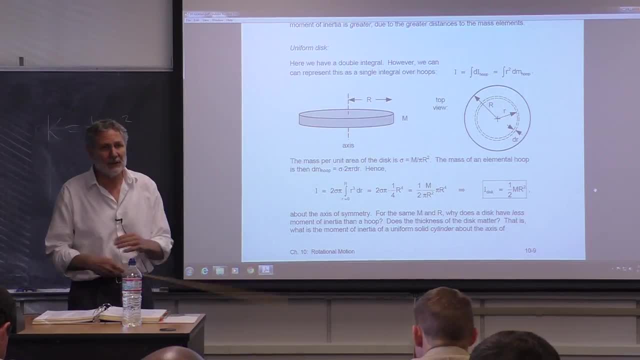 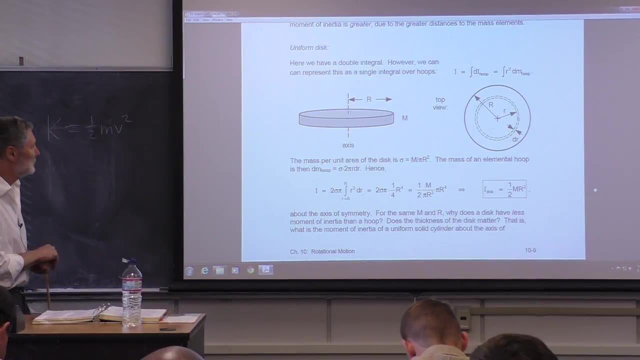 We'll also talk about, you know, tops and gyroscopes, but that gets a little complicated. We'll just talk a little bit about that. So the disc is going to be an important object for us, So we're going to take it to be a uniform disc. 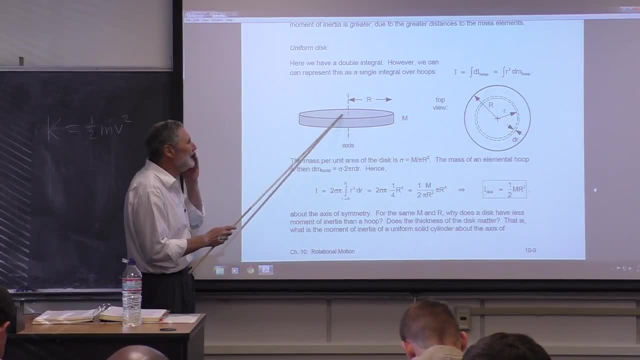 All right, It's not loaded. Okay It's got. its density is constant here. Its mass per unit volume is constant. Total mass in it's got some radius and we're going to do find the moment of inertia about the axis of symmetry right here. 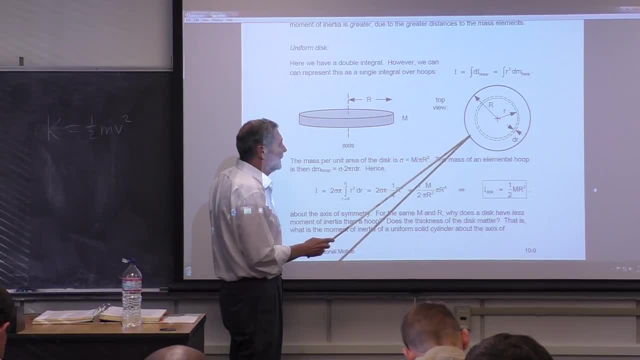 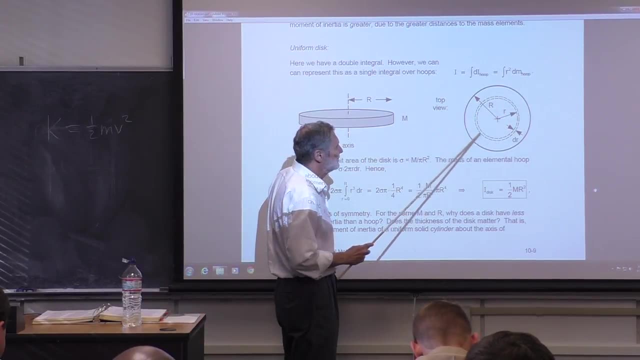 So this is now a double integral. We have a little bit of mass here and I've got to integrate over all little masses and it looks to me like a double integral. So you can treat it that way, You can treat it from a purely mathematical point of view, and you can do that. 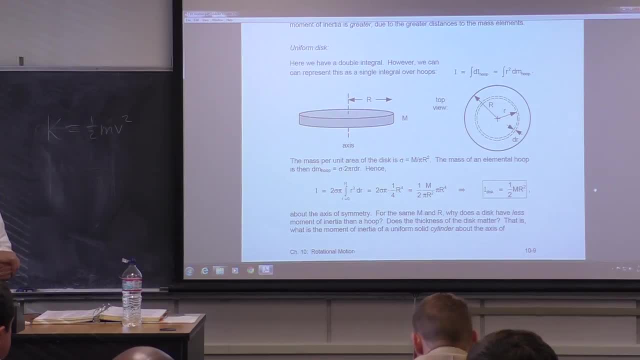 But it's not fun. I don't think, And you're likely to make a mistake. Okay, So here's what we do. This is a standard trick and you may. they do this in calculus. I think We're going to split the double integral into: is there somebody dying out there? 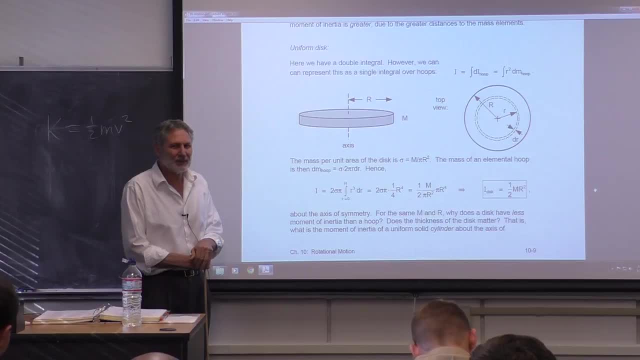 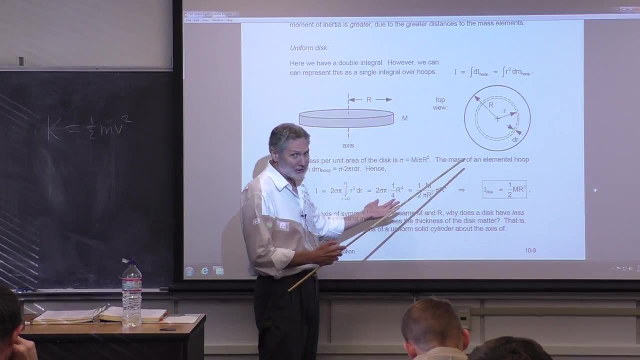 We're going to split the double integral into two single integrals. So what do I mean by that? So this is, I think it's probably done in calculus, but this is definitely how physicists look at it. I can tell you that. 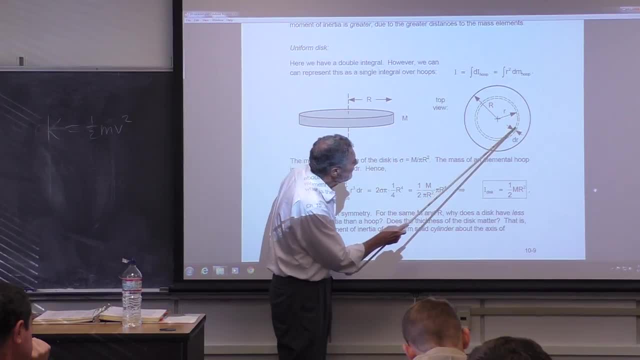 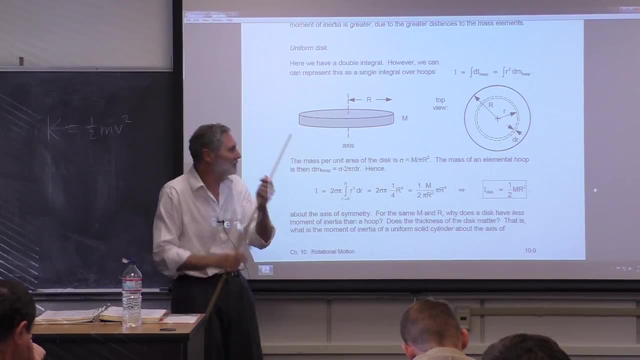 Here's the top view of the disk. I see a little. we're free to choose the element of mass, anything we want to be. Okay, I've been writing it as a little cube or a little square like that. Here I want to think of a hoop. 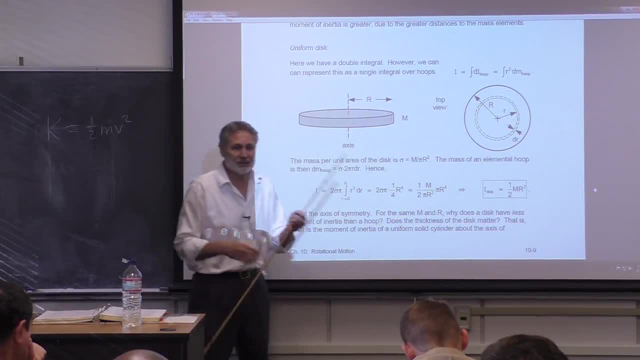 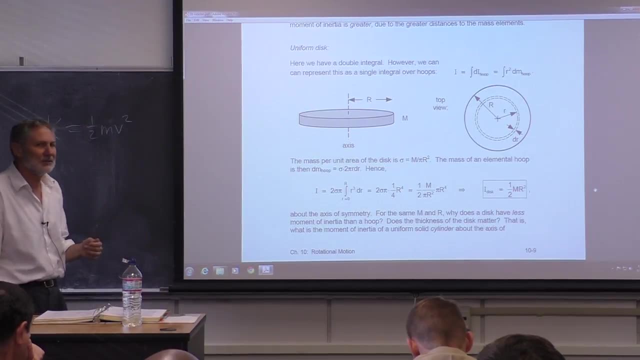 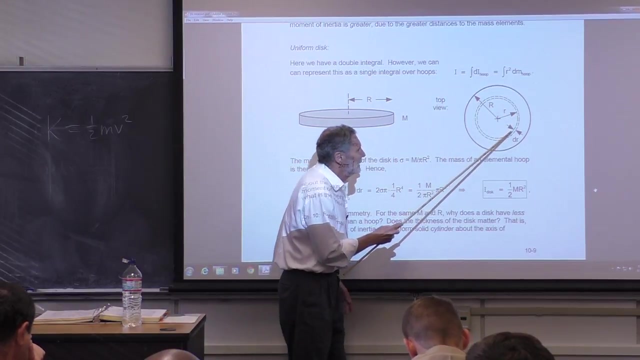 I see a hoop here, So I'm going to think of this disk as a collection of hoops. So it may sound strange to you, But it sounds good, I think. So here's specifically what we mean. Here's one hoop, okay. 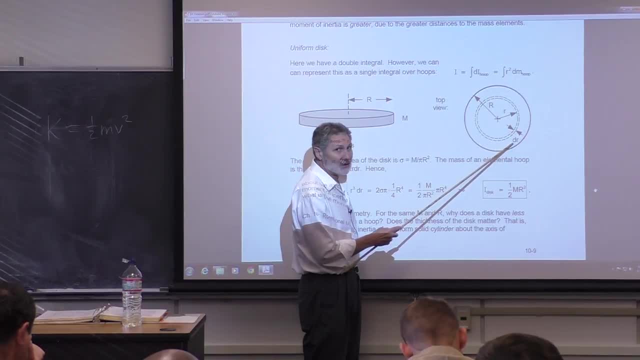 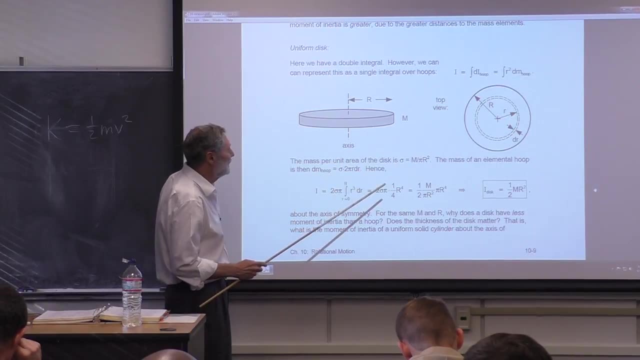 It's an element of mass. It has a thickness, dr. all right, And I know the moment of inertia of this. of that hoop, It's one half the mass of the hoop times the square of little r. all right, So what's the mass of this hoop? 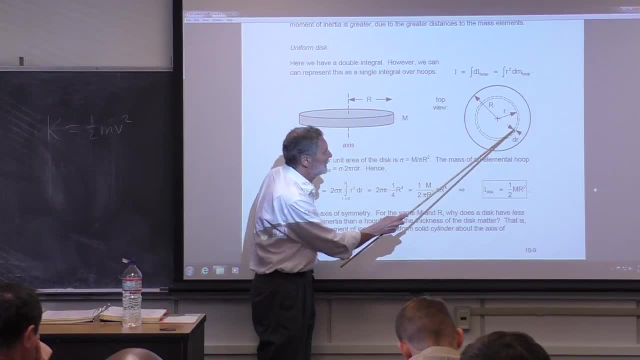 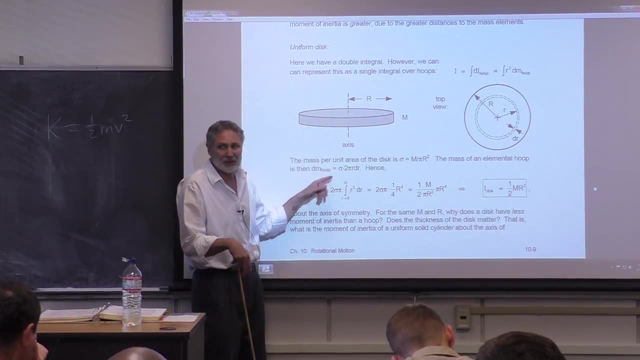 Well, it's a differential, because we're taking a differential thickness here and it's going to be the mass per unit area. Now it's natural to use the mass per unit area. You know, previously it was natural to use the mass per unit length. 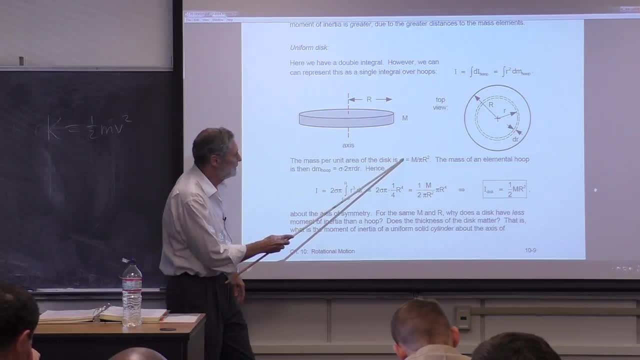 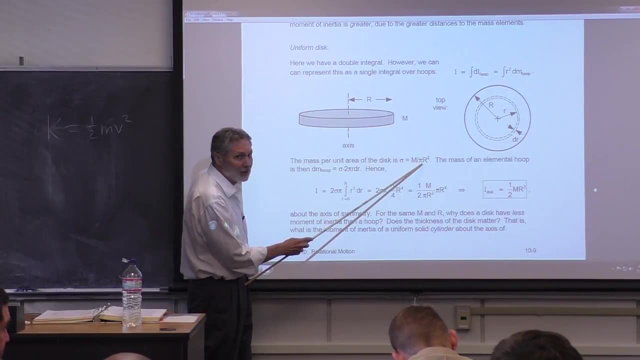 Now we want to use the mass per unit area And that's often called sigma. It's going because the hoop, because the disk, is uniform. it's going to be the total mass divided by the total area. The total mass is m. 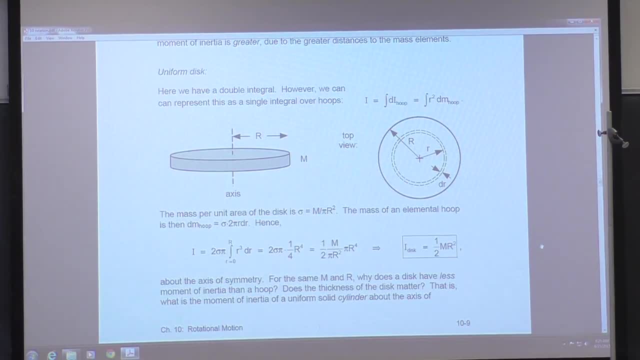 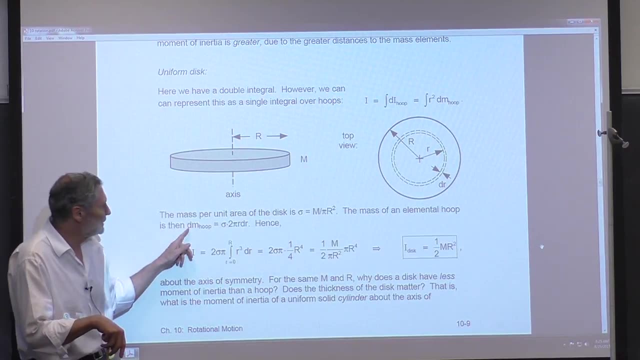 The area of this is pi r Pi capital r squared. So the reason I'm doing this is because now I can write down what the mass of this elemental hoop is. It's the mass per unit area times the area that you see here of the hoop. 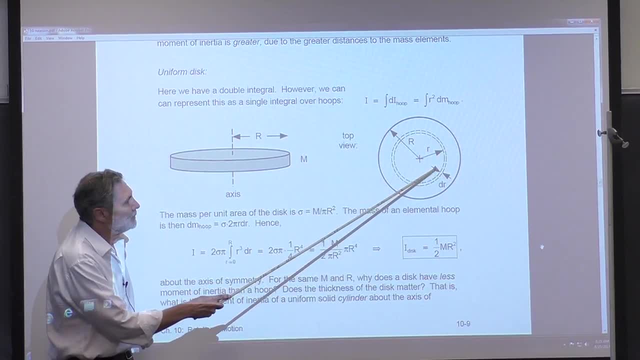 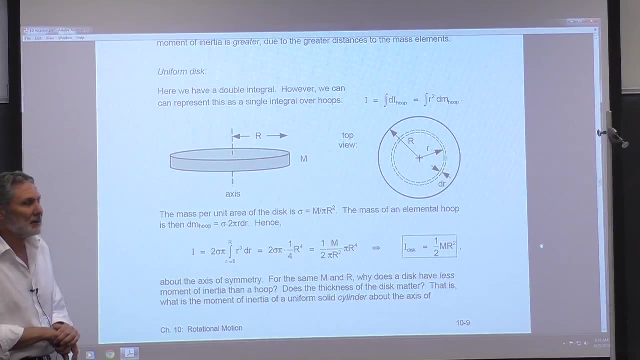 And what's that? That's the circumference times the thickness. So there's the circumference and there's the thickness. Now, once you realize what I just said here- and it probably takes a little getting used to right- I have to think about it a little bit. 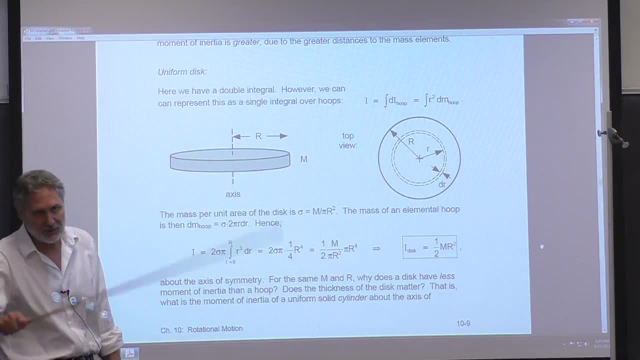 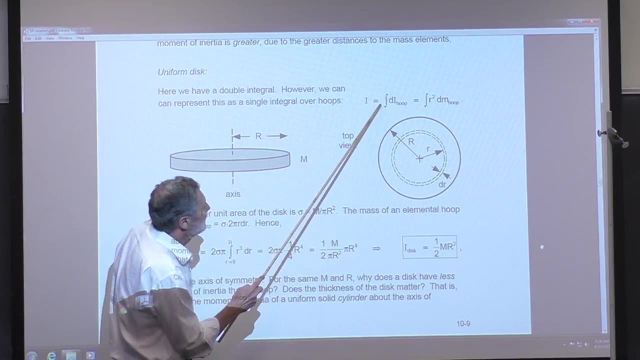 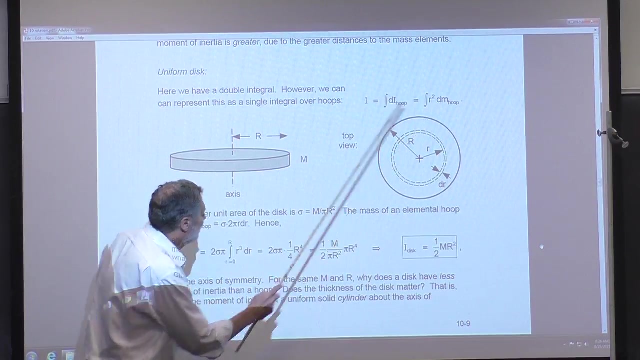 Once you see it, The rest is easy. It's just turning a crank. okay, So the here it is. We integrate over all these little elemental hoops, which is: each hoop contributes r squared times its mass. So we substitute for what the mass of the hoop is in here. 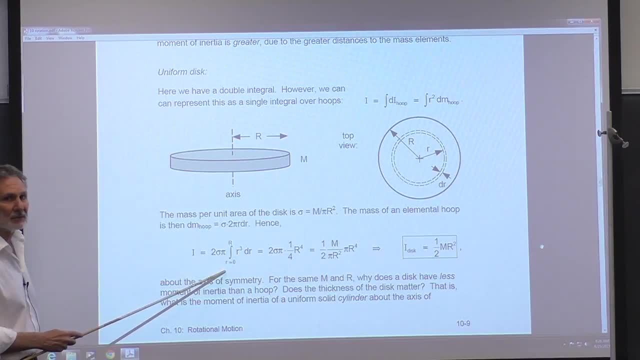 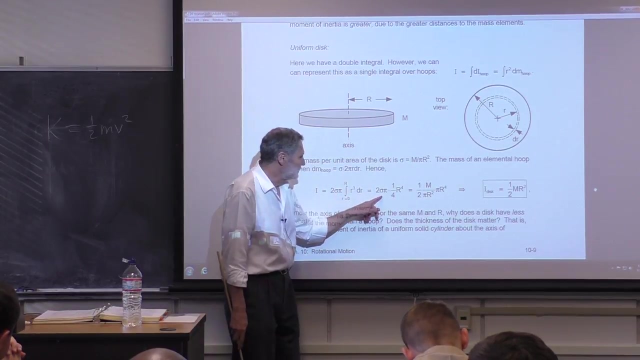 And now we have this is calculus Integral. we can, everybody can integrate this. The integral of r cubed Is going to be one-fourth r to the fourth and I evaluate it and I get this. And again, nobody remembers this. 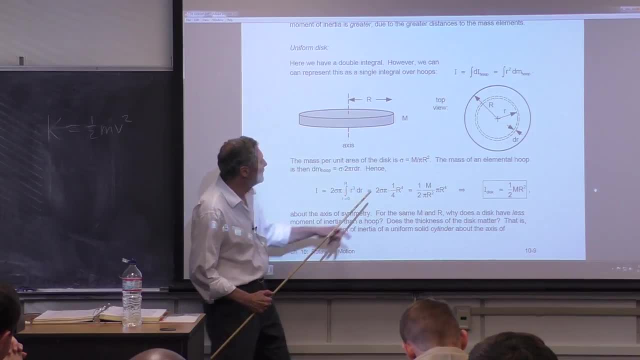 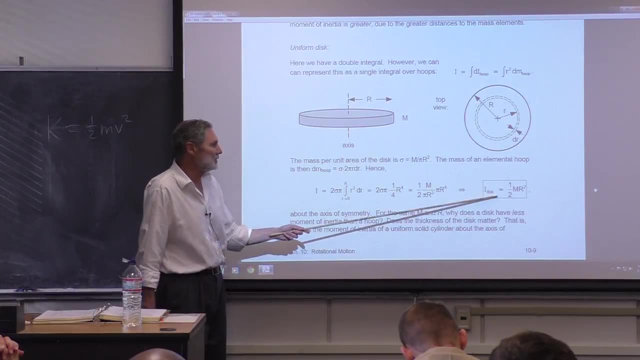 You want to now substitute what sigma is. Remember, sigma is the total mass. We did a similar thing with the rod right. You substitute it in simplify and you get something that you will not be able to forget after taking this class, because we're going to use this so much. 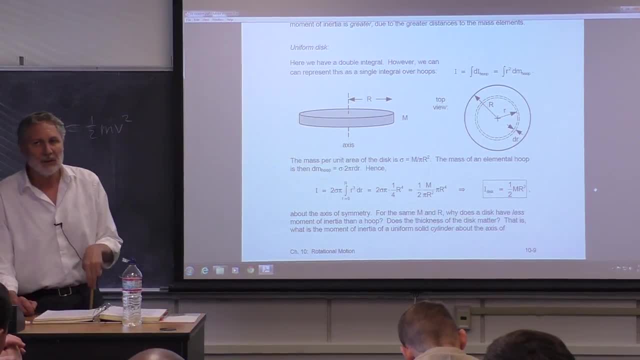 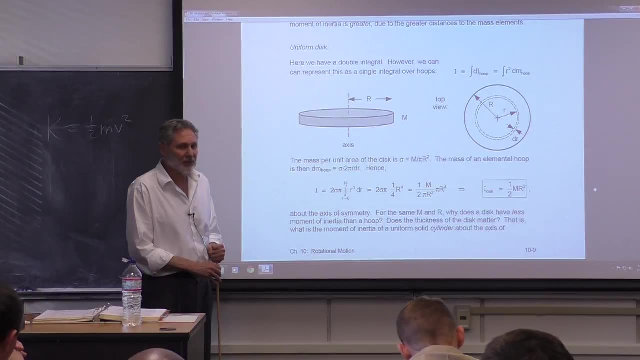 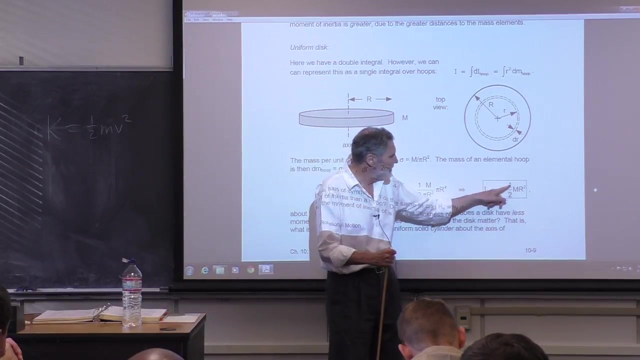 It's one-half the mass times the square of the radius. The moment of inertia of a disc about its axis of symmetry is one-half the mass times the radius of the disc. It turns out to be a nice simple factor here. Why is there a factor there? 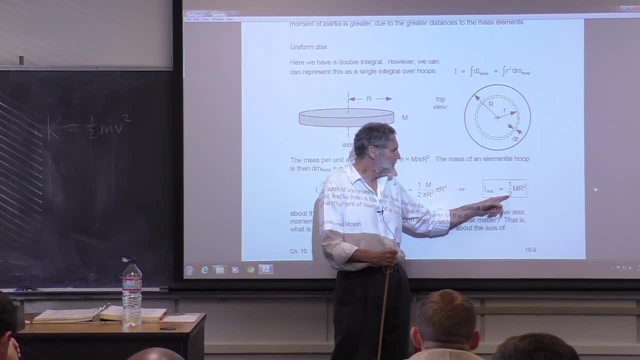 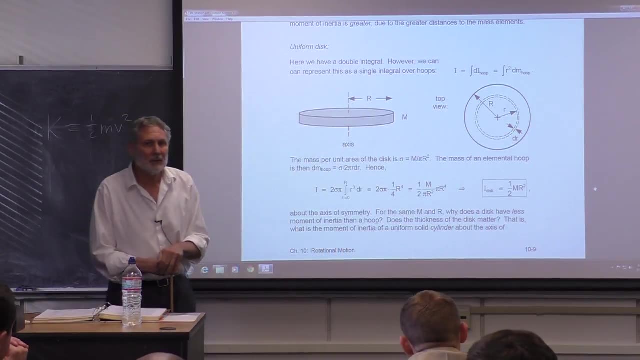 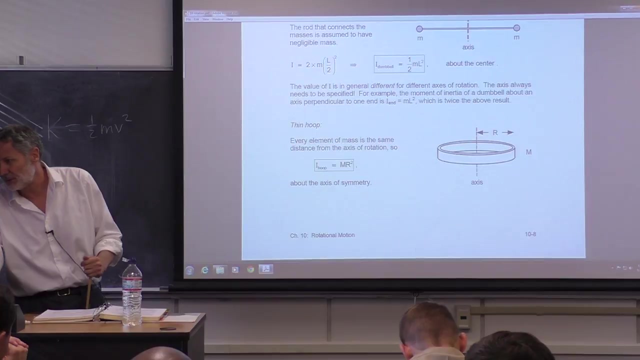 Why isn't it for a hoop of the same mass and the same radius? we have half the inertia here. Why is that? A hoop has is integral. It's m? r squared right. That follows immediately from the definition. I should have written that. there we go. 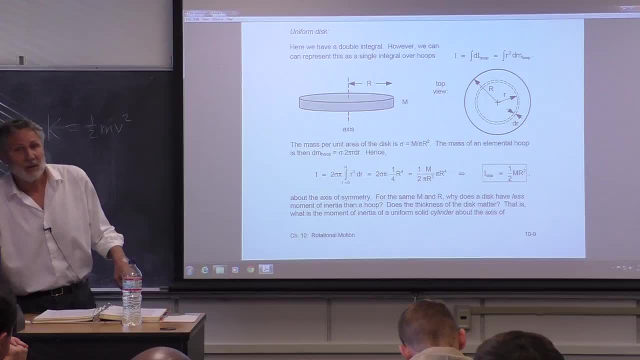 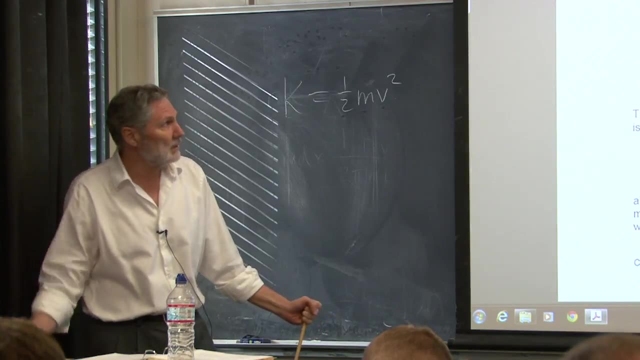 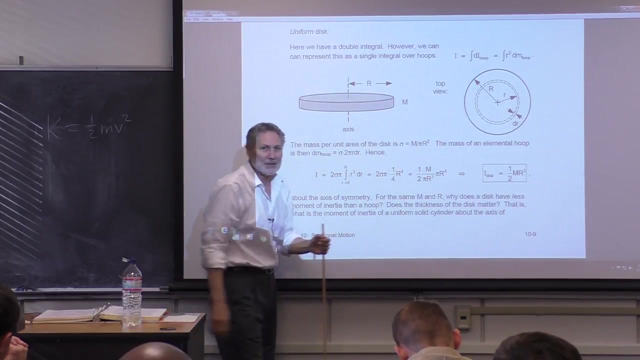 Okay, now we have one-half. Why is it less? This is a simple, simple question. Because the mass is spread out. Yeah, the mass is. you know, you can imagine starting off with a hoop To get to the disc. we've got to migrate some of that mass. you know we've got to migrate. 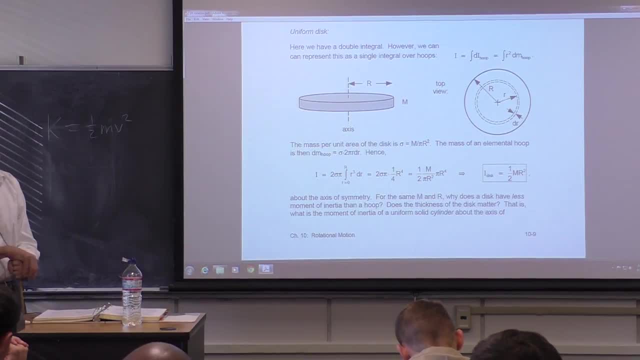 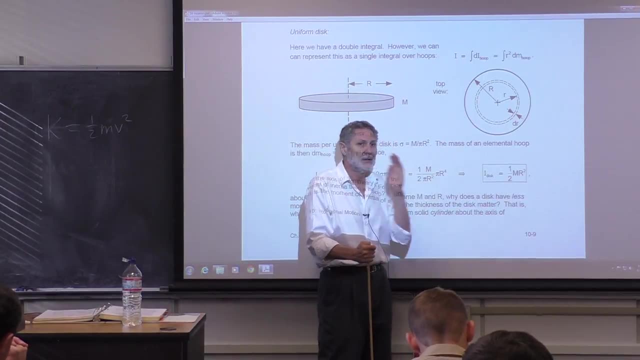 the mass towards the center, spread it out towards the center. We're going clearly going to be reducing the moment of inertia. And it just turns out here that it's a very simple answer. It happens to be one-half. I don't know if anybody has a physical argument for that. 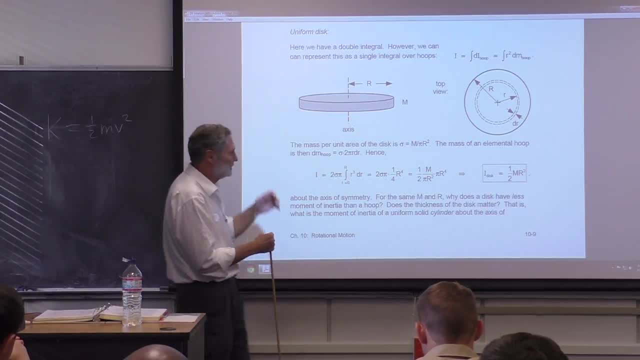 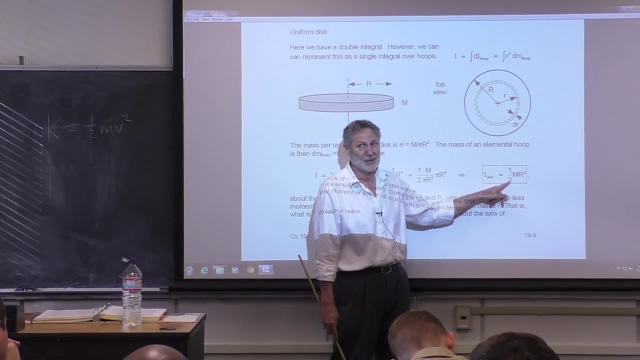 But the the integration here shows that it's simply one-half. But we would definitely expect a number here between zero and one. This coefficient here has to be between zero and one. It's got to be, And it turns out to be a half. 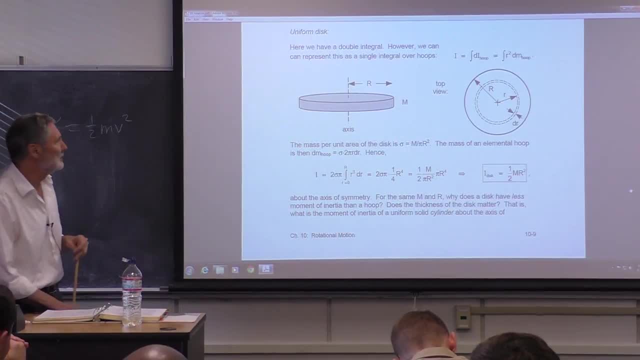 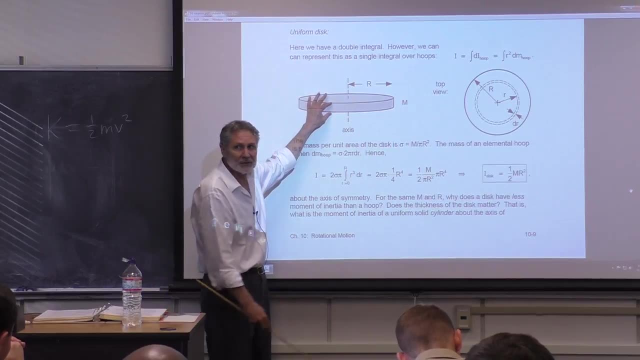 Easy to remember. Oh, here's something. Where's the thickness? There's going to be some thickness here. How come that's not in the answer, in our, in our expression here: Yeah, m is in there, R is in there. 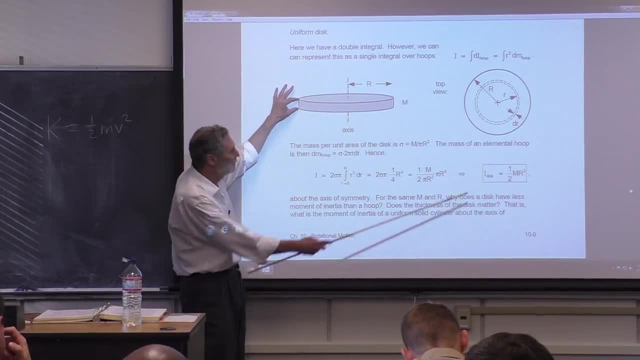 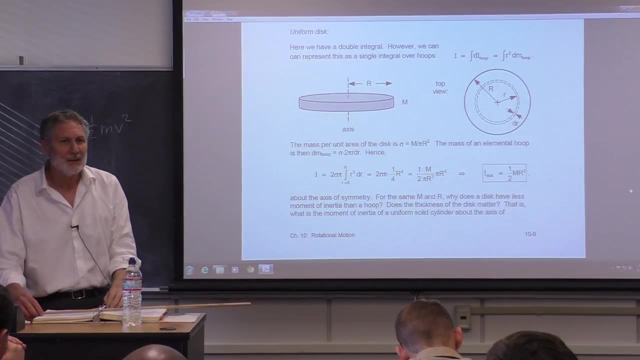 What about h? Call that little h. How come h is not in there, If you, if you reduce r but keep m, the same h will increase, you know so it's. you only need m and r to define the distance. 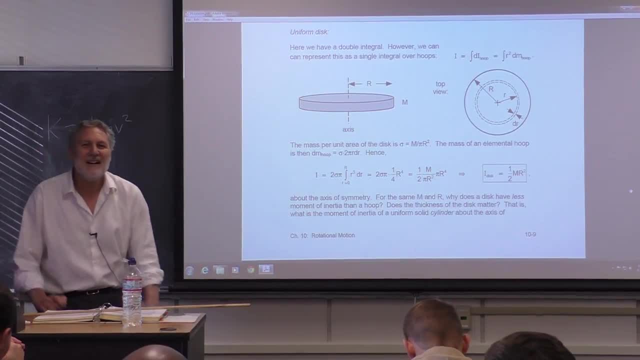 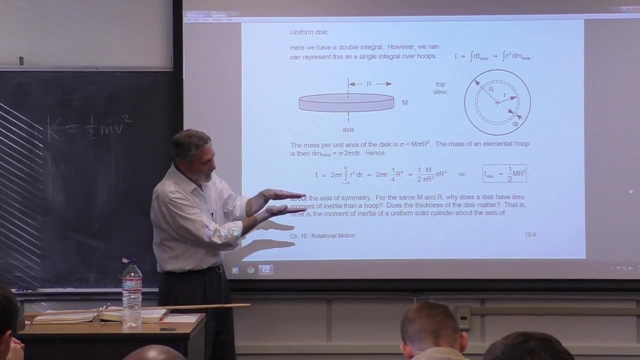 Hmm, Huh, Yeah, let's look at it from a different point of view. Suppose I took this disk and I imagine spreading it out. All I'm doing, I'm trying, I'm just spreading it out. I'm keeping r the same, m the same. 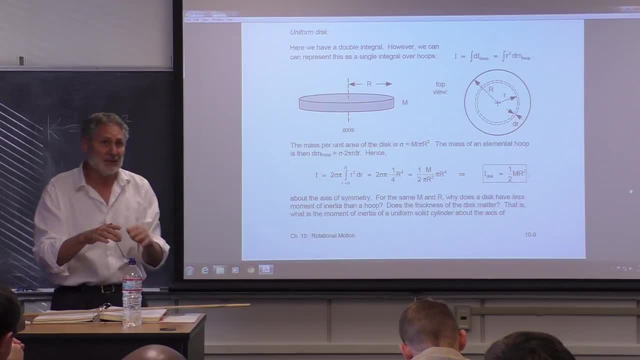 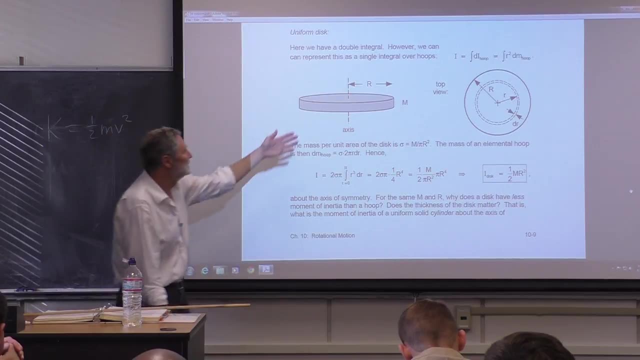 It's density. You're, you're, Mitch was fixing the density. okay, Let's not worry about that. Let's just imagine spreading. How's the moment of inertia going to change? What if this is a cylinder instead of a disk? you know something like this. 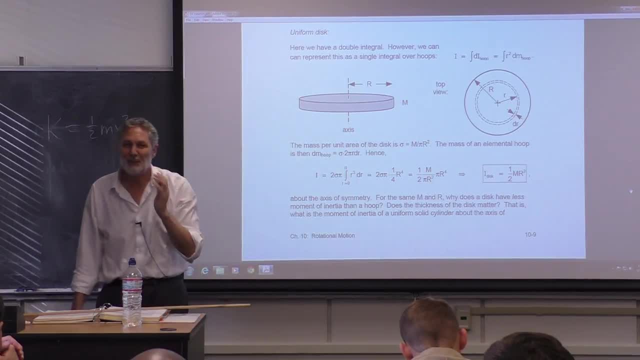 What's the moment of inertia going to be about the axis of this? It's going to be the same right, And the reason is every little element of mass. its distance to the axis has not changed When I spread it out like this. now, this is not a practical thing. 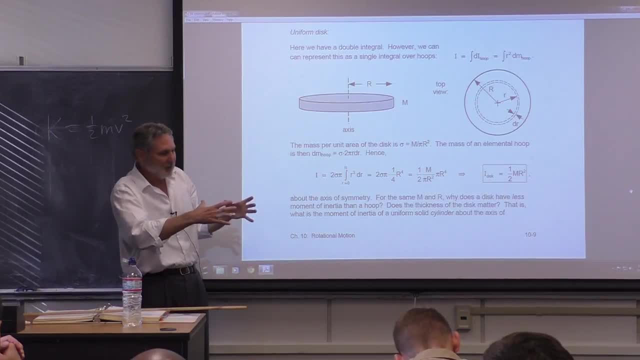 If you- and this is what Mitch was thinking- If you tried to do this, this, its radius is going to go down right. If I take something and stretch it, it's going to compress. That's because it's trying to keep the density the same, okay. 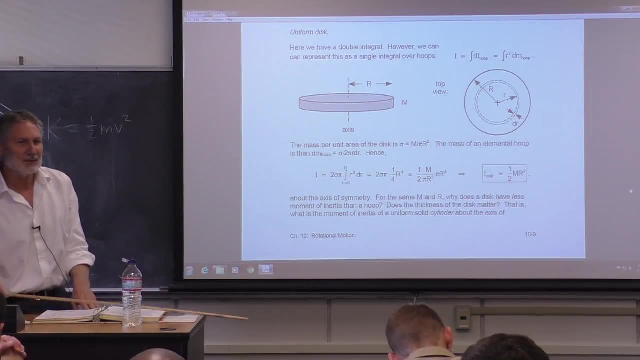 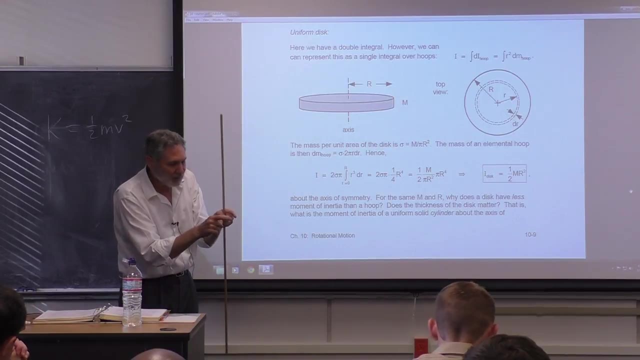 But this is just in our, this is a Gedanken experiment here. okay, This is just a thought experiment. If I imagine spreading this out, every little bit of mass is going to stay the same distance to the axis, so the moment of inertia can't change. 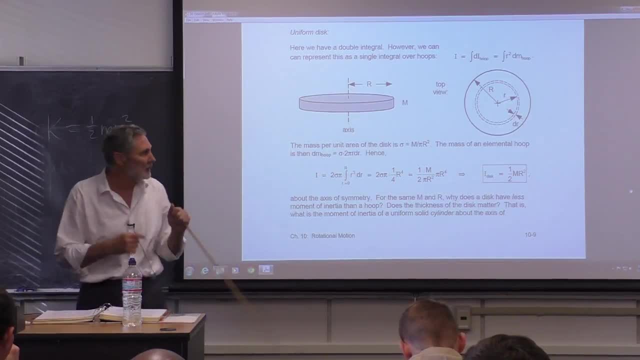 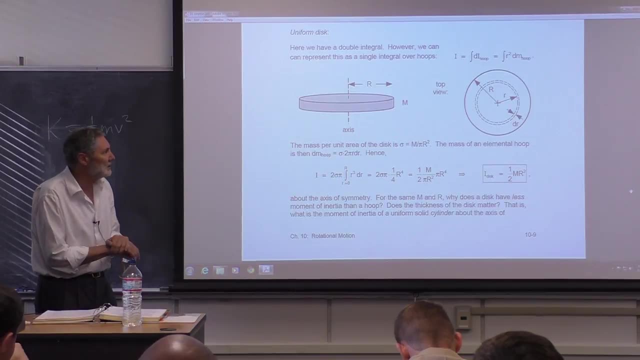 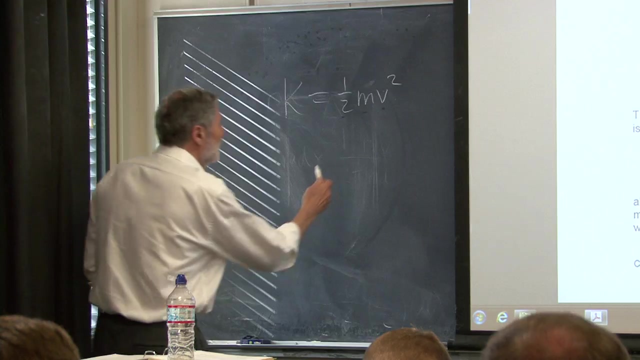 That's why h is not in here, That's why it's not in there, this height here. So we can. one way of summarizing this is that the moment of inertia of this, what we think of as a disk here, is the same for the same mass and the same radius. 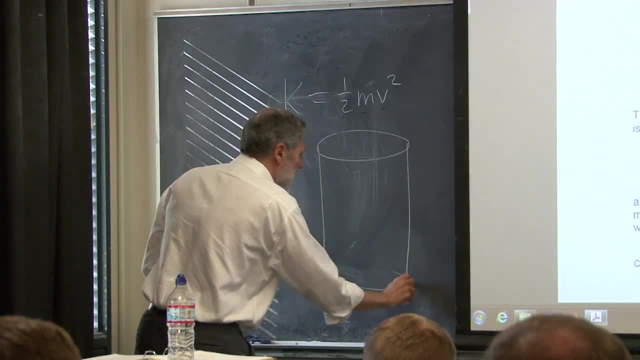 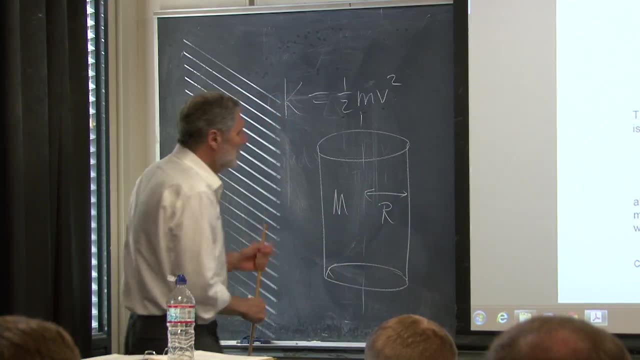 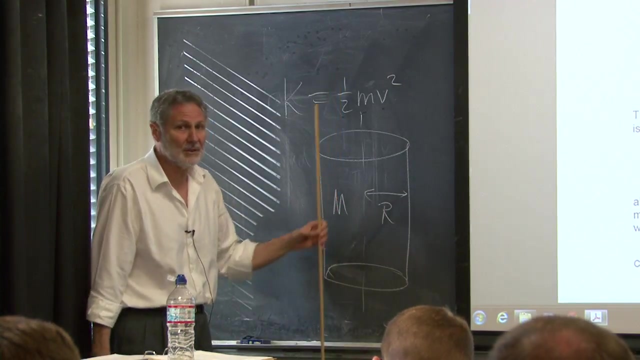 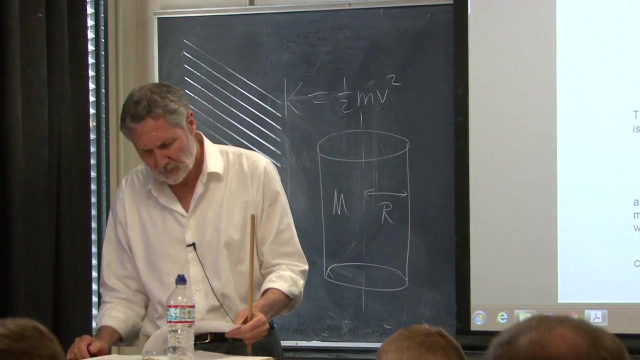 It's going to be the same. if you have something that we would normally call a cylinder right Of a mass here and a radius here, The moment of inertia, the rotational inertia presented by this object here, is going to be the same as the disk. 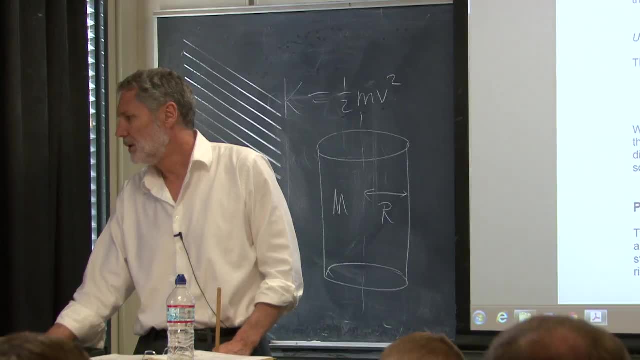 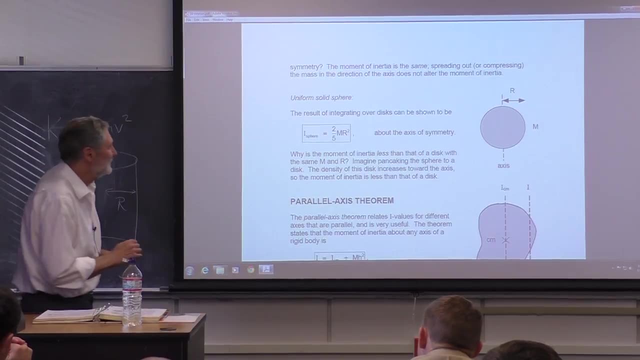 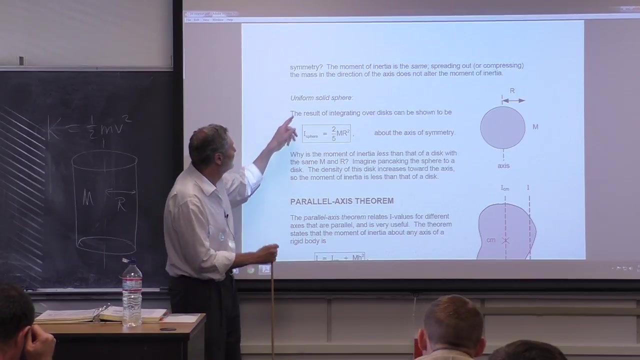 Okay, any questions or comments? Okay, So another. Obviously, We're headed towards rolling objects. in the next chapter We want to deal with spheres. okay, Now I want to emphasize something here: that this is a uniform. there's two types of spheres. 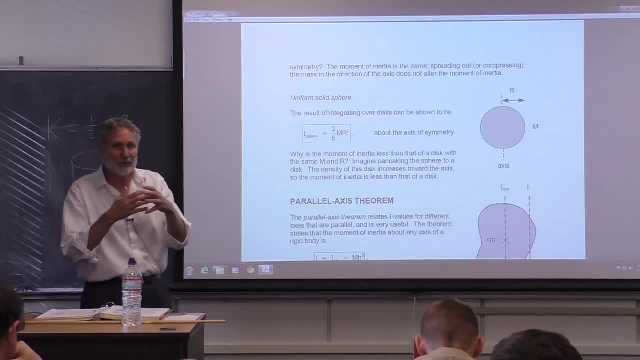 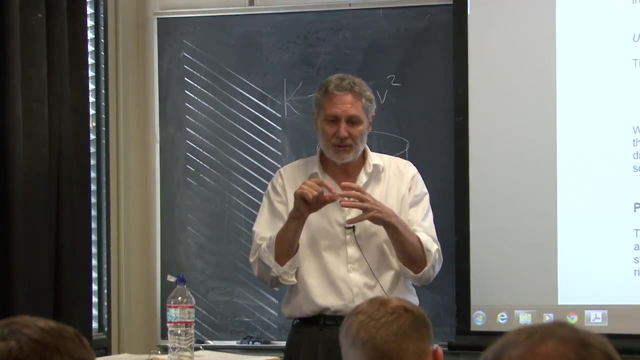 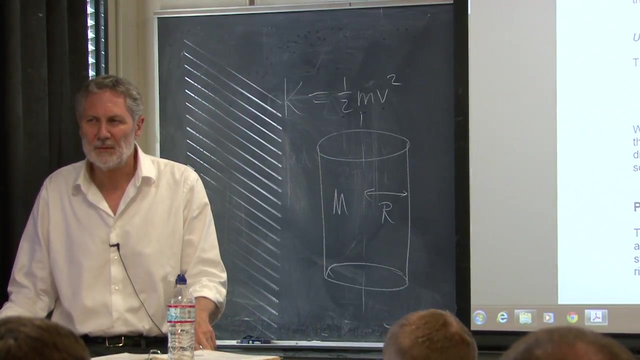 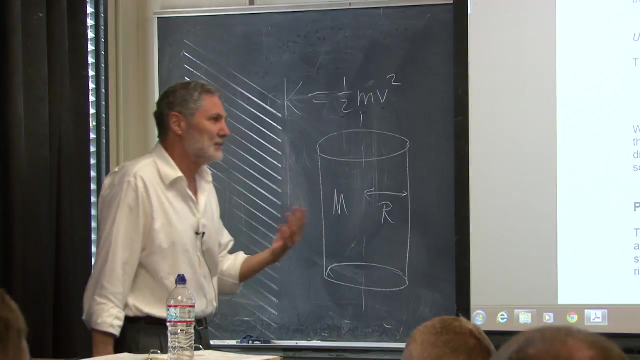 that people typically deal with. There's a uniform, solid sphere like a billiard ball, And then there's a spherical shell which is it could be thin, And we have that. We have a lot in the demo lab. It's one of the reasons that it looks so messy and is messy. 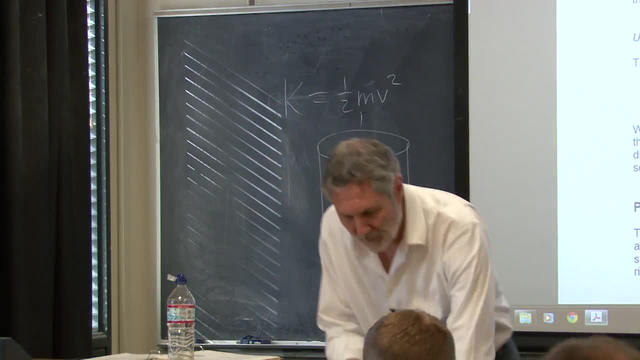 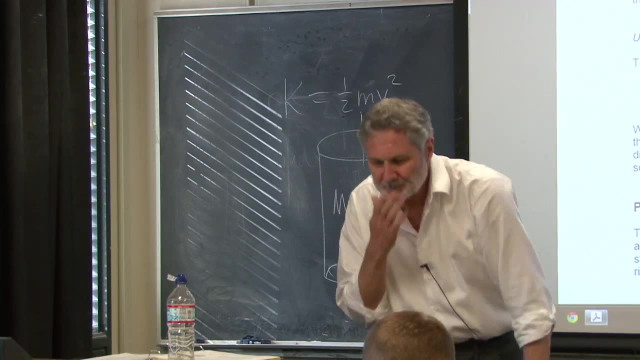 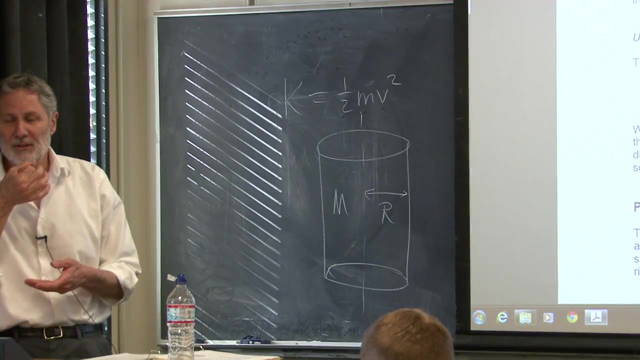 Yeah. So I just want to make a note. I might bring that up. I normally don't show that That's done for an acoustics demonstration Because it has a hole in it. We made a hole in it And then you blow across it. 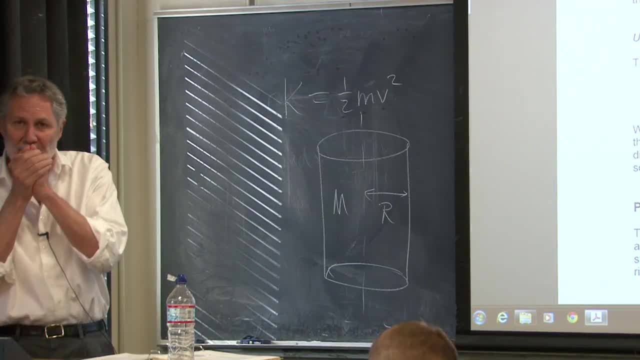 You blow across the hole and you hear a tone, Right, It's like this. Do kids still do this? It's really annoying, Right, And I remember when I was a kid And our parents it drove them crazy, I think the elementary school we went to, I think they like, passed a law saying you. 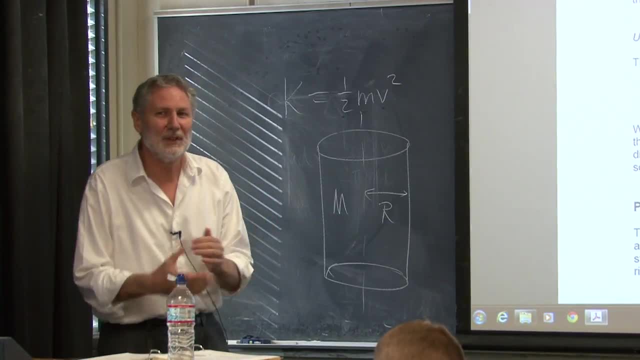 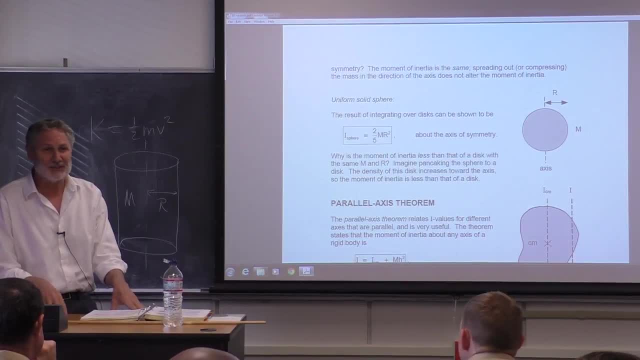 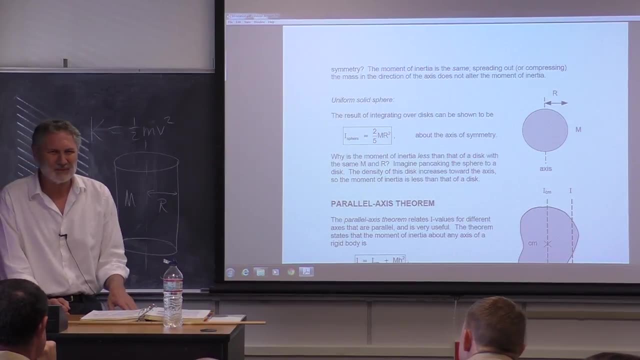 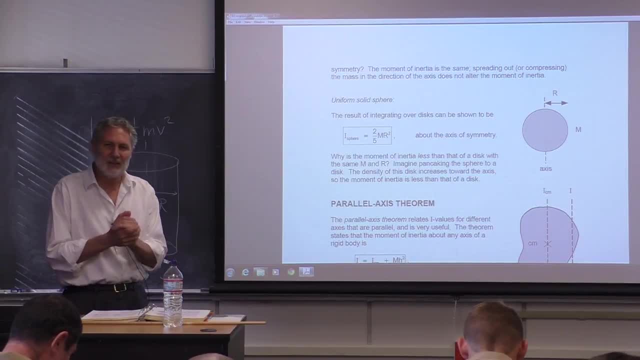 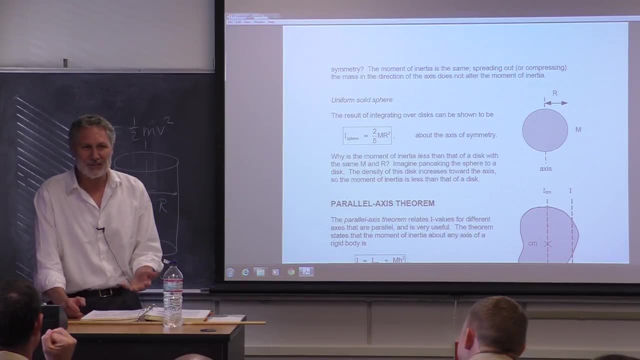 And you can't do any gestures that the Three Stooges do. Now I don't know if you guys ever seen the old Three Stooges movie audience laughing. Yeah, they had these gestures And they were so popular They said, no, that's it. 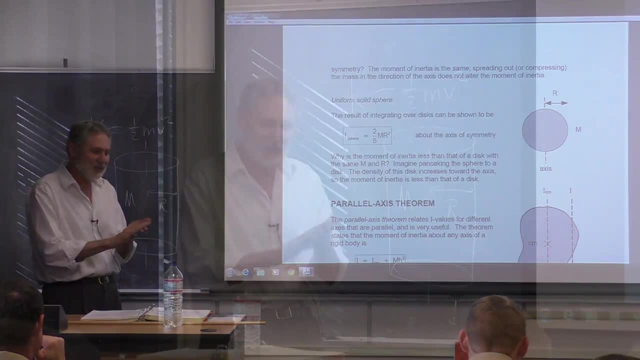 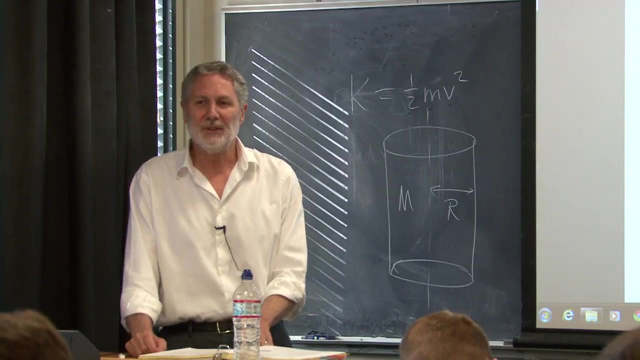 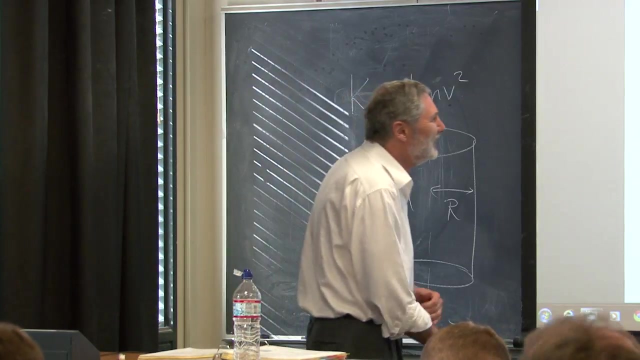 We have a law now You can't do that. And we said, OK, you know, we just did what we were told. You know, duck and cover. We ducked and covered, you know, Okay. so how do we find the moment of inertia? 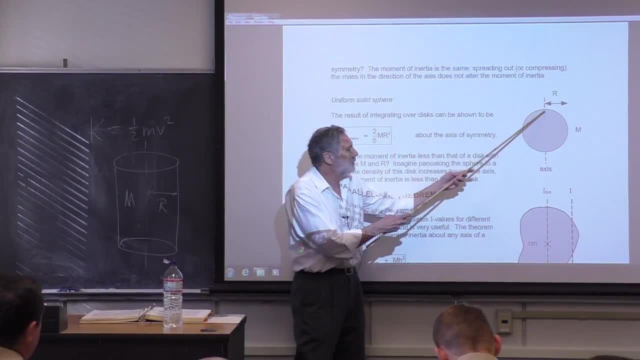 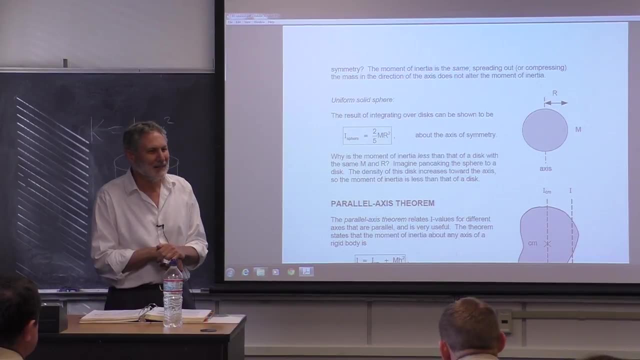 of a uniform solid sphere about a diameter. here you know an axis going through a diameter, Hmm, Okay, well, it turns out. I think probably the easiest way to do it is to imagine that we have a collection of hoops again. 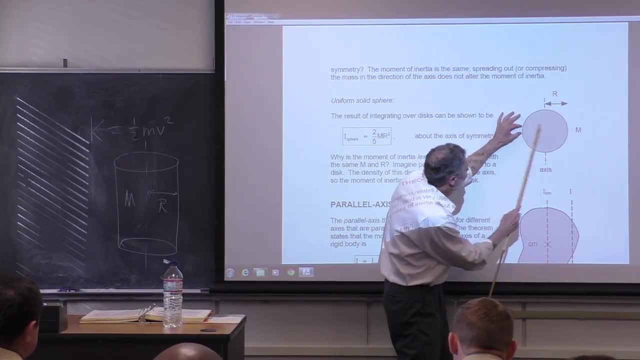 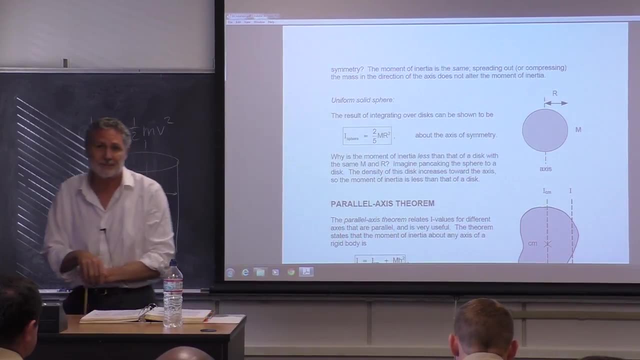 but the hoops are going to have a varying height. you know, I see a hoop here, the next one in is a little higher. you have to be. it's going to cause their mass. it takes a little bit of effort. I think I looked in the. it's not in the text. 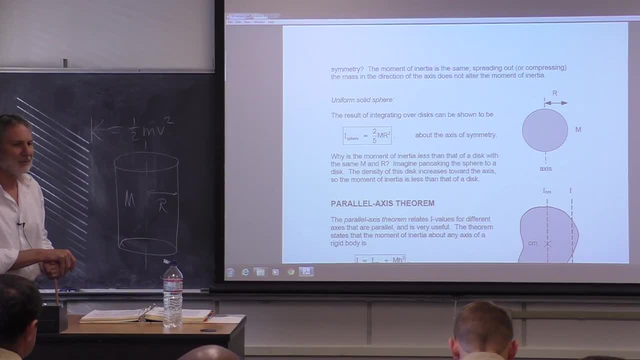 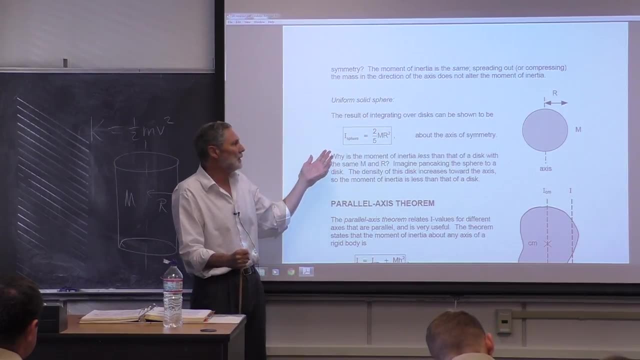 it's probably a homework problem in the back of the chapter, but I don't think we're going to do it. okay, If anybody gets interested in how this is done, you'll find the derivation somewhere on the internet And you can always come by and talk about it. 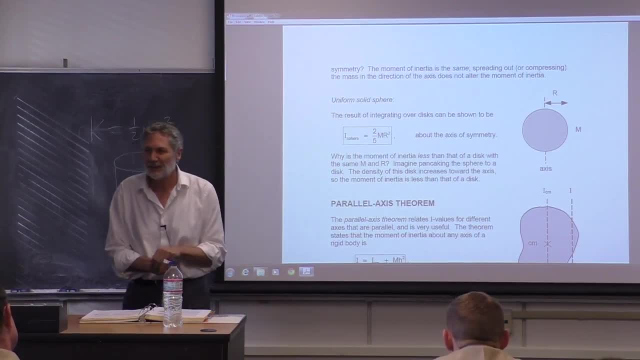 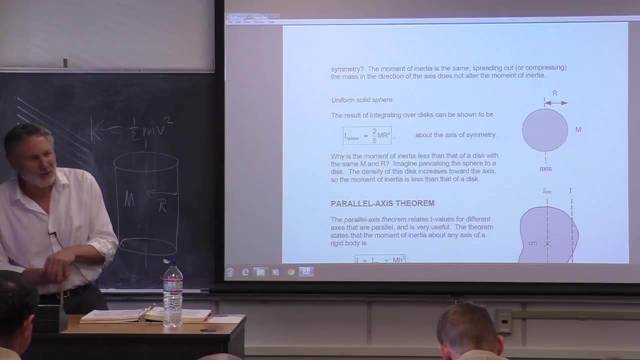 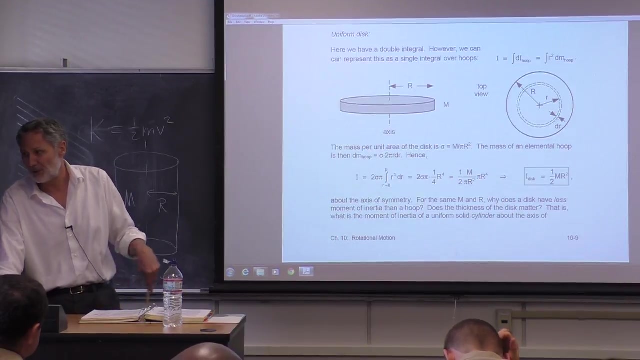 but here's the answer: it's 2 fifths m r squared, 2 fifths. So you'll notice here what is it in comparison to a disk of the same mass and the same radius. Remember the disk 1 half m r squared. 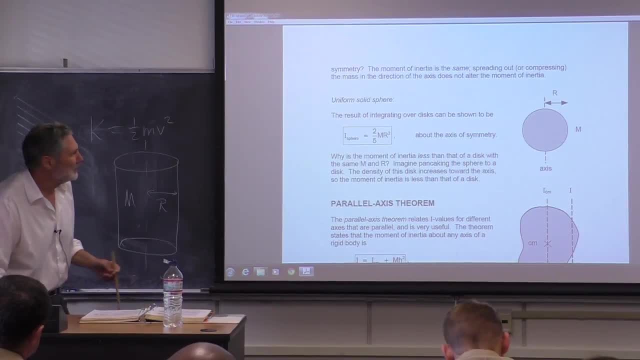 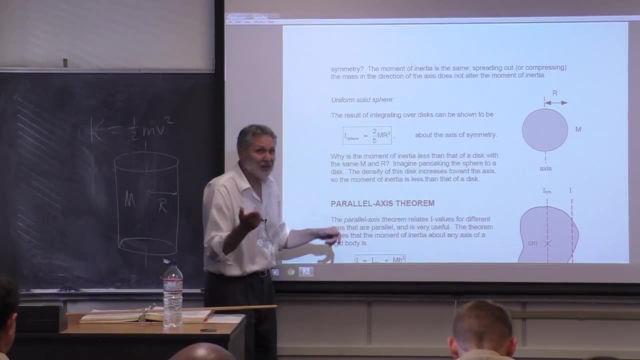 2 fifths is less than 1 half. So can we qualitatively explain that? If I tried, if I took this and compressed and got Duncan, I got Duncan compressed to this. okay, I'm imagining compressing this down. 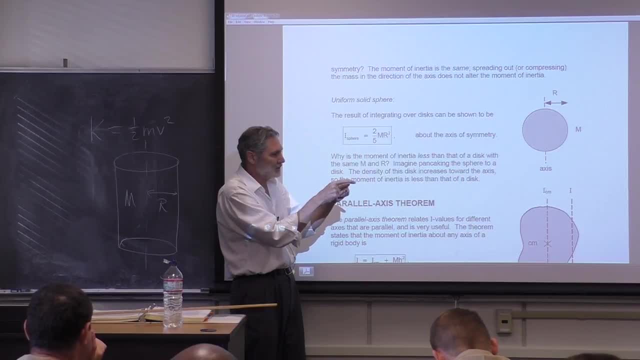 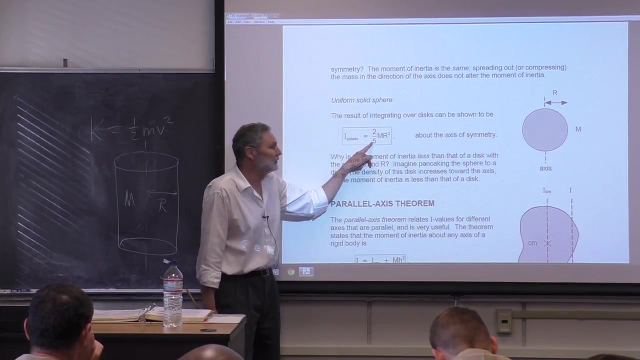 with each mass element staying the same distance to the axis. okay, Do I get a disk, A uniform disk? It's greater density towards the center, So that's going to lower. And look at that, That 2 fifths is less than 2 and a half fifths. 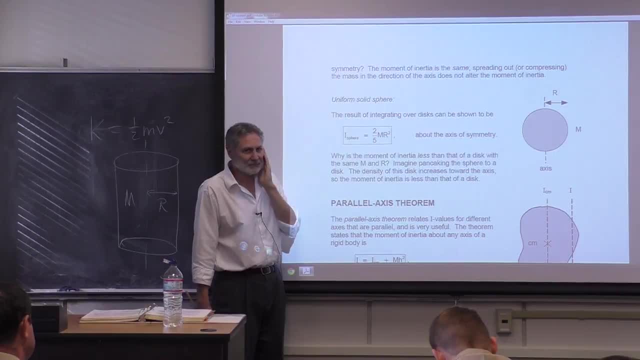 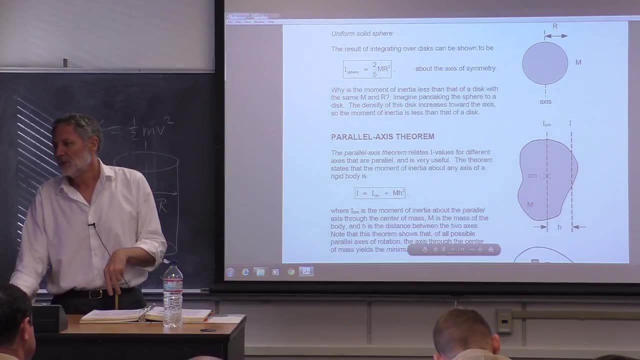 2 fifths is less than 1 half. What's interesting is, it's not that much, It's less, You know, but that's qualitative, It's in qualitative agreement. Okay, enough moments of inertia. right now Specific cases. 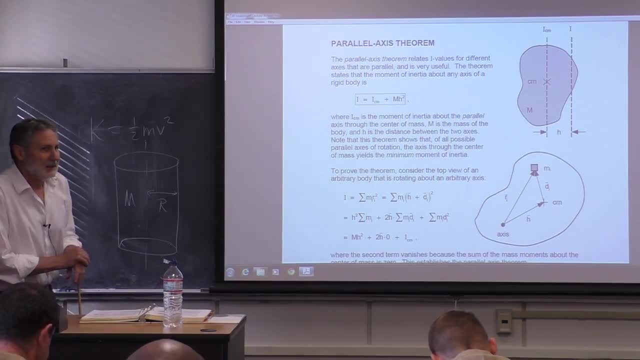 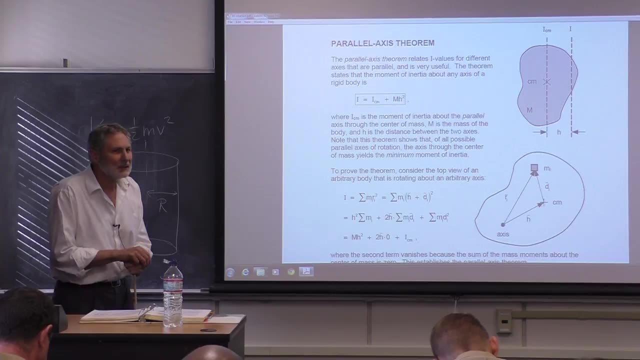 That's going to get us a lot of mileage knowing those. The next thing is this theorem. It's got a great name. It's called the parallel axis theorem. Which it's called that because it has to do with parallel axes, And it's remind that's reminding you. 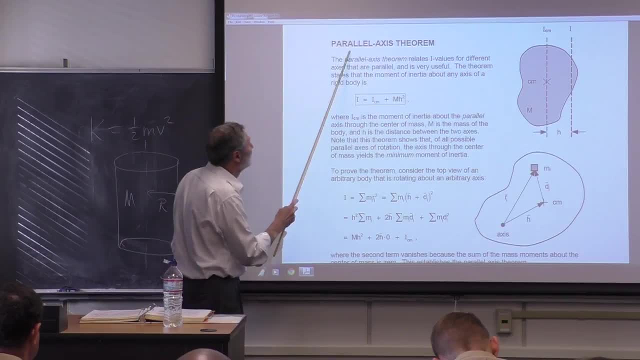 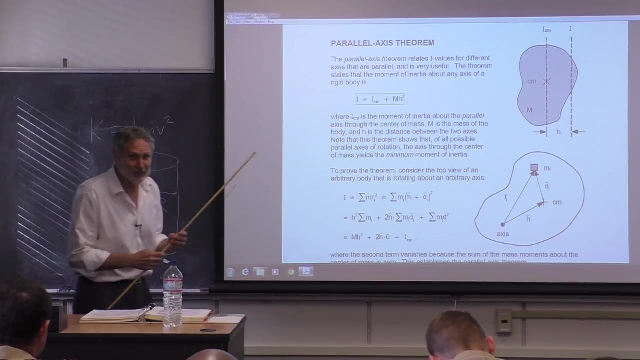 Okay, Some- whoever- I don't know what the history of this is, But I think the name is some instructor- got tired of students misusing it, So they said the students need to understand that this applies only to parallel axes. 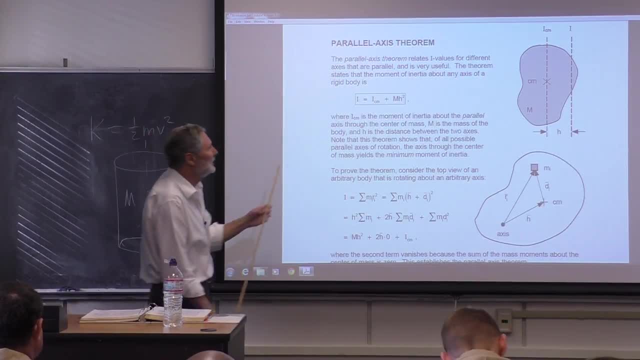 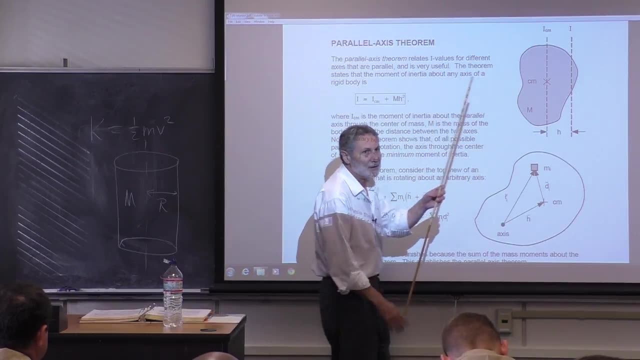 So that's probably why that's maybe what happened there. So here's the idea, Here's the theorem. It says the moment of inertia, you have a rigid body And you take any axis anywhere. Okay, Okay. 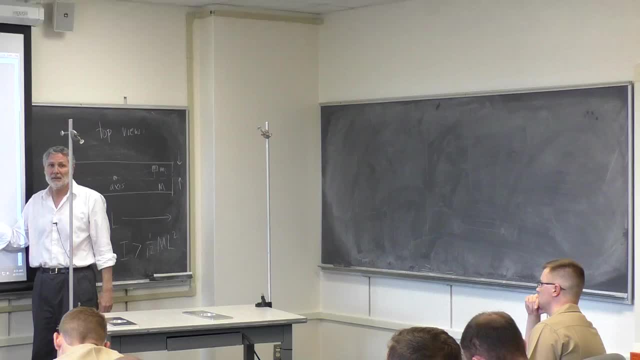 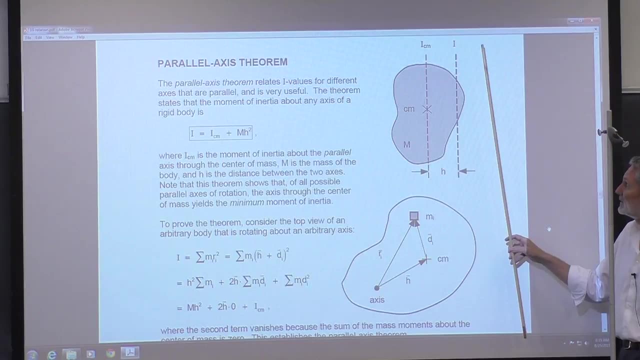 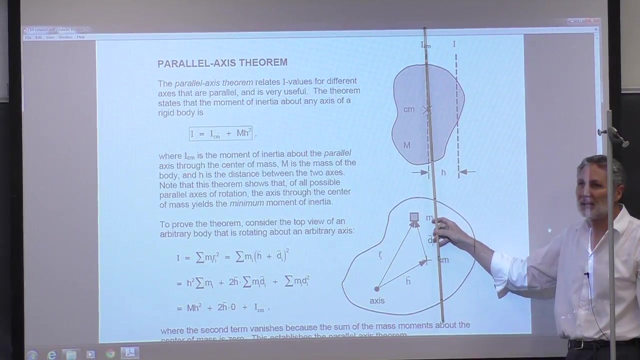 Is there anything wrong with taking an axis Over here? No, We just imagine we have some massless rods connecting this, So it can be anywhere. The parallel axis theorem relates the moment of inertia about any axis here To a parallel axis going through the center of mass. 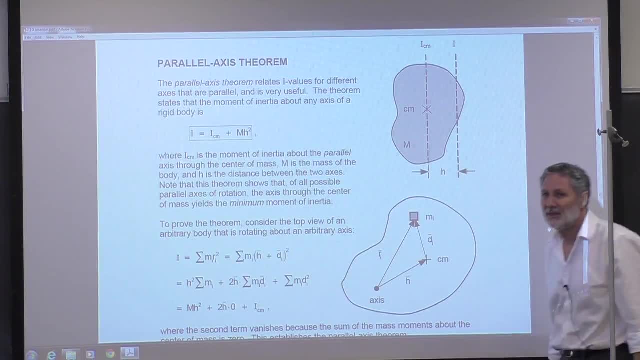 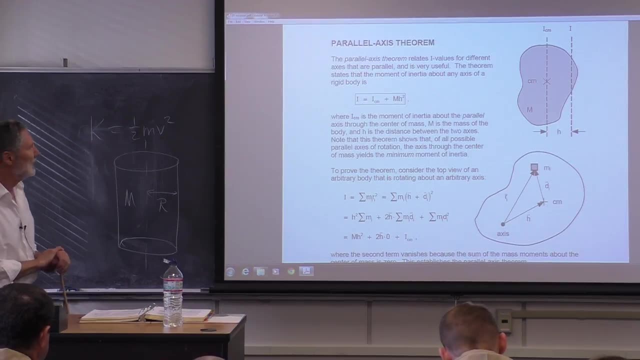 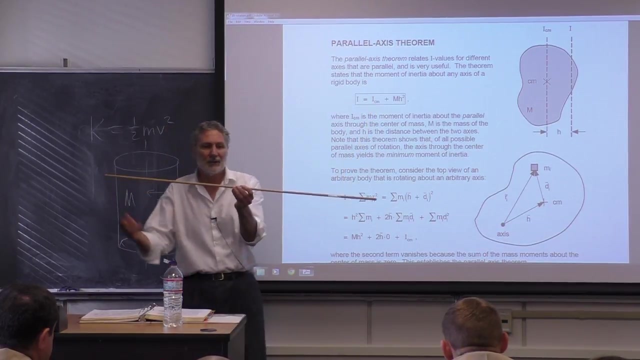 And here it is, And we're going to prove it In general For any rigid body, And it's an easy proof, As you'll see. I want to point something out first, though. Oh, So this is useful because, like the rod, the first thing we're going to apply this to is the rod. 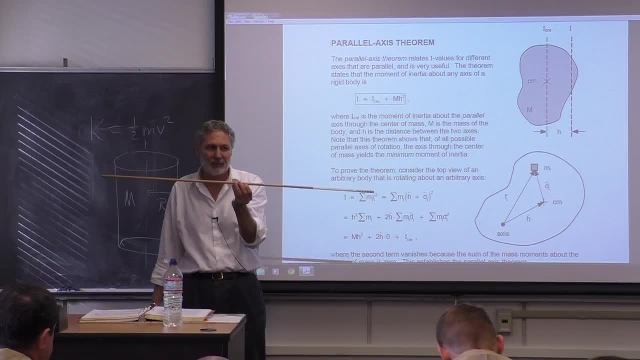 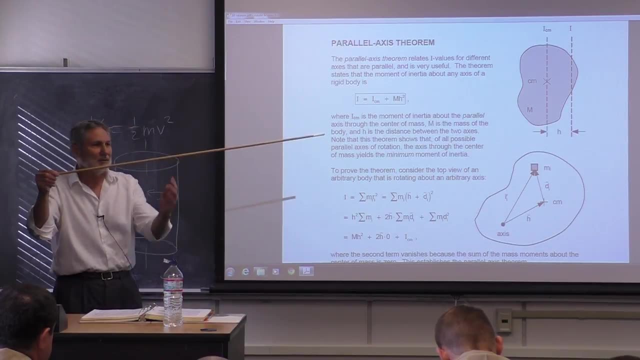 We calculated the moment of inertia about here, about the center right. It's 1 twelfth the mass times the square root of the length. What's the moment of inertia about here? That'll come up in a lot of problems. Well, if we know the moment of inertia here, we can get the moment of inertia about this parallel axis over here. 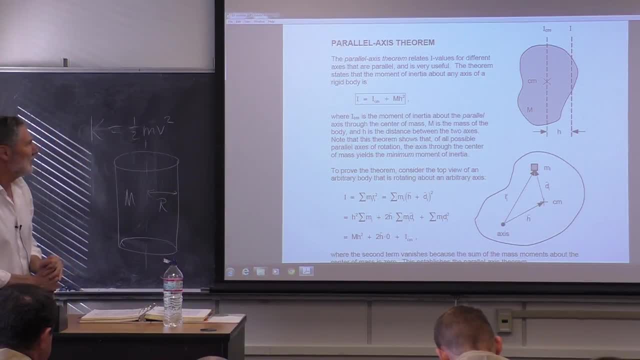 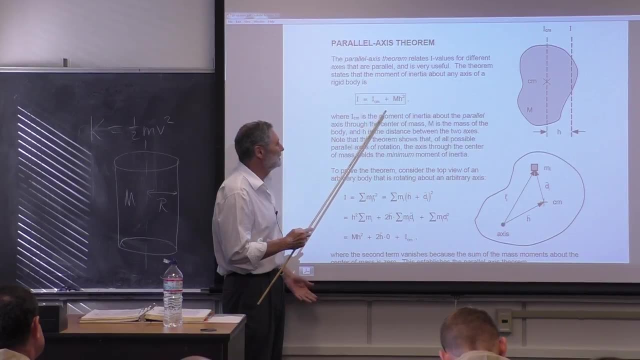 Right, So it's useful for that reason. It's also useful because it tells it's telling you something Here. Suppose you want to find an axis among all possible parallel axes, The axis that minimizes the moment of inertia. Where, which axis is going to minimize the moment of inertia? 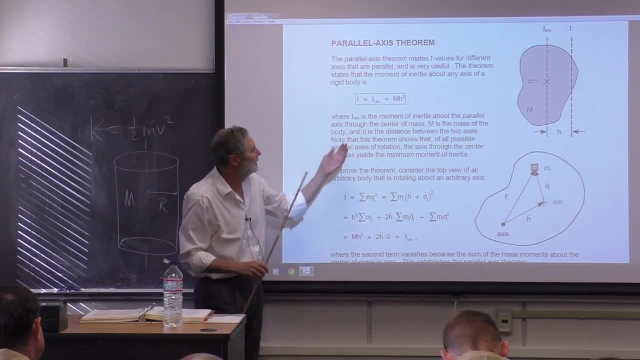 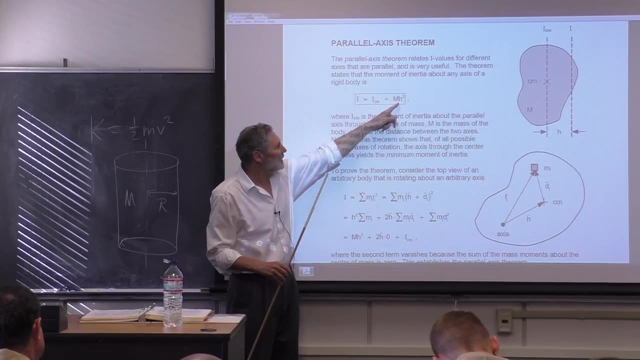 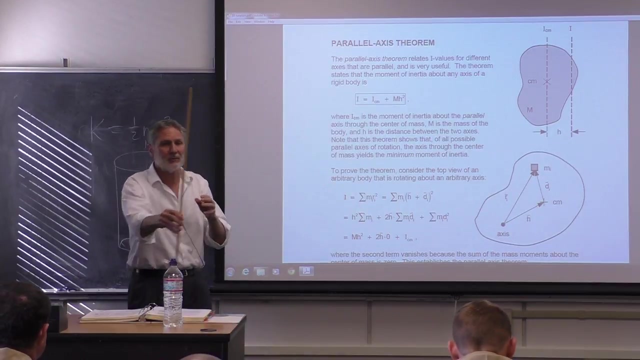 Of all, of a whole collection of parallel axes. How do I minimize this? Well, I take: h equals to zero. H is the distance between the two parallel axes. So, in other words, Of all possible, you have a bunch of parallel axes and you can find any, define any family you want, okay. 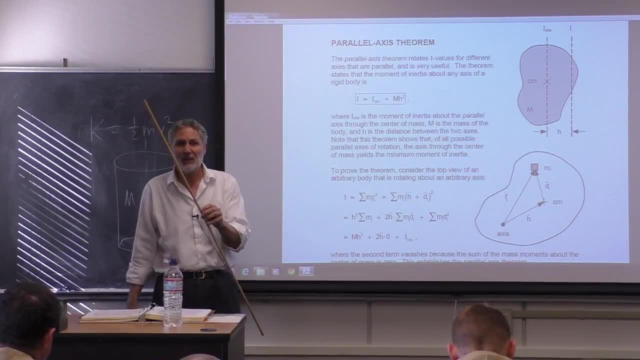 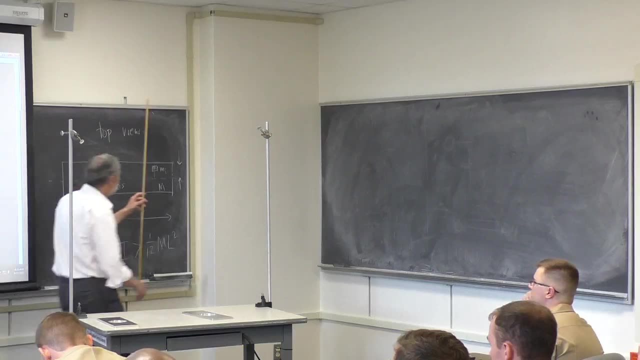 Just as long as they're all parallel, The axis that has the minimum moment of inertia is going to be the one through the center of mass, Which kind of makes sense. You know, the farther, if I get over here, I'm going to have a big moment of inertia, right? 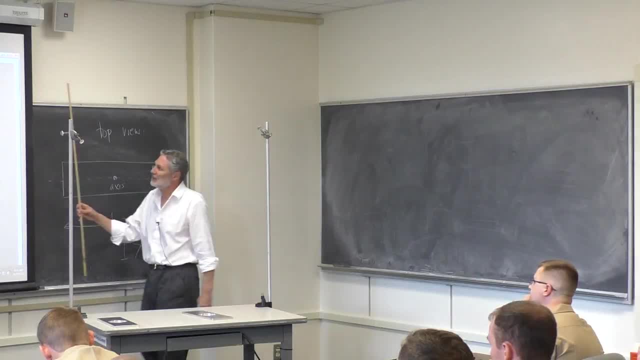 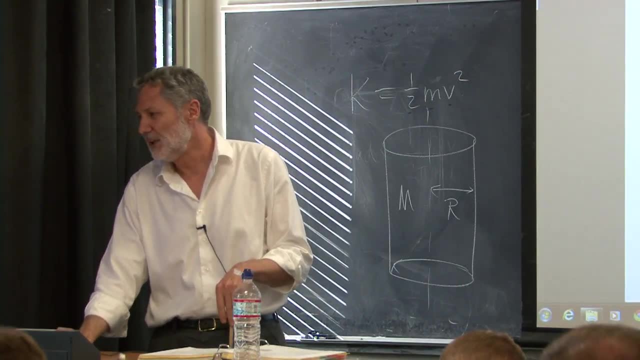 Because I've got a big distance here And the axis that minimizes it among all the parallel ones here is the one passing through the center of mass. So here's the proof. Now, This is probably going to look. this is analytical, okay. 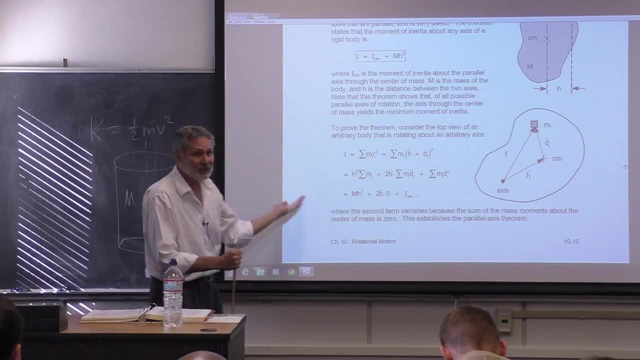 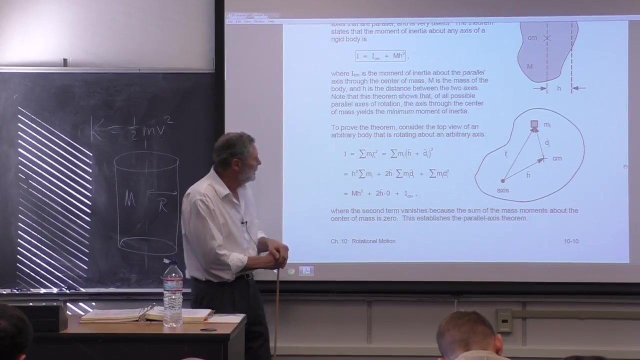 It. it's. the advantage of it is it applies to any rigid body, Alright, So we'll just use the summation notation. We'll use that. you know it applies to any it. you know it doesn't have to be a. this is true instantaneously. 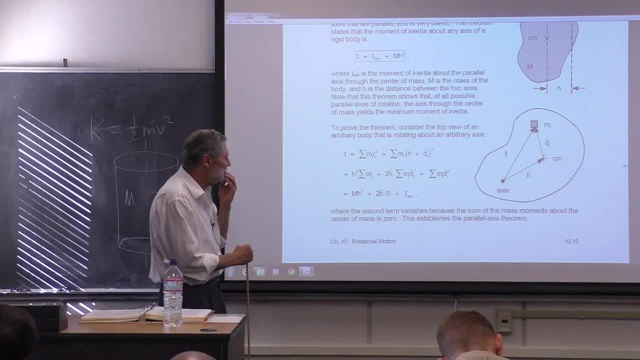 It doesn't have to be a rigid body, is that right? Well, the application is overwhelming for rigid bodies, But I think it's more general than that. It's like any system of particles. Okay, so here's the definition of the moment of inertia. 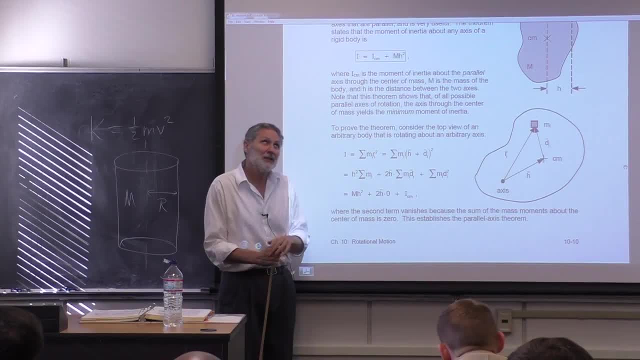 Which we derive for a rigid body. So I guess I have to say, yeah, the usefulness of this is for rigid bodies, Because this is the moment of inertia for a rigid body, Everything has to be locked in place. Remember, v is equal to omega r. 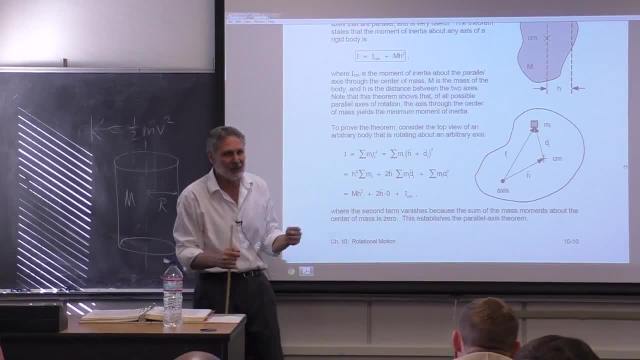 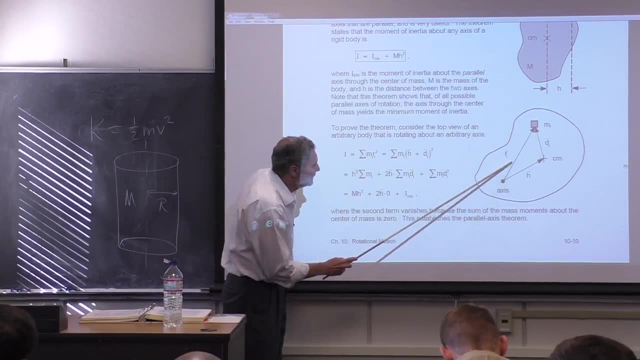 If you've got things going their own merry ways, it's not, it's going to be meaningless, It's not going to be useful. Okay, So here it is Now. the trick here is: this is the relevant distance for this little mi here. 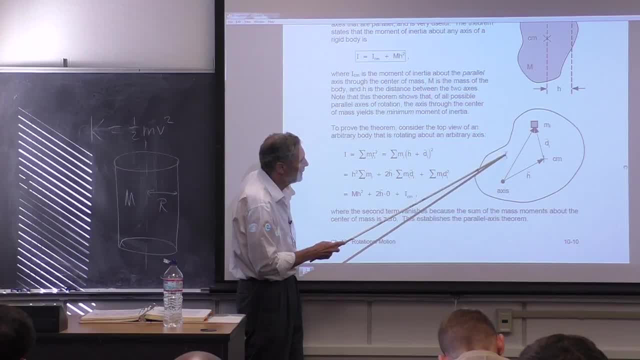 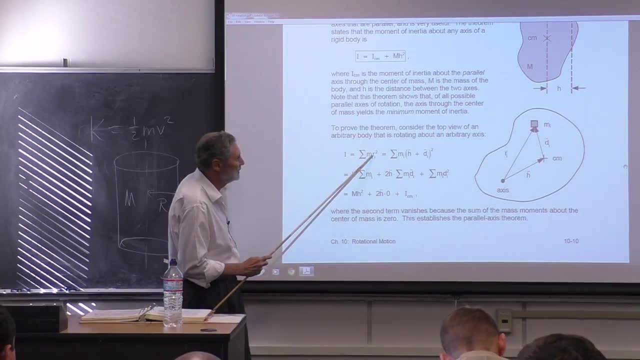 We want to represent it as a vector. sum Each little ri here, this vector as this vector to the center of mass plus this one. That's the trick here. So we get rid of our vector in terms of h and i. 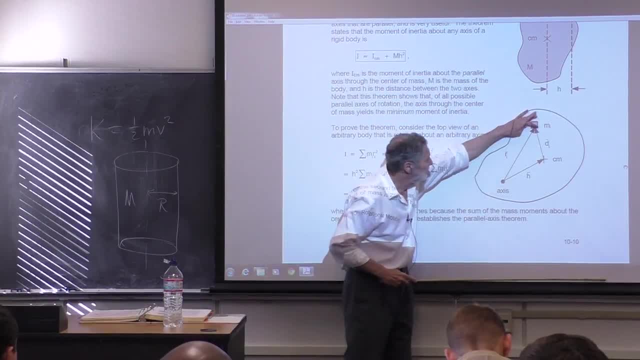 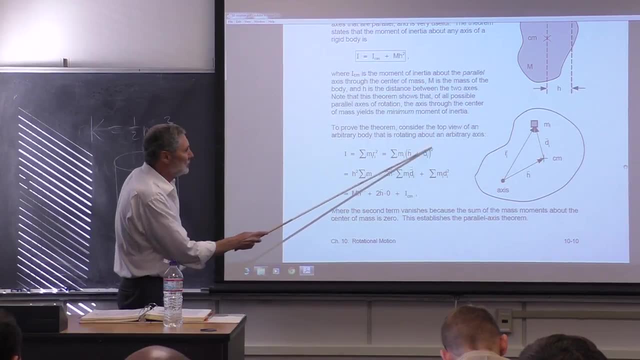 Now h. here is just some. it doesn't depend upon what the mass element, It's just this fixed vector here, From our axis to the center of mass. Now you can square this and you get three terms. You get the h squared term first of all. 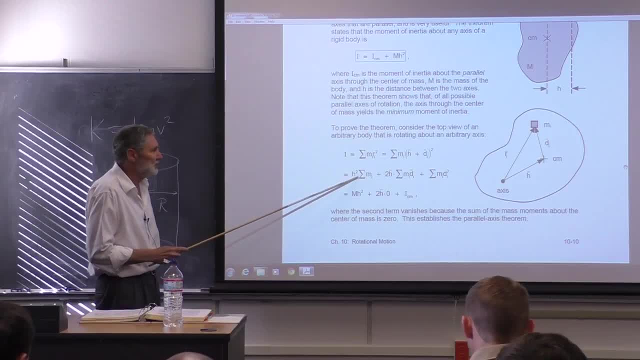 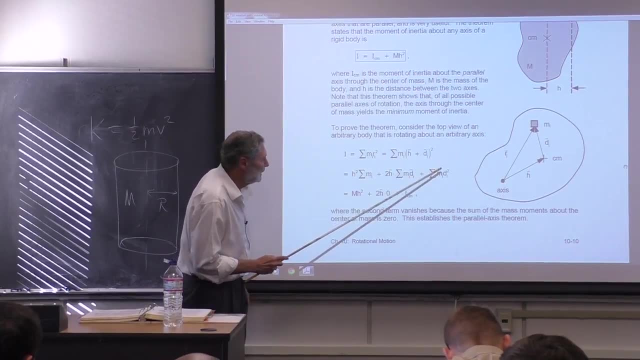 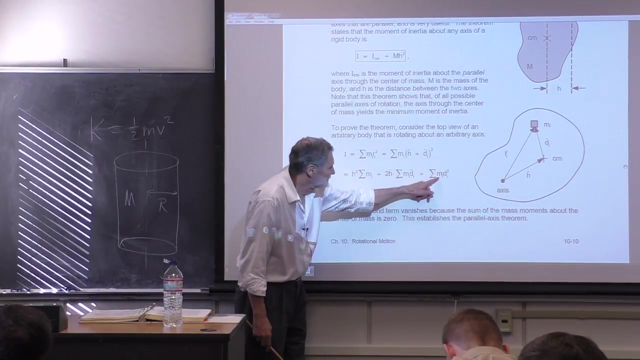 Because that's constant, it comes outside the sum And we just have the total mass times h squared. The third term, similarly, is the mass times d? i squared. We can't take d? i out Because it depends, okay, on i. 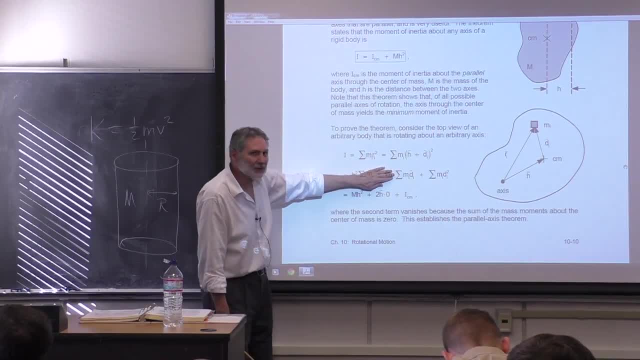 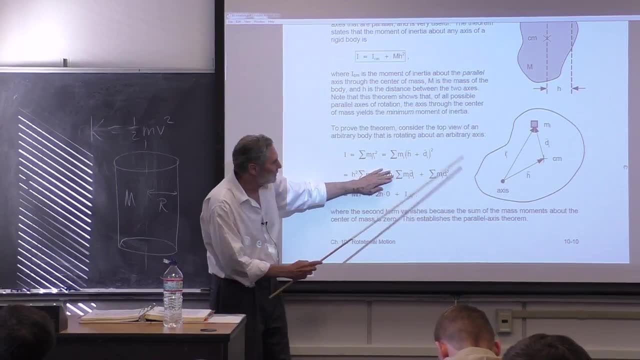 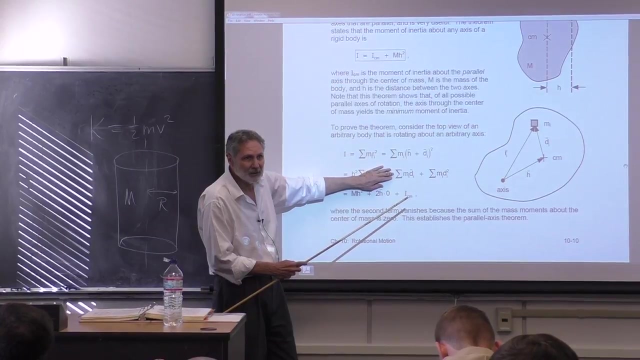 What about this middle term here? Does this look familiar? This is the sum of the moments of all the masses about the center of mass. So remember what this equals to. The sum of the moments is the total mass times, the vector to the center of mass. 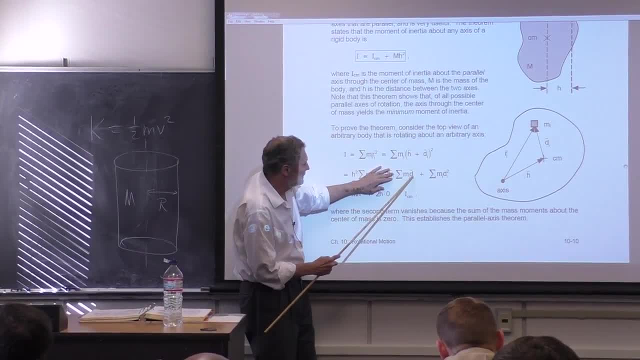 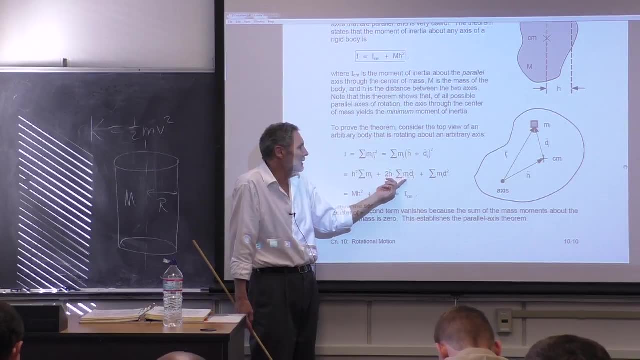 So if I'm at the center of mass, because this d is in the frame of reference where our origin is the center of mass, This has to be. this specifies the balance. This is the balance point. So this sum has to, the sum of the moments has to be zero. 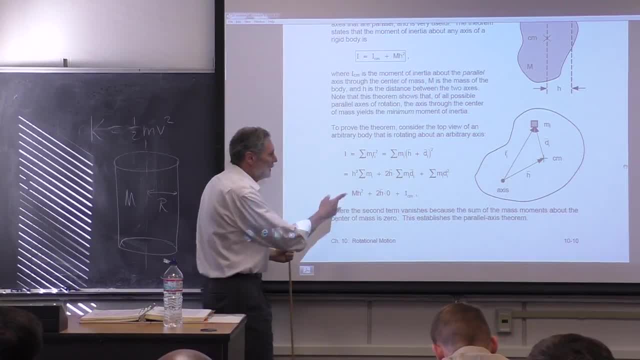 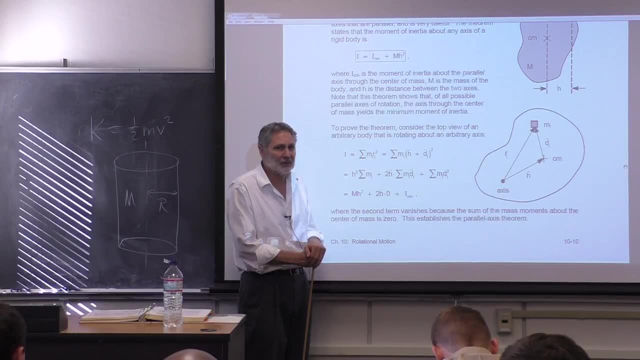 It's got to be zero when you have the center of mass here, Because we have a theorem that says that the sum of the moments is the total mass times the r vector to the center of mass. And if we're at the center of mass that r vector is zero. 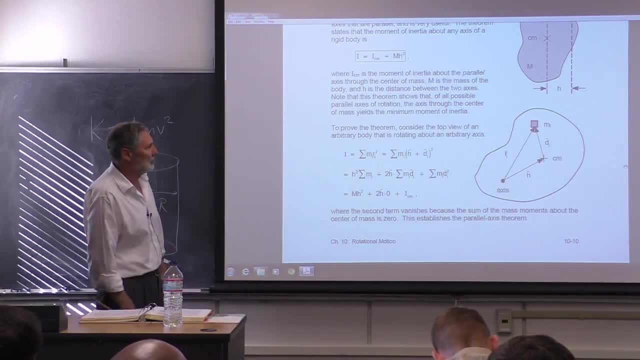 So this term goes away, We get this, and then we just prove the theorem. I'll move these around a little bit. Right, You just have to move this over here and you get this. So it's actually easy to prove in general. 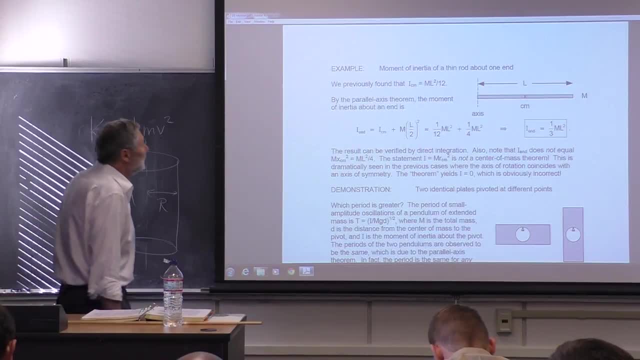 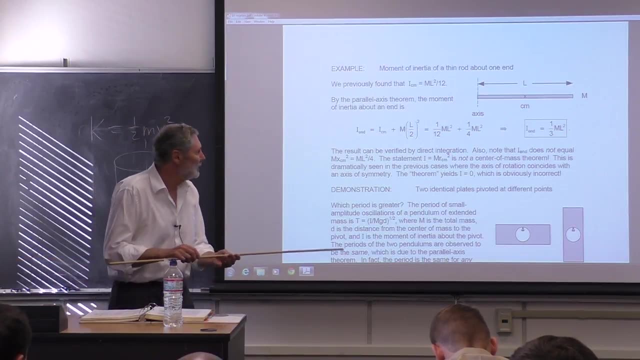 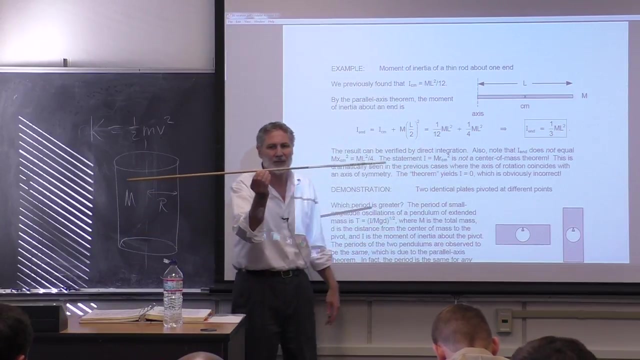 So here's- we're going to look at a couple of applications of this. Here's as promised. here's the rod. okay, And most people, somewhat including me, don't remember this: 1 twelfths m l squared. 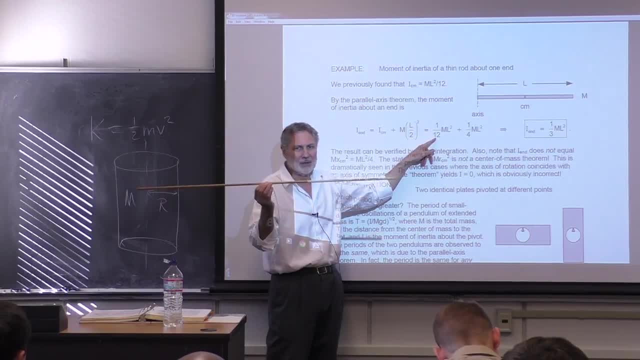 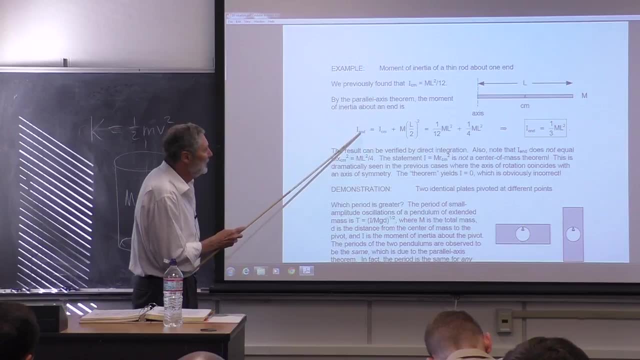 Because this is like a you know weird thing. It's a weird number 12.. However, if we ask what the moment of inertia is about the axis, about the end, and we use the parallel axis theorem, I about the end, is I center of mass plus the total mass times the distance to the center of mass. 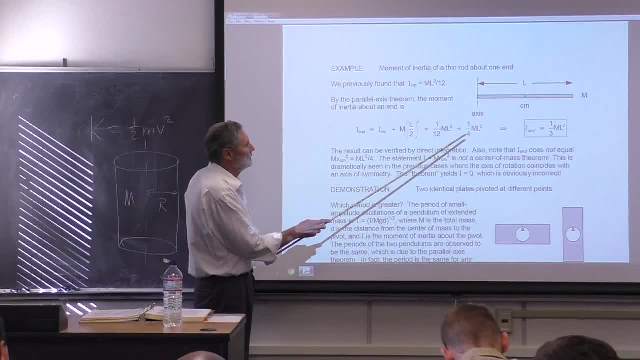 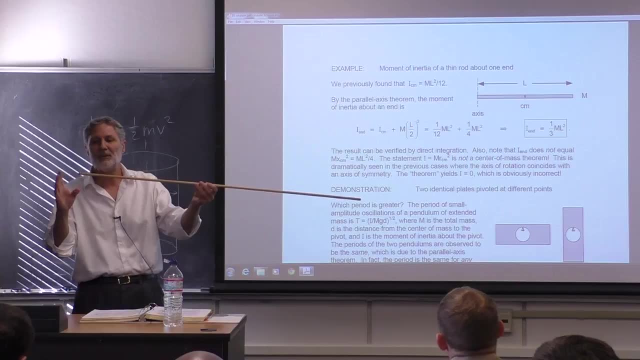 which is l over 2.. What's 1 twelfths plus 1 fourths? It happens to be 1 third. So this is what people usually remember for the moment of inertia. They remember the moment of inertia about the end of a rod. 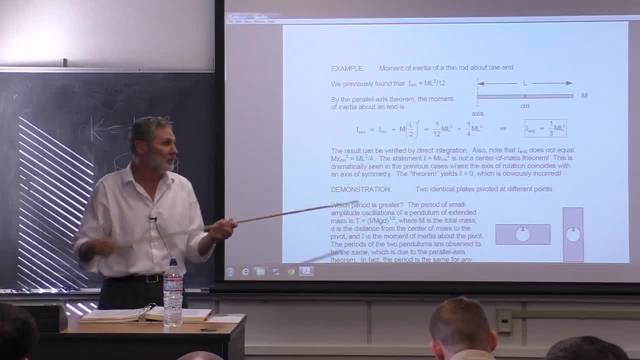 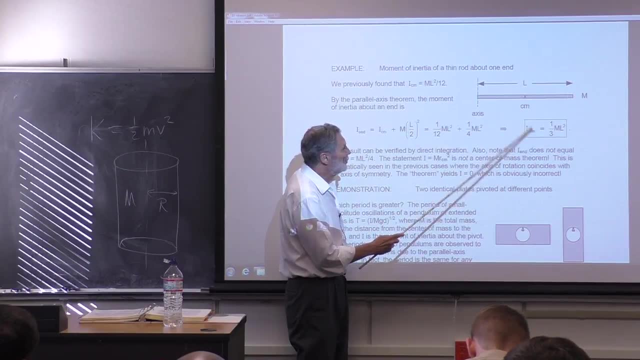 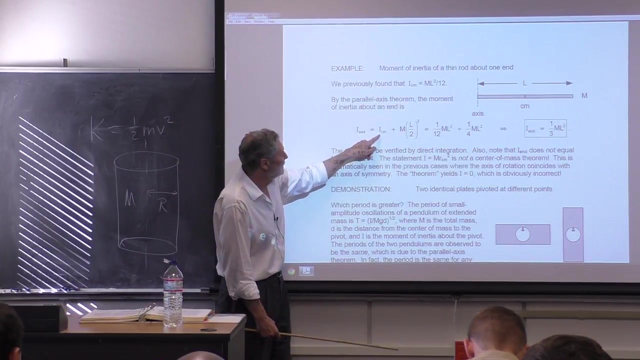 And that's often, you know, in applications, that often comes up. So usually people, including me, memorize this just naturally. If you want to find the moment of inertia about the center of mass, what do you do? Well, you, just you, you. 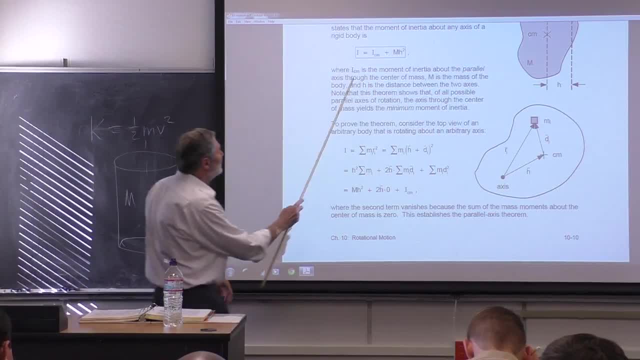 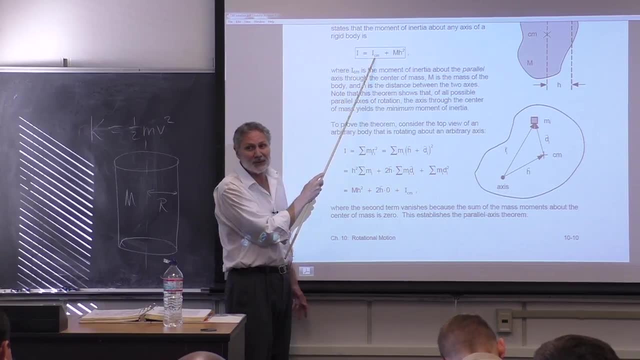 if we know the moment of inertia. see, this tells us what the moment of inertia is. if we know it's the center of mass. If we know this about some axis, then we can find the moment of inertia about the center of mass. right. 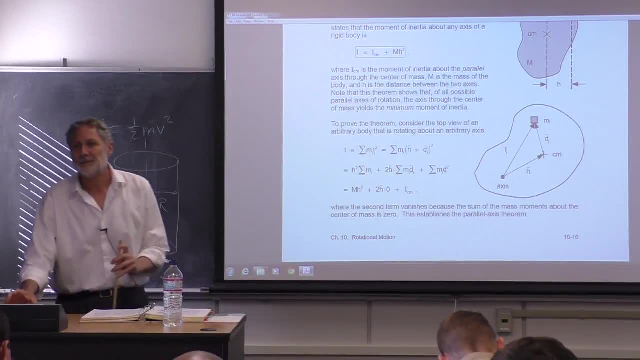 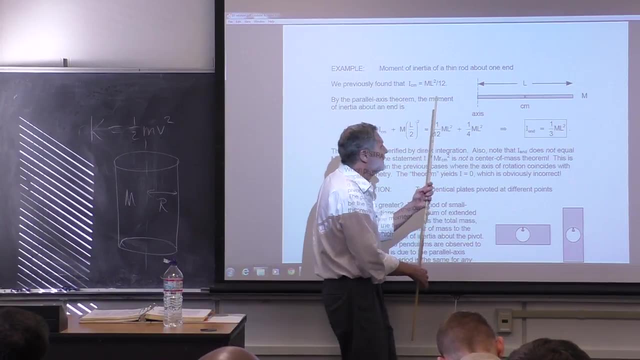 It's just algebra. They call that algebra So we can look at it from. you know, turn the tables on us, look at it two different ways. So most people remember this is 1, third and then, if they need it here, 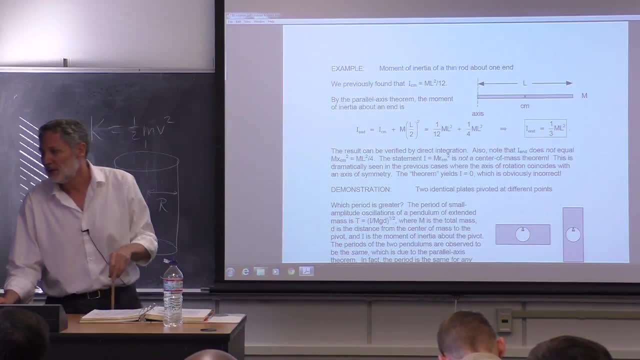 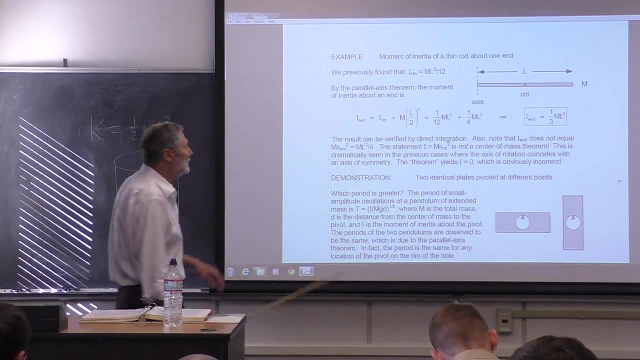 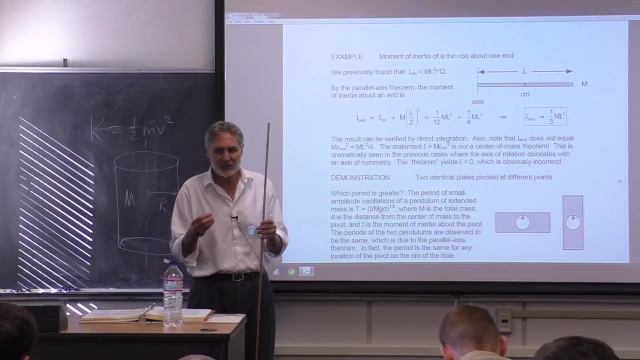 they can derive. use the parallel axis theorem to get it. Now just a little word of warning here. Obviously, if I have an object, it's going to have a center of mass. So if I want to find the moment of inertia, 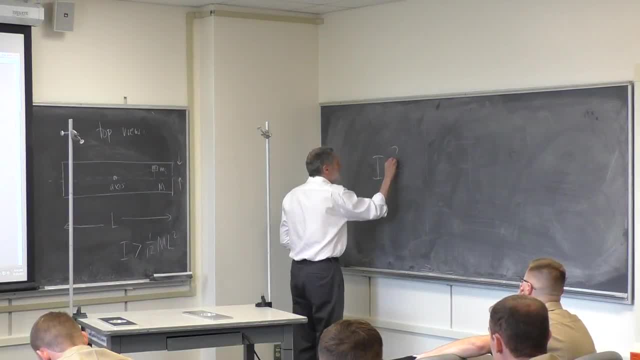 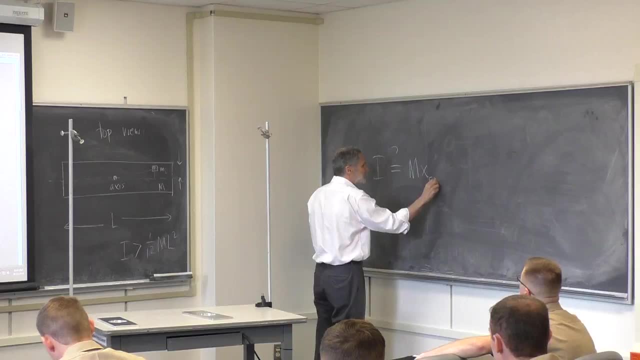 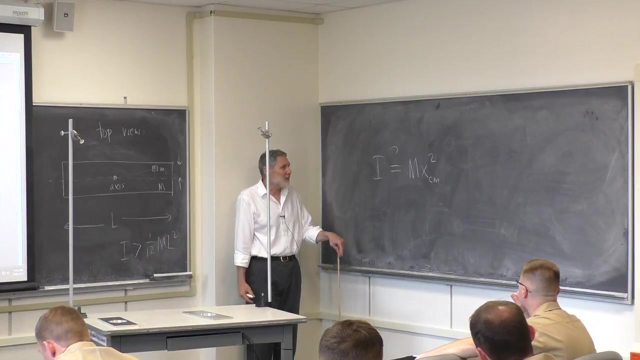 shouldn't I just take its total mass times, its distance to the center of mass? let's call it x here squared, We have all these center of mass formulas, right? This sounds like. this sounds good. The total moment of inertia of a body. 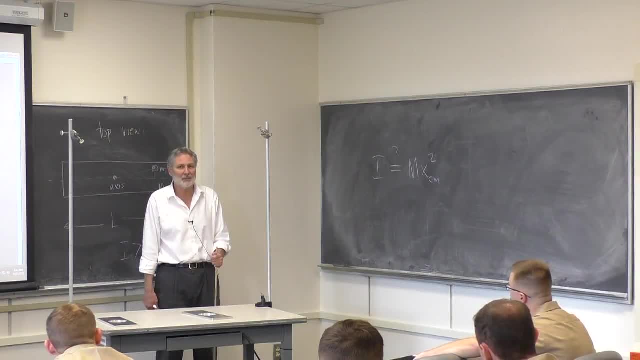 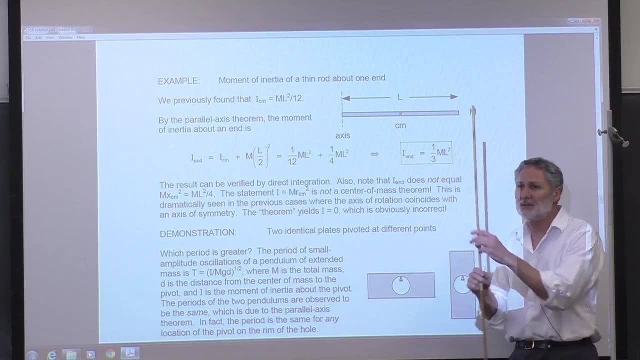 is the same. if you imagine its mass to be concentrated at the center of mass, It's bullshit. It's not right, is it? What? what? take a look at this. Look at the center. the center, this, this. 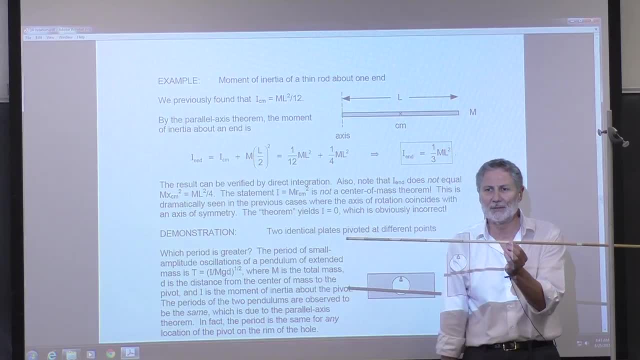 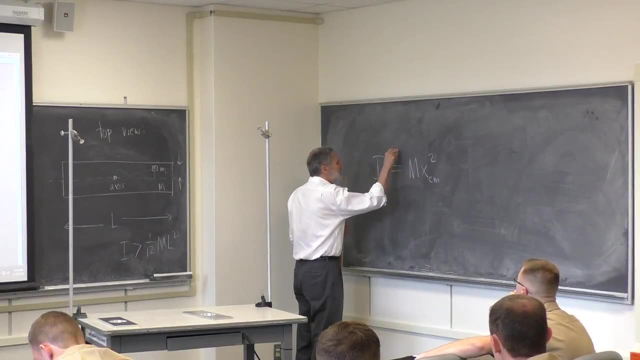 It has a moment of inertia. If I imagine all the mass to be concentrated at the center of mass, what you get? zero right. So this is this is not true. It's one of those. you know, you've got to be careful. 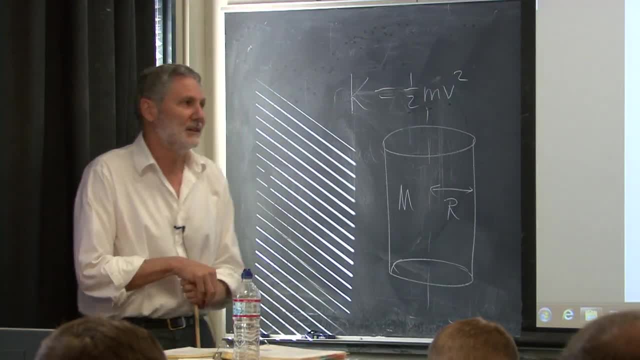 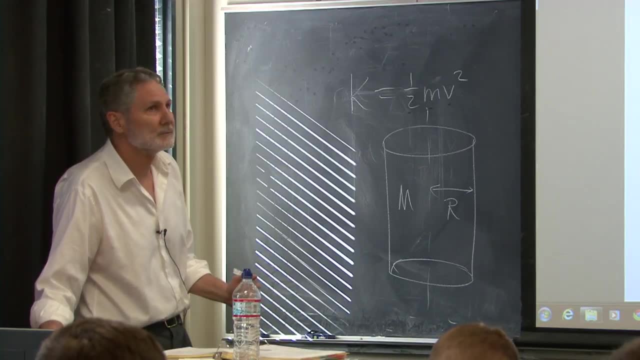 even though the center of mass has a lot of properties And it sounds good, The center of mass is the same. if you imagine it's not right, it's obviously not true. So it's just a little word of warning there. 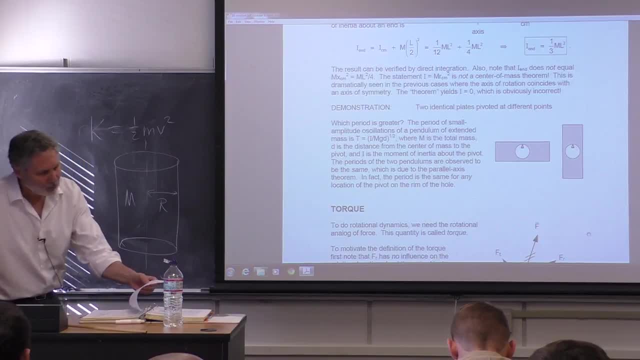 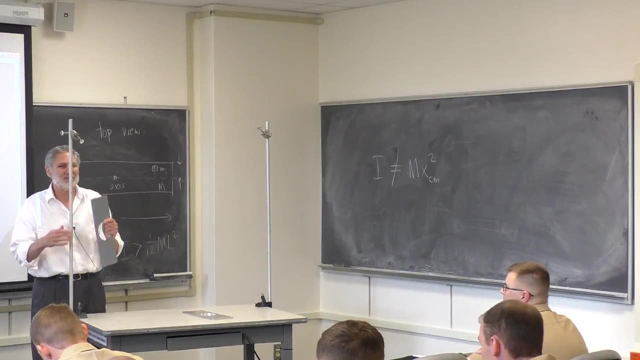 Okay, so what we? there's a demo here, okay, And it involves oscillatory motion, something we're not going to be able to do in this class, But it's still worthwhile to see this demo, I think. So this object. 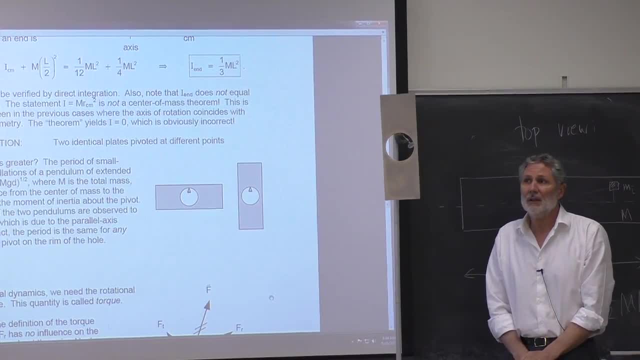 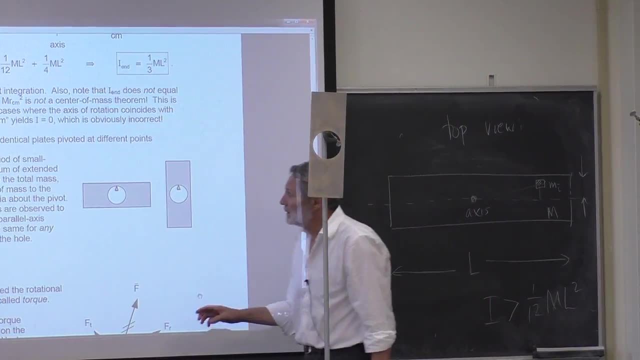 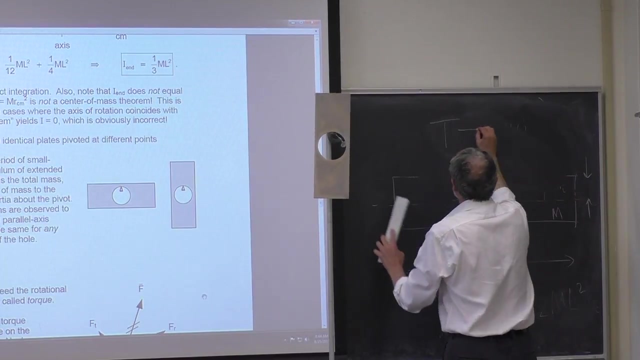 this is a kind of pendulum. It has a frequency there or a period: the time for one cycle Right And the. what we don't have time to derive is the fact that the period here is given by it's in the notes there. 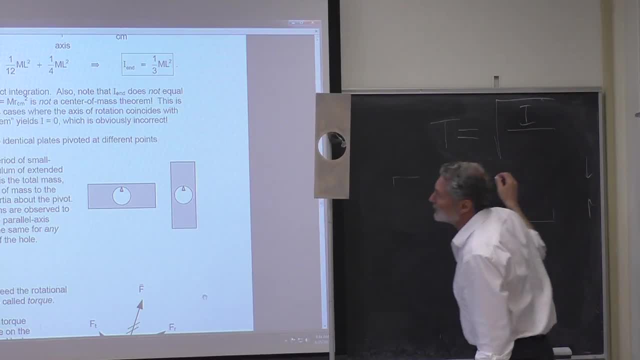 the square root of the moment of inertia. times the divided by the total mass, times g times the distance to the center of mass. Okay, So this has some total mass. It's what's the distance to the center of mass? 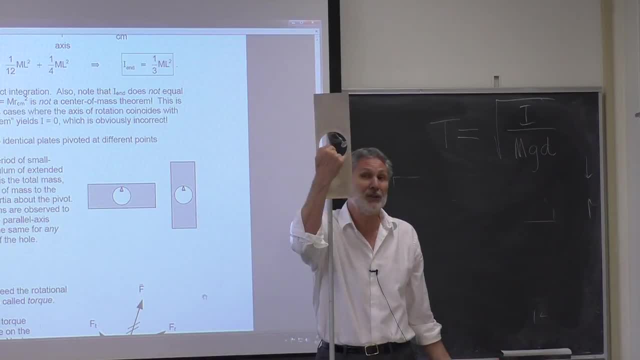 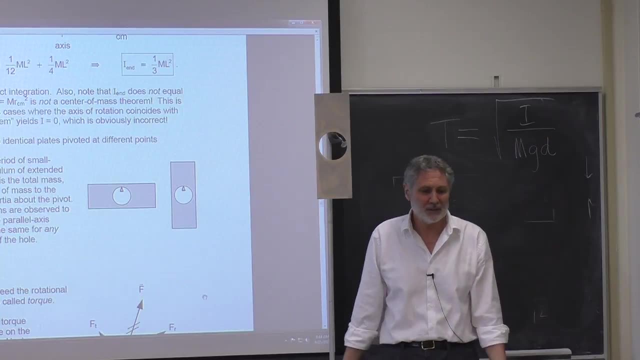 Where's the center of mass Right in the center geometric center here, And it's got some moment of inertia about that axis And you can calculate it. but we're not going to do that. But the point of this demo is: 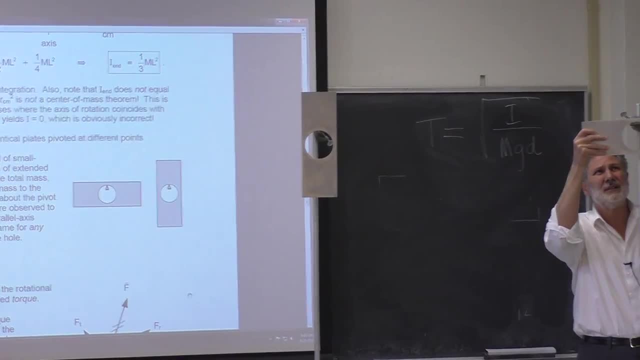 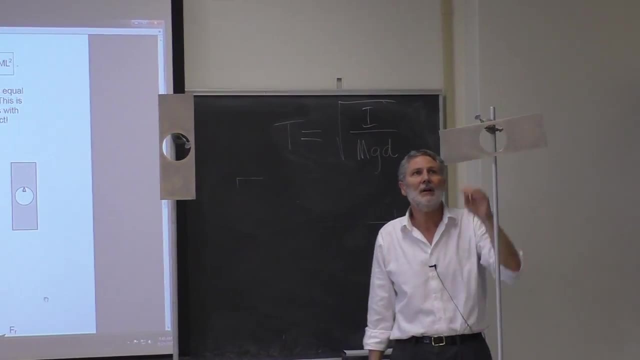 I've got an identical plate here, but I'm going to put it at 90 degrees. Okay, this is also a pendulum. What's what should be the? how do those periods? which period's going to be bigger? Any guesses? 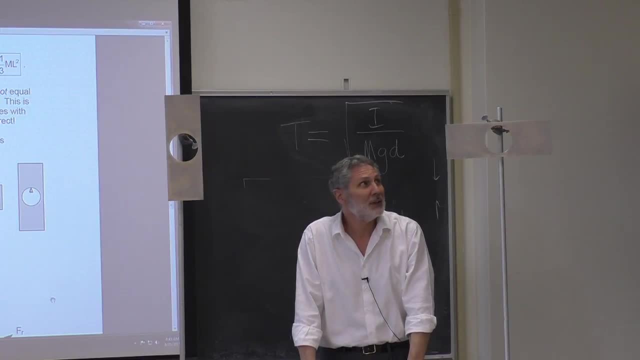 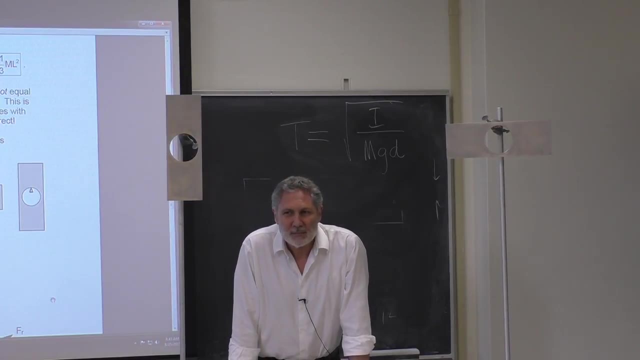 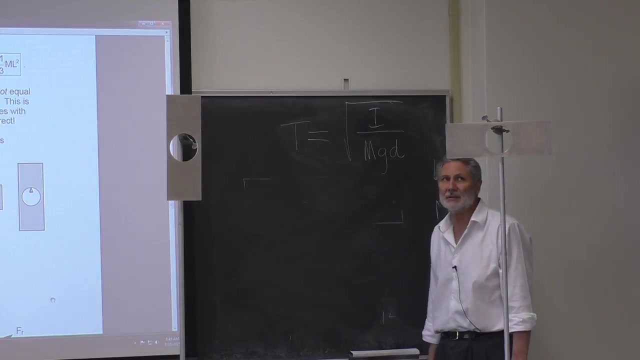 I heard something: They've got to be the same, they have to be the same. Why are they the same? Because the mass is the same. Oh, the moment of inertia depends upon the distance to the center of mass. Okay, The distribution of the mass. 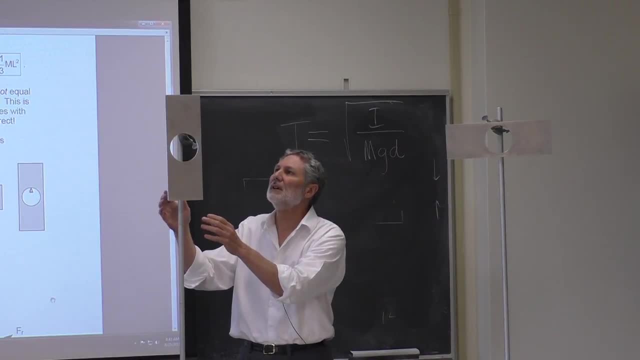 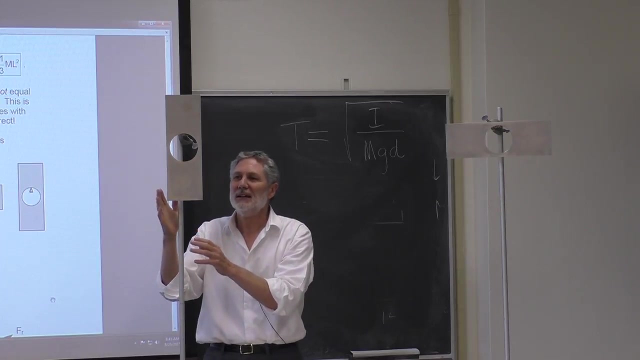 So I see whoa this thing's. this is called a librator Right. That's important for the Tacoma Narrows Bridge Collapse. I keep working on that when I get a chance. So it looks like the distribution of the mass. 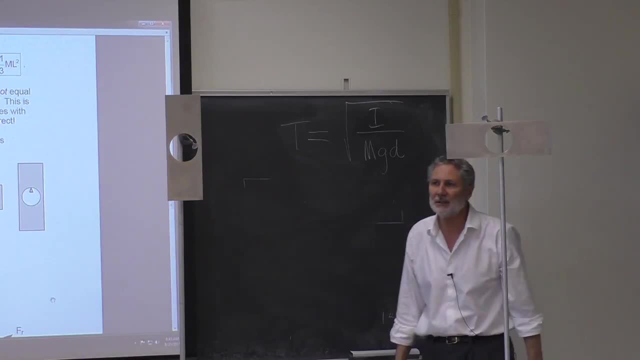 about this? it looks like they're going to be different moments of inertia. However, what does the parallel axis theorem tell us? Okay, The masses are the same. What about the distances to the center of mass? Same, But it looks like the moments of inertia. 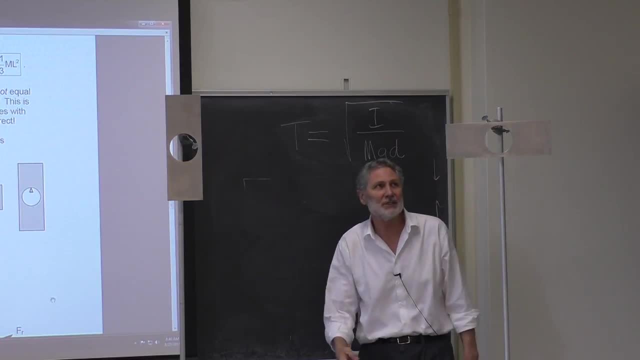 are going to be different. However, the parallel axis theorem tells us that the moment of inertia about here is the moment of inertia about the center plus the total mass times the square of that distance. So what do I get? over here, The same. 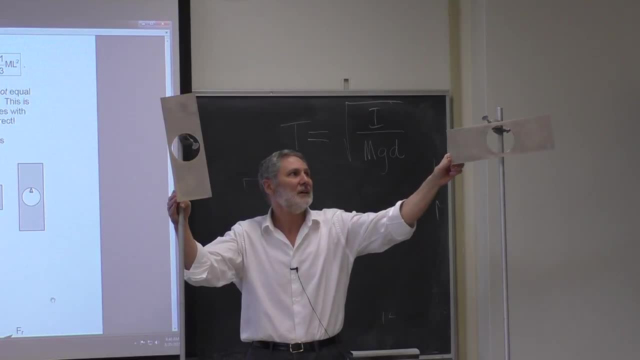 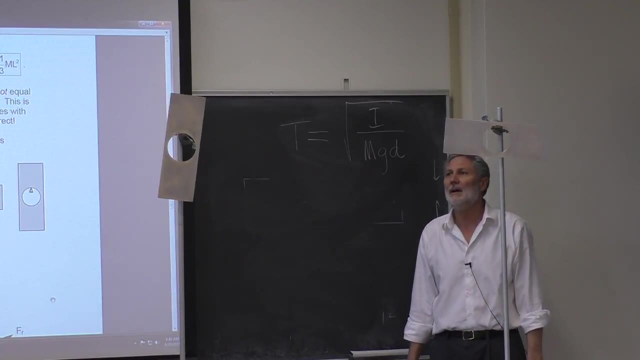 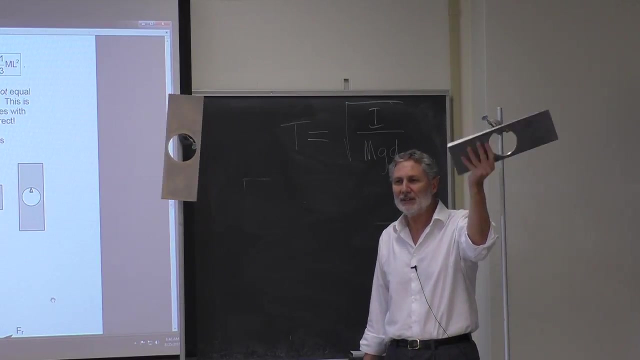 So these should have the same period. So let me see if I can do that here. I'm going to try to release them from rest. Okay, A little bit of phase there. You see they're the same. So this is actually. 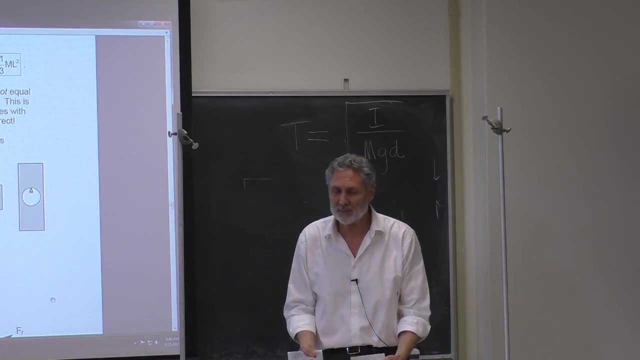 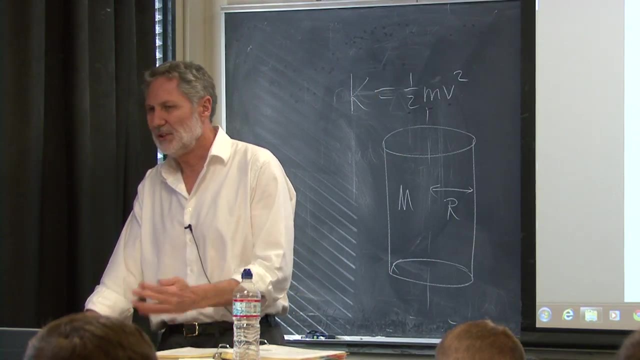 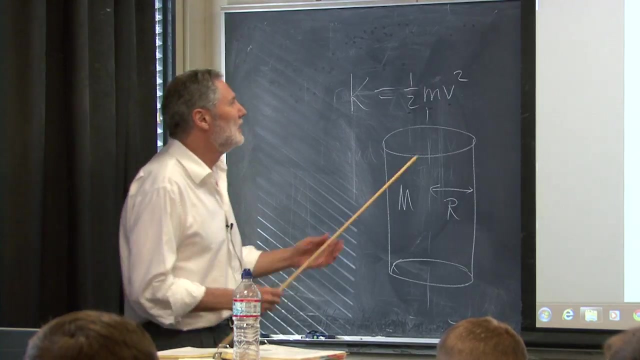 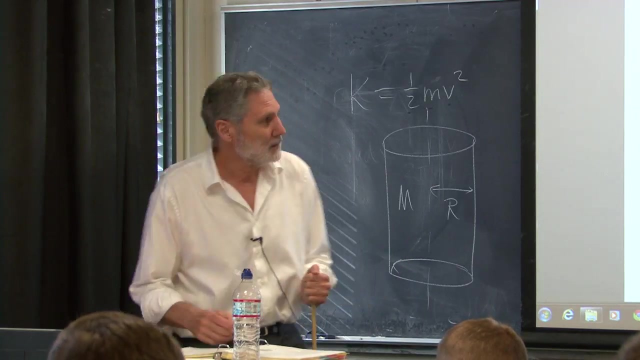 you can think of this as a demonstration of the parallel axis theorem. Somebody published that, believe it or not, In an educational journal. I know because I was the one who published it. Okay, All right, Short, Short article. I looked into that. 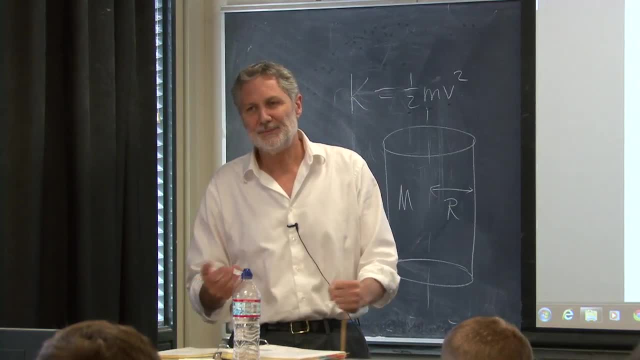 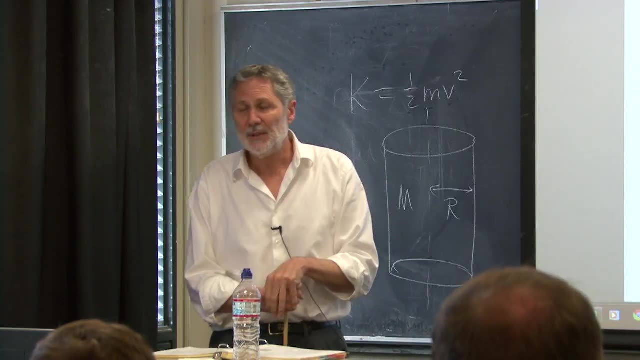 because I wanted to see. There are some really, you know it got murky. So this thing about the monkey hunter, I checked into that. It's very short But you'll find really short things. There are a lot of times just notes. 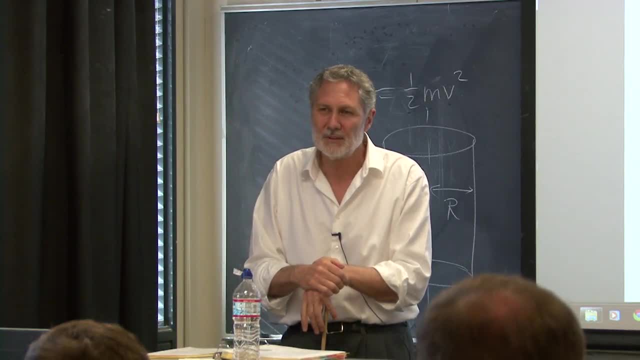 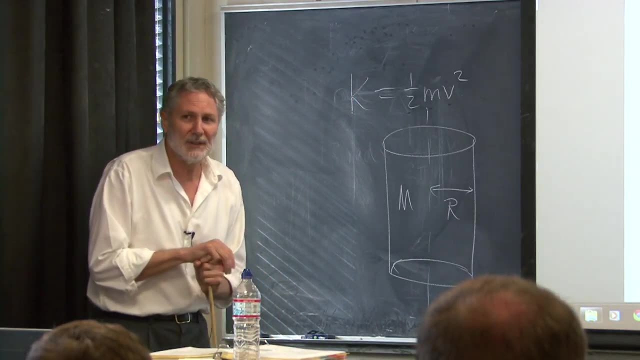 that somebody wrote about some other paper, So I couldn't really claim it, So I dropped it. I usually follow up on these things, Yeah, So So forget the Guinness Book of World. Records. That's going to All right, So. 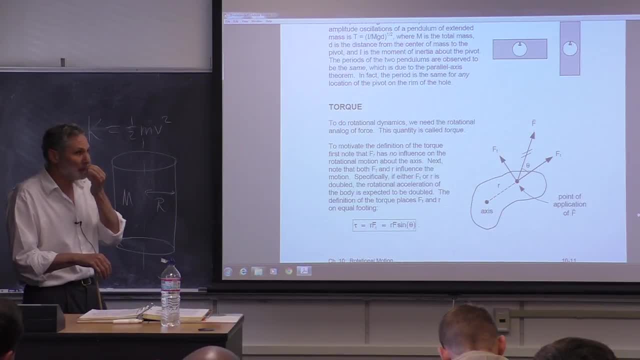 To set. We're setting the stage for dynamics. We've got to do one more thing here before we get into it, And that's to deal with torque. Torque- You've all heard of that, And it's the rotational analog of force. 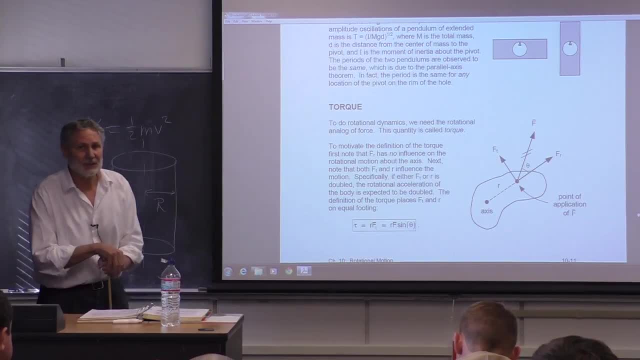 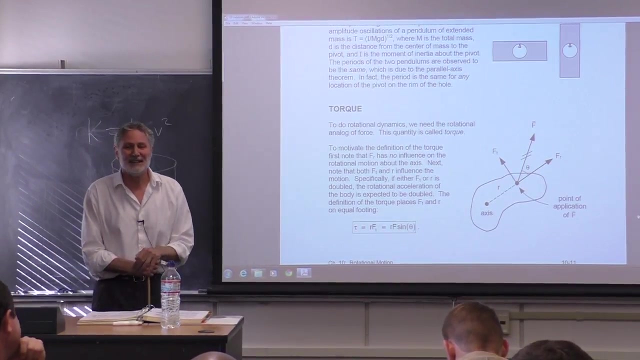 We're headed towards an. F equals MA, type description And instead of M, what are we going to have? Take a wild guess: Moment of inertia. Right, And instead of A: anybody, Omega, Alpha, Right, D, omega, DT. 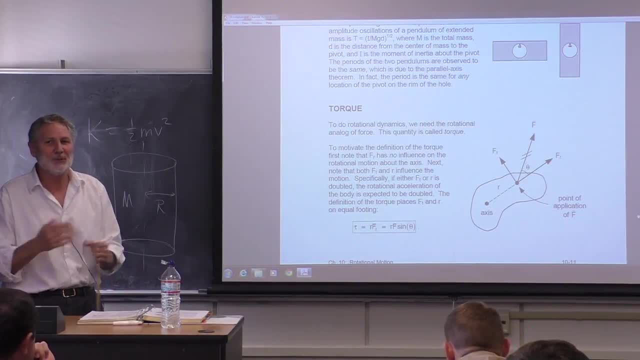 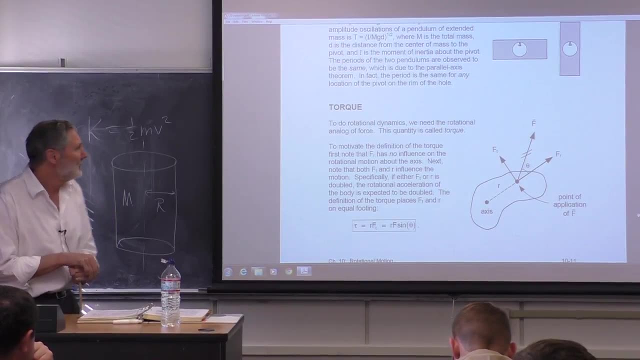 So we're headed towards. And so what's the analog of force? Well, that's what: torque. So we're headed towards. torque is equal to the moment of inertia, times the angular acceleration, which is D, omega, DT. That's where we're headed. 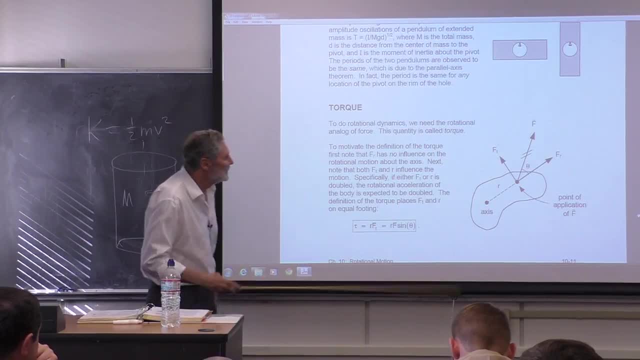 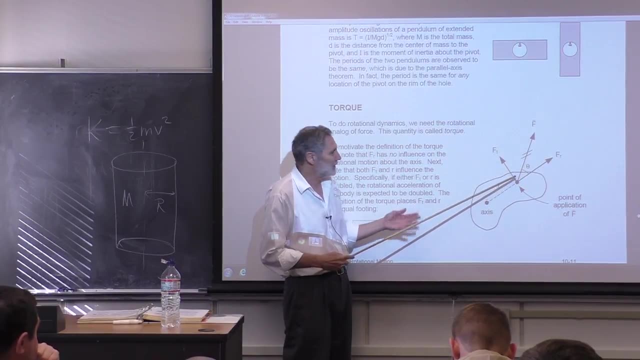 Okay, So we're going to talk about torque now. So here's a fixed axis of rotation, Here's a body, A force. An arbitrary force is applied at some arbitrary point off axis here. So this is a force. here We can resolve the force into two components. 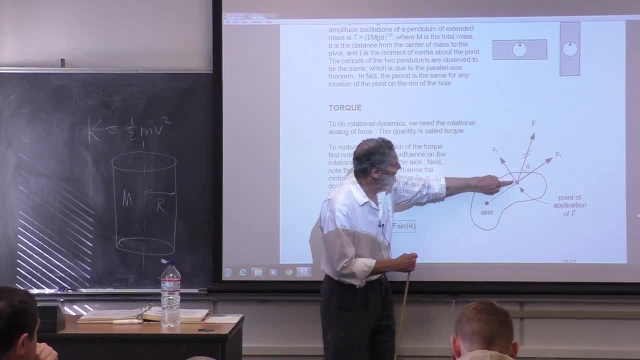 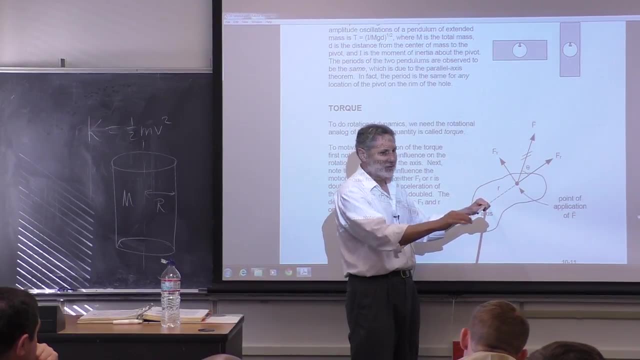 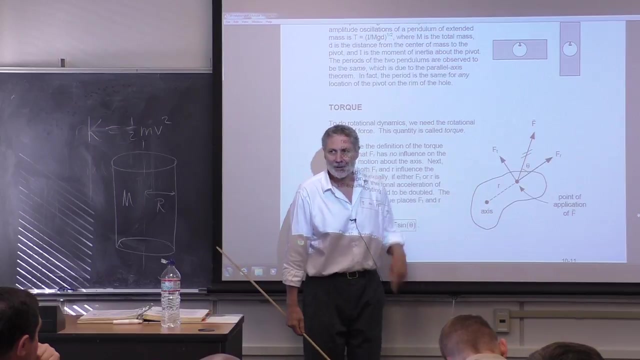 A radial component and a tangential component. What's? Somebody has fixed it. It's making sure this axis is not moving. Okay, It's attached to some bearings. It's attached to the earth, Okay. What influence does FR have on the rotational motion? 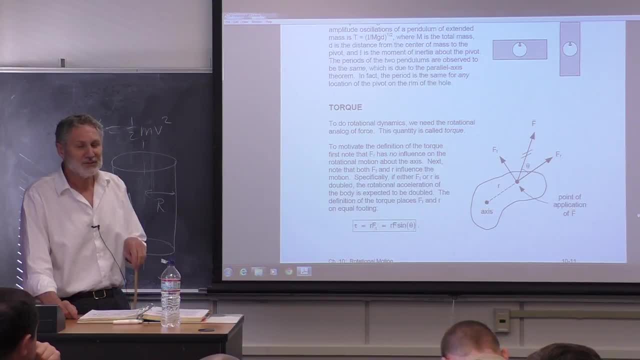 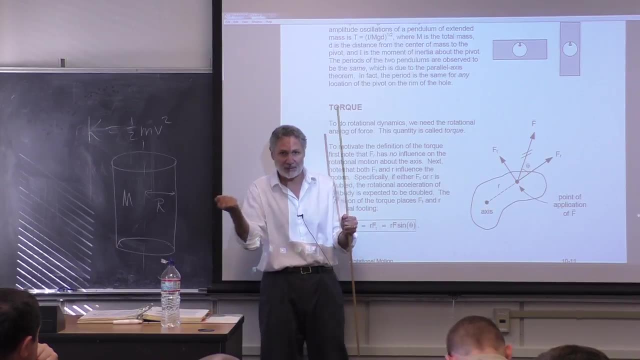 I'm looking for. one word here Starts with Z, Zero, Zero. This is not going to influence the rotational motion. You know you have an object like this, You exert a force like this, Nothing's going to happen. Something has to prevent. 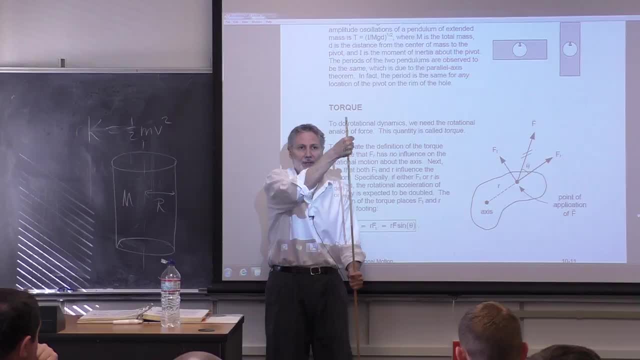 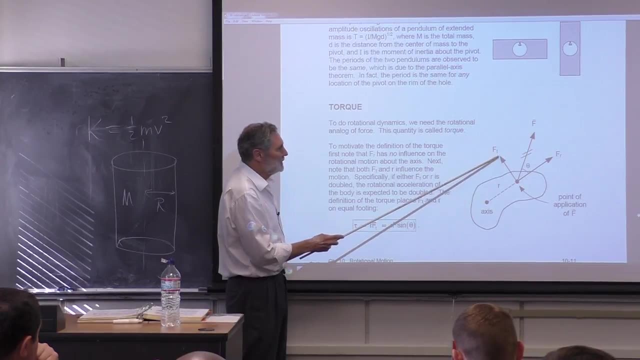 You know it's going to be balanced by whatever this axle here, Whatever it's rooted in, Okay, Whatever it's anchored to. So this is irrelevant. That's interesting. What's important is the tangential part, But that's not only what's important. 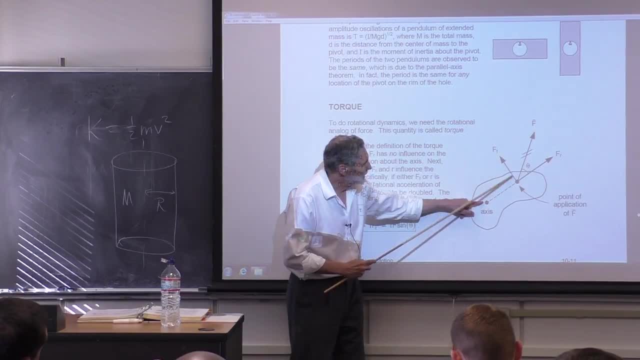 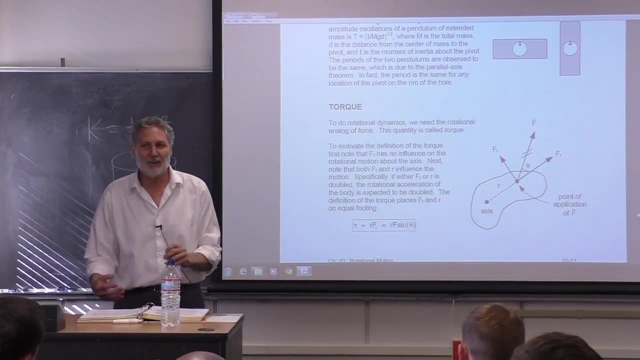 See this distance here. What if I applied this tangential force but I doubled the distance? What's going to happen to the angular acceleration? And you've all experienced something like this- It's going to increase. It's going to, in fact, double. 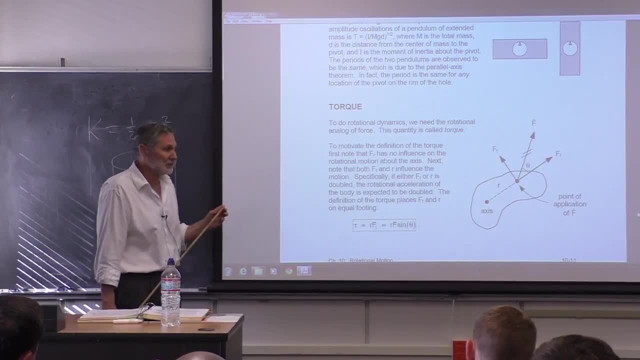 Okay. So our definition of the appropriate definition here And the only reason it's known to be appropriate, because people played around with it and looked back and say, okay, that's what you know. in retrospect, looking back, this is what you want to define it as. 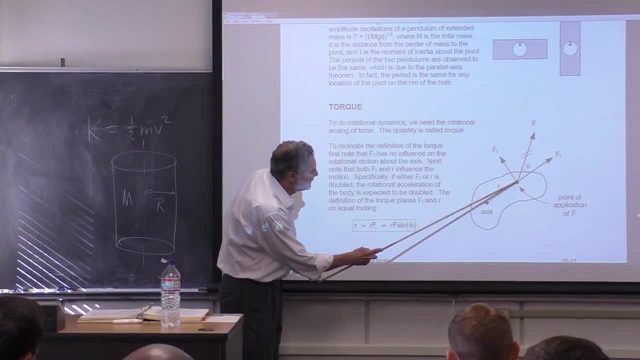 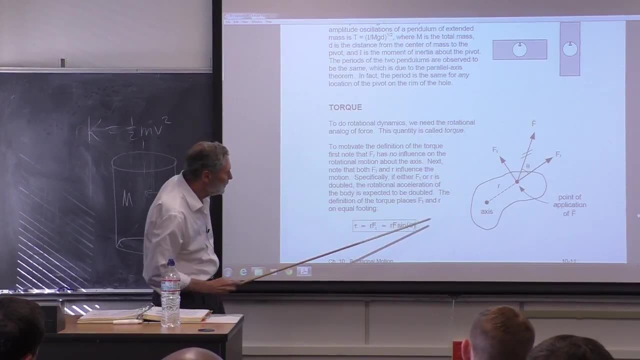 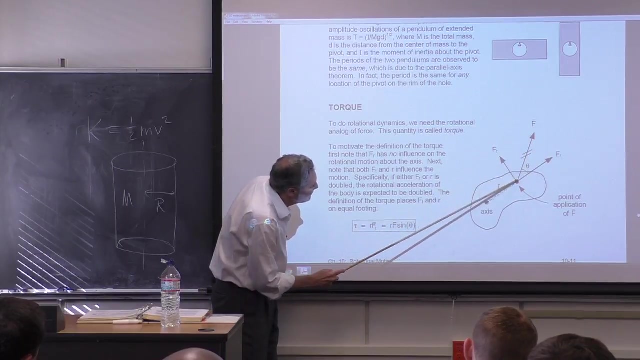 The torque is the tangential component times that distance right there. That's the torque. We can put it in terms of the total force if we multiply by the sine of theta, because the tangential component here this is the same as that And you can see that it's F times the sine of theta. 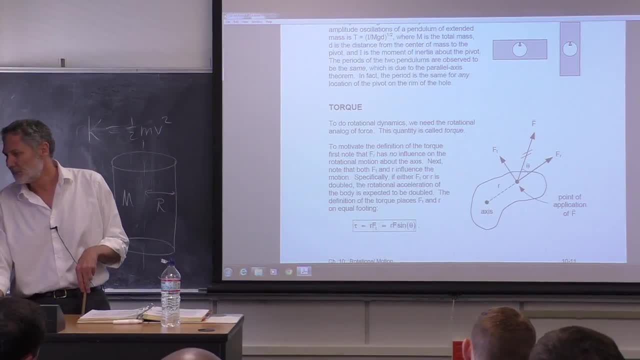 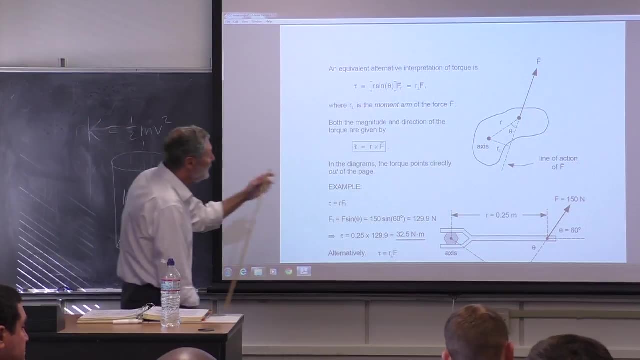 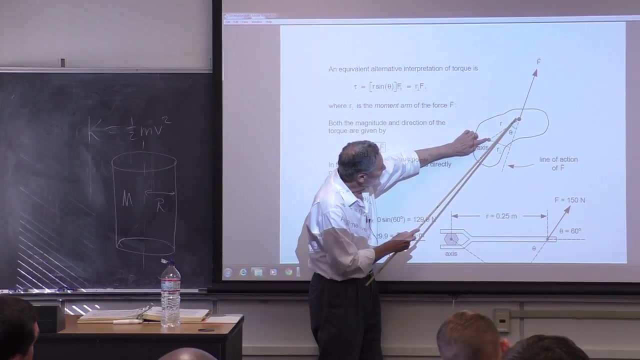 So that's our definition of the torque. There's an alternative definition that is sometimes useful. So our current definition is: you take this component of the force right and multiply by this. Here's another way of looking at it that's useful. 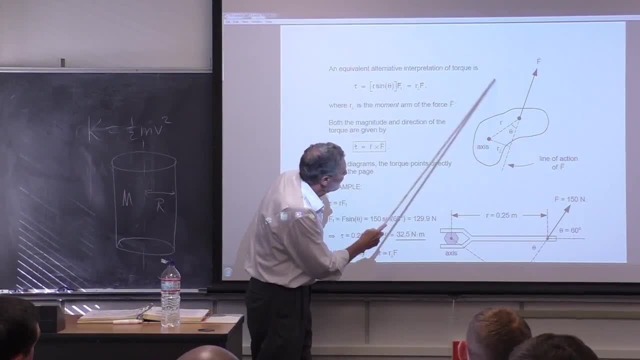 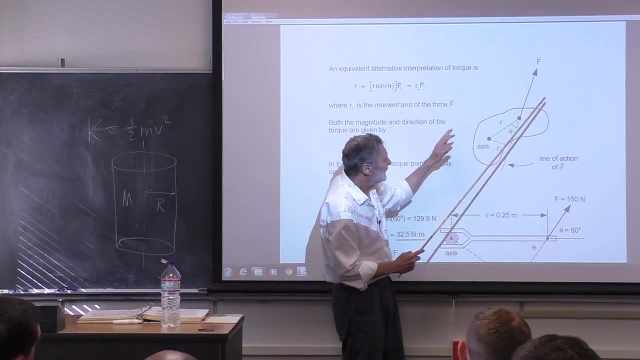 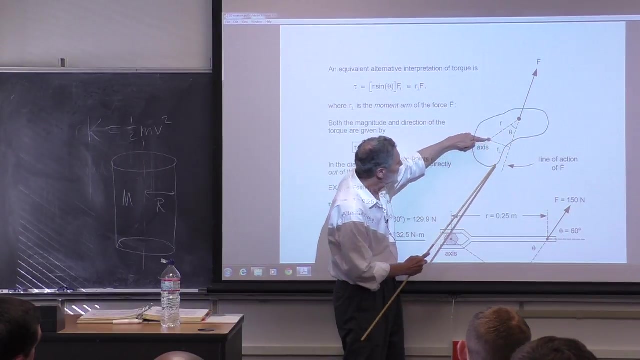 It is useful, as we will see. Forget this component, Consider your actual full force here, But the distance, the effective distance in regards to rotation, is going to be this distance right here, That's called the moment arm. This right here, This is called the moment arm of this force. L. 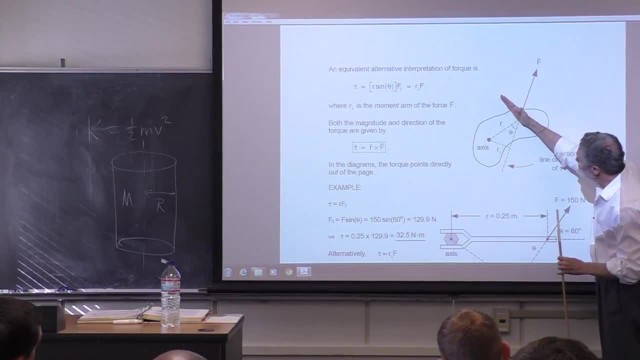 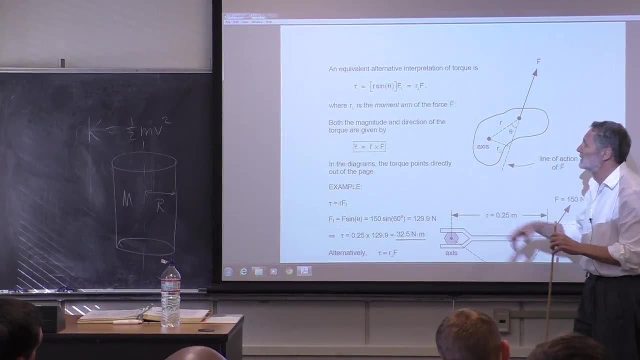 So I can look at the torque as this distance times this, the tangential component. I can also look at it as this times the relevant distance, which is this moment arm. They're identical. And then you put the sine of theta. There's a sine of theta floating around here. 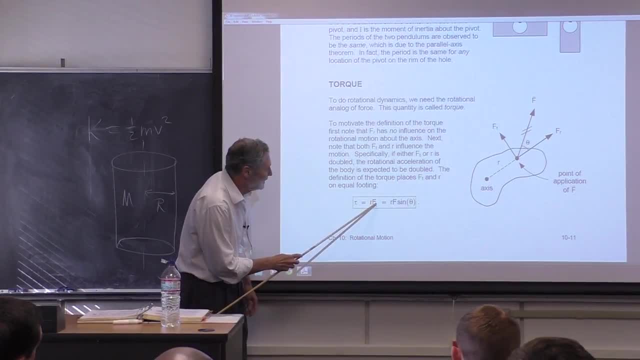 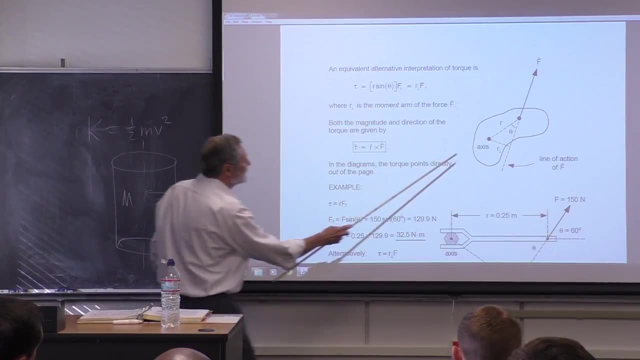 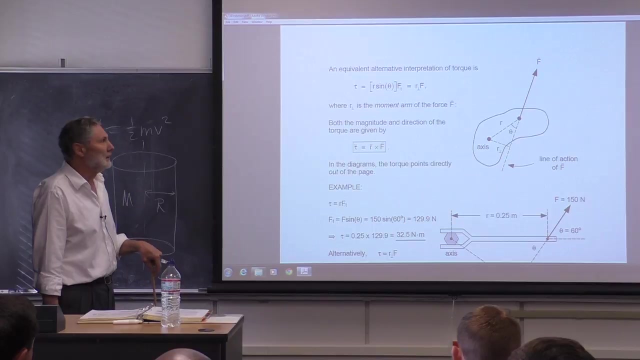 And before we associated the sine of theta with this F of t. Now we're associating with the r. This is r times the sine of theta. Now we have to talk about direction here, And the direction, the appropriate direction, is: we can use the right-hand rule. 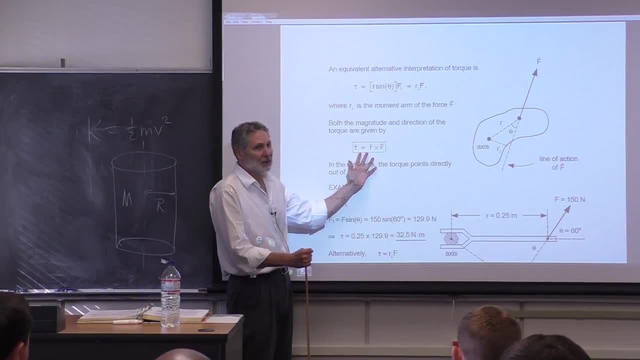 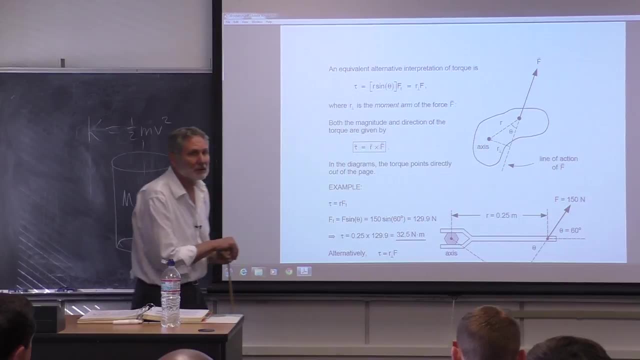 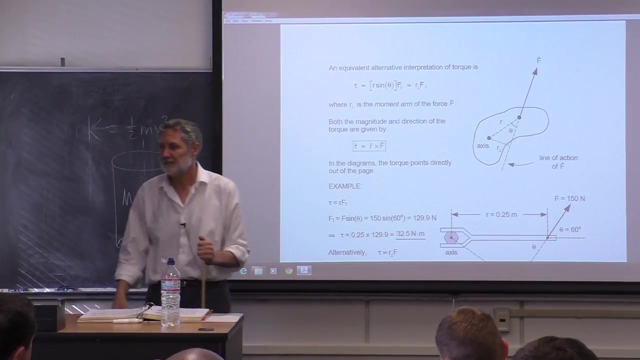 So we can actually unify the magnitude and the direction into one nice expression. here It's r cross F. So in this case, where does the torque point? This is r Straight out And it's going to cause an angular acceleration. that is straight out.